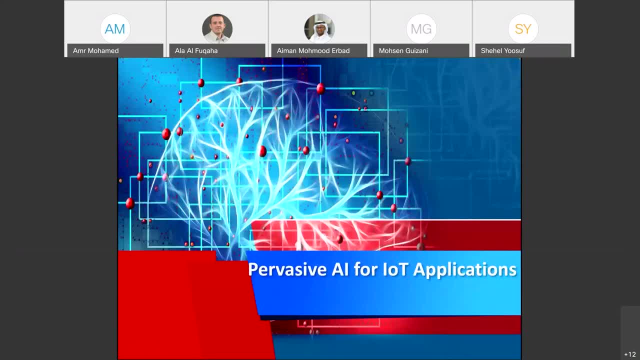 almost 10 years taking leadership role in system development for vertical industries. He's currently professor in the College of Engineering, Qatar University. He has 25 years of experience wireless networking and industrial system development. He holds three awards from IBM Canada for his achievement and four best paper awards from ITP conferences. His research interest. 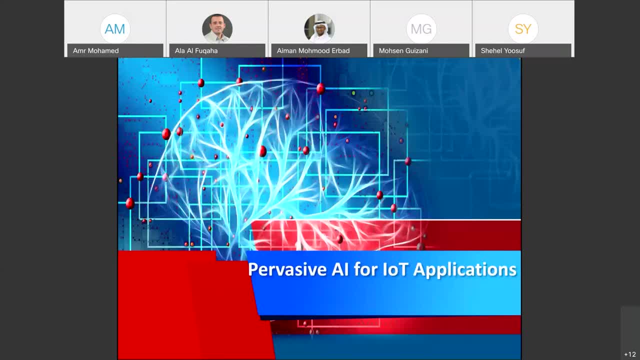 spans wireless networking, edge computing, IoT. Dr Aam authored and co-authored over 200 referred journals and conference papers, textbooks and books, chapters and reputable international journals and conferences. He served as an editor for two international journals and has served as TPC and co-chair for many IEEE workshops. Thank you, Thank you, Dr. 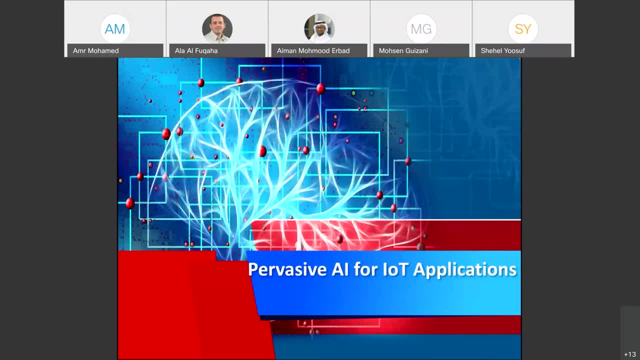 Aam, for accepting our invitation. Please go ahead. Thank you, Dr Aam. As-salamu alaykum everyone. As-salamu alaykum, Dr Aam and Biskay, and be upon you all. 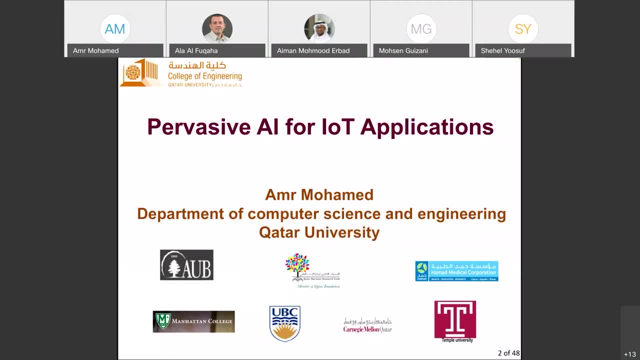 Thank you, Dr Aam. Thank you, Dr Aam and Biskay. As-salamu alaykum everyone. This work has been done in collaboration with many stakeholders in Qatar and the organizations- academic organizations like UNRF, American University in Beirut, HMC, Temple University, University of British Columbia and Manhattan College. 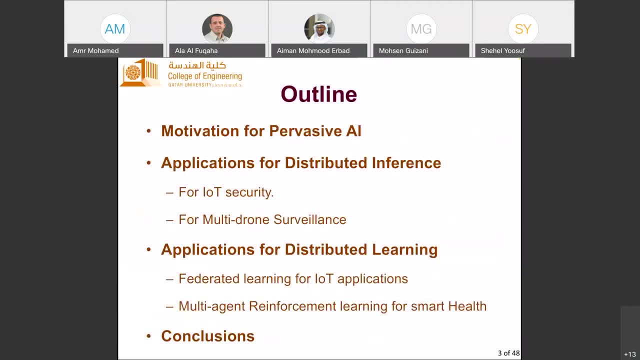 So the outline of this talk is: first I'm going to go through some motivation for pervasive AI and what it means. Then I'm going to talk about two major branches- applications for distributed inference- and I'm going to explain what that is, particularly for security and for multi-drone systems. 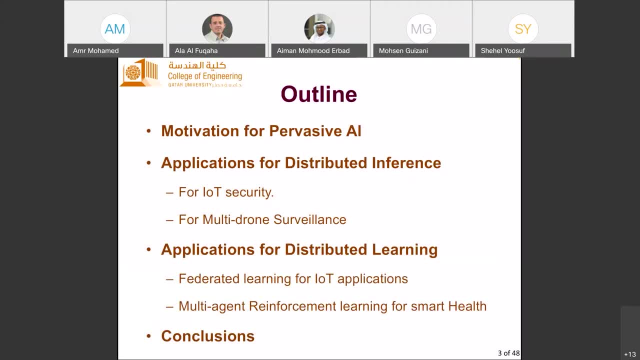 Then I'm going to talk about applications for distributed learning, including federated learning for IoT applications and multi-agent reinforcement learning for smart health, And then I'm going to conclude the talk. So, as a motivation, as we all know, IoT was first. 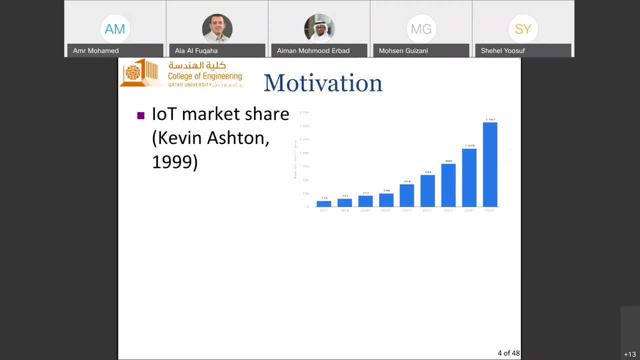 It was first coined in 1999 by Kevin Ashton from MIT, and it's evolving to dominate the market with more than $1.5 trillion by 2025.. IoT, together with AI, constitute the two most critical technologies that will shape the future of the Internet. 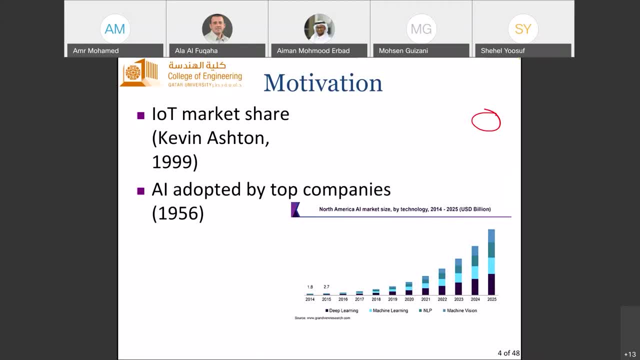 With all the technology, We have had to stop companies which are currently overtaking even the ranks from the energy companies and so on, like Apple and Google and all these companies. They are all adopting AI technologies Recently, in 2012,. we started to have the paradigm of edge and focus computing, which is also growing exponentially to address some of the scalability issues. This has become an important new language for AI. We have to adapt it to the digital age. If we can't avoid the possibilities, we have to move on to the rat race to perfect technologies for all. So we have a long way to go. So we have a long way to go. So for the next few years, we have to be prepared to face the challenges. We have to come to terms with the role that AI plays in cryptocurrency. We have to be prepared to face the challenges. 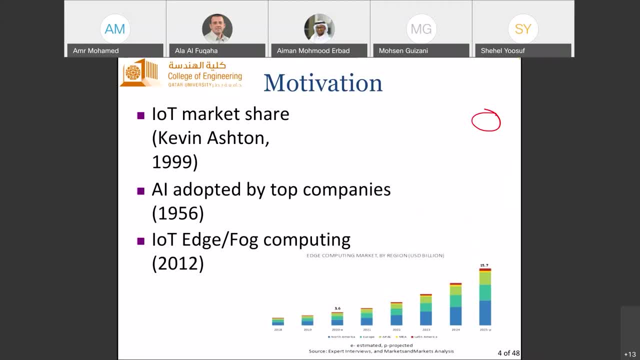 We have to be prepared to face the challenges. We have to be prepared to face the challenges paradigm of edge and fog computing, which is also growing exponentially, to address some of the scalability issues in IOT architectures, as we will see in a minute. so all these technologies, they, they are integral and critical. 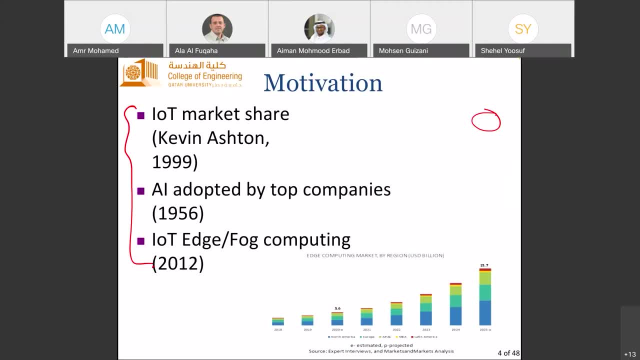 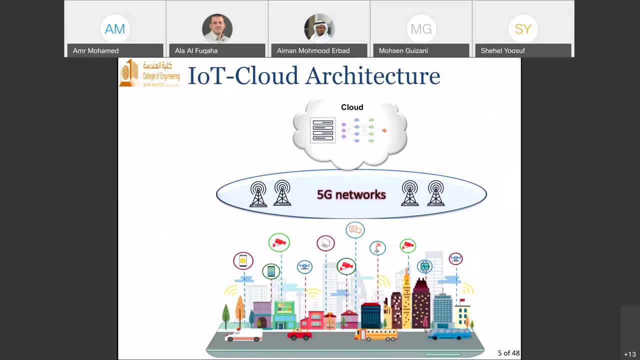 components for the industry 4.0 revolution that we see today. so traditional OII and cloud architectures. they rely on IOT devices as like mere data collectors that collect blindly the information that constitutes some characteristics from the environment and they send it directly to the cloud in a 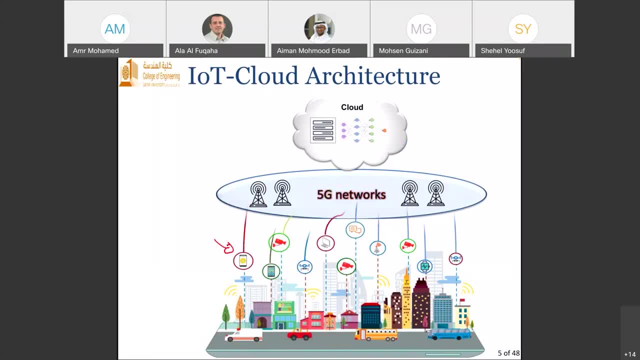 massive data streams over 5g networks. of course, this type of architecture creates or causes some scalability issues because of the fact that all these massive data streams, they, they, they actually put loads. they are not only on the cloud, but also on the on the 5g network. of course. in that case, the 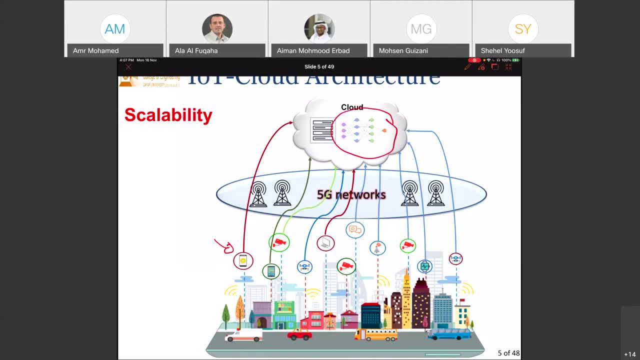 intelligence resides only in the cloud, where the AI models, they they reside and they they perform all the intelligence at the cloud level. other issues, like in the storage, where the raw data gets sent from these IOT devices and they get stored into the cloud with massive amounts and some of this data is not. 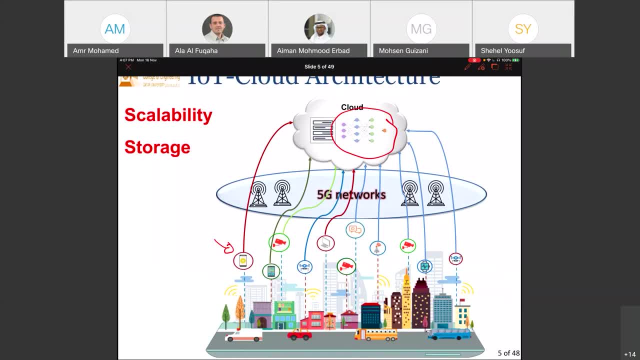 even relevant and some of it is actually not cleaned and not it's actually in some cases garbage. so this also puts some a load on the network. so from the network perspective the bandwidth provisioning for the IOT devices is a very challenging issue, also from the IOT. 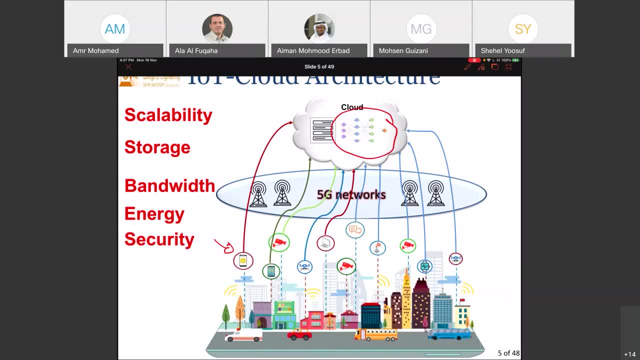 point of view. we have issues like energy consumption, where the devices are very energy hungry to try to send this raw data in massive amounts to the cloud. we also have some issues because some of this data has- it's not even you know- cleaned and and in that case you have some data. 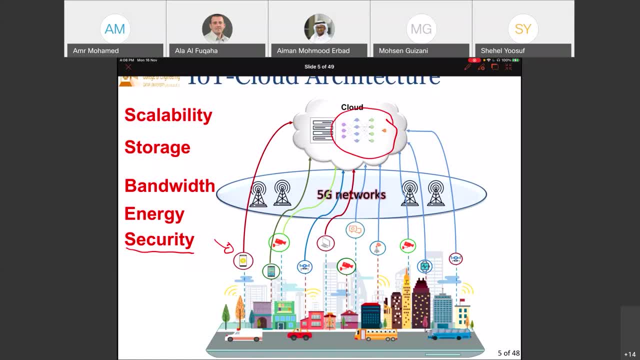 integrity issues that some of the raw data that reaches the cloud are not are not really relevant to the AI, intelligent ultrasound, the club and also some of this data is actually sent as pure information. so we have some privacy issues as well that someone could tap into this data and going over shit. 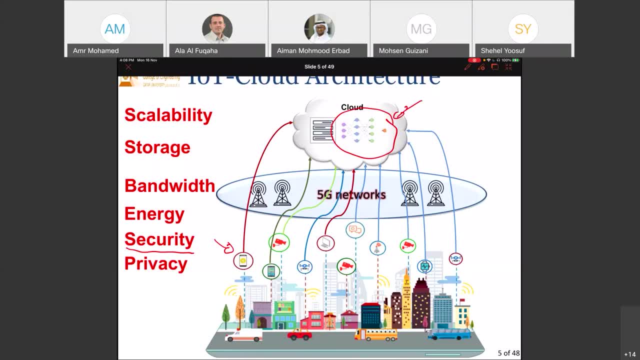 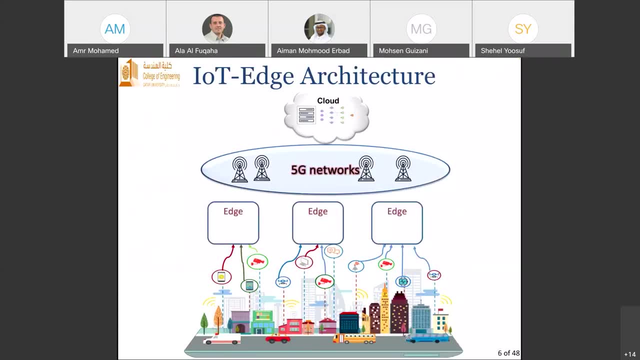 we have some privacy issues as well, that someone could tap into this data and going over shit and read some private information. so all of these issues has mandated or motivated the evolution of edge computing, as you all know, where we actually push the part of the intelligence from the cloud. 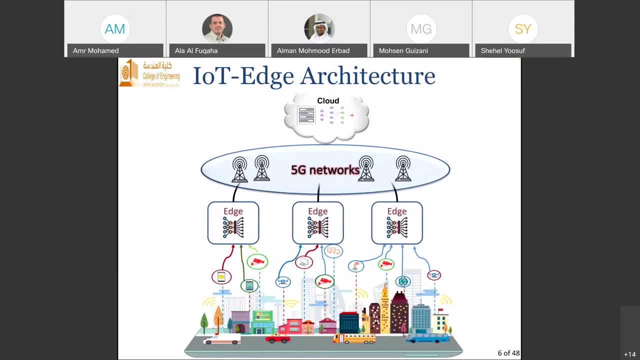 to the edge, to a designated edge node, where- these edge nodes- they collect and summarize the information from the iot devices and send that over the network in a more clean and more intelligent way, in which case this edge computing paradigm solves many of the issues that we talked. 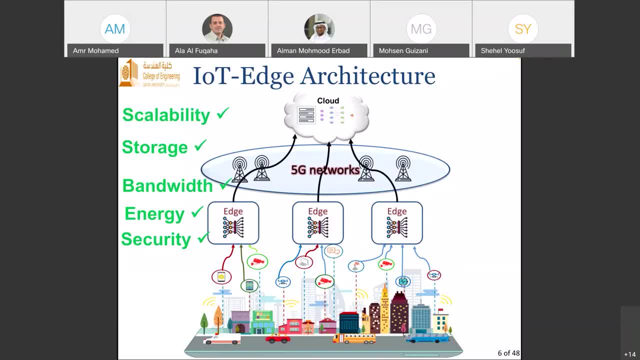 about, in terms of scalability, the storage, and they can interact with the with the 5g network more efficiently, in which case they use the bandwidth more efficiently because of the fact that you can use some energy efficient radio technology between the edge and the and the iot nodes, because of the proximity of these edge nodes to the iot devices. 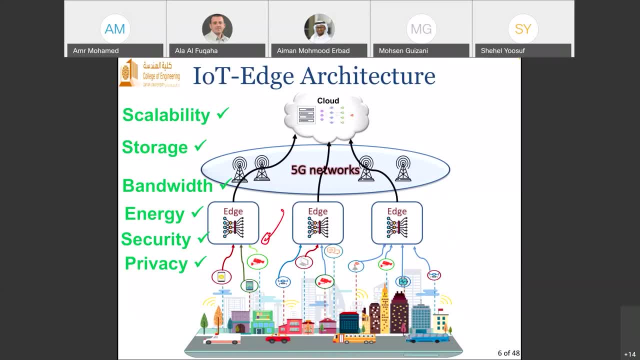 you have less energy consumption and also all the security and privacy issues can be resolved at the private network level between the edge and the iot devices. of course this creates more challenges in terms of deployment: deployment complexity because these edge nodes, they have to be deployed in strategic places. 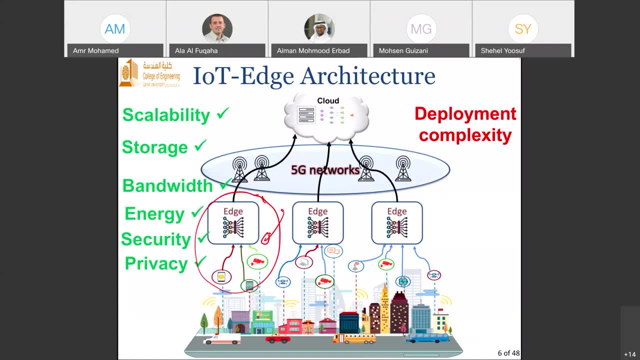 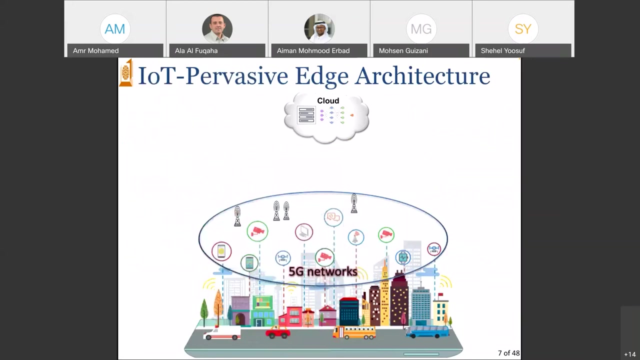 and also you have extra infrastructure by deploying these edges, and sometimes they they actually merge some of these edges with the iot devices, in which case you have some issues with the limited resources of the iot devices. so this paradigm is currently evolving to what we call pervasive edge architecture, or in other words, democratized edge computing. 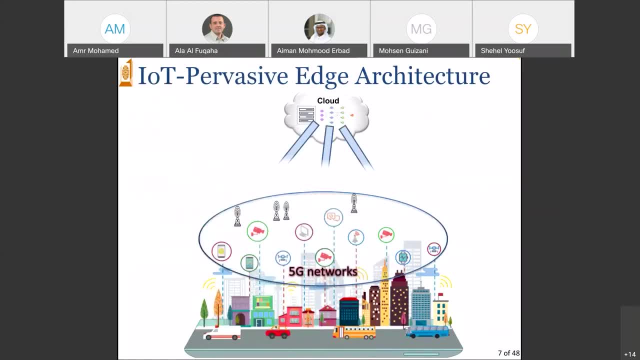 where the intelligence is actually pushed one level down to the iot devices themselves, where we actually distribute both on all the uh, the iot and the network resources in the 5g network and we do that strategically to try to address all the resource constraints that these iot devices have. so some of the issues: 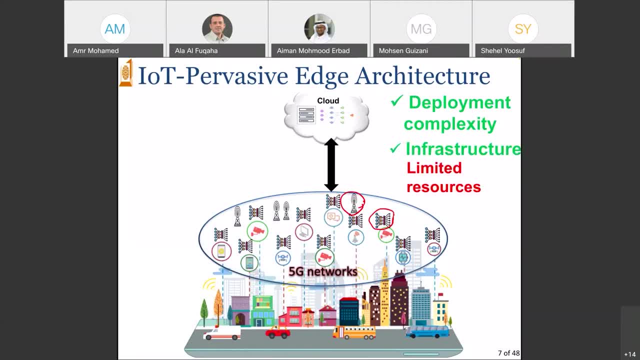 like deployment complexity is reduced, we don't have to have designated edge modes, and so on. however, we still need to address some limited resources. in fact, it's more challenging in the case of uh- pervasive edge computing- where these iot devices are more resource constrained, in which case we have to distribute both the 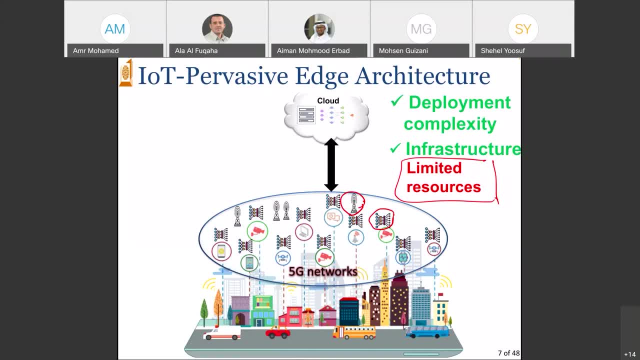 communication resources and the computation resources more strategically in that case. so this pervasive edge computing creates a new paradigm of communication versus uh computation, where we need to actually have both the access points and iot devices strategically positioned and we have to distribute the computation amongst all these network and iot devices strategically, in which case we have pervasive edge computing. 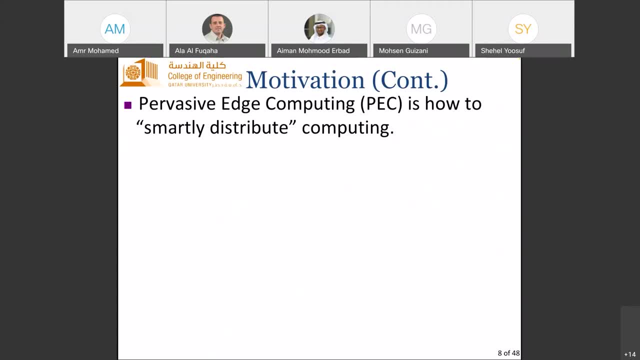 so pervasive edge computing is about smartly distributing the computation and the communication, so, uh. so when communications meet computation, the uh, the idea here is that if you compute efficiently and compute more, then you can communicate less, uh, and vice versa. so how to address the uh, the trade-off between where to where to compute in order to communicate less, in which case you can? 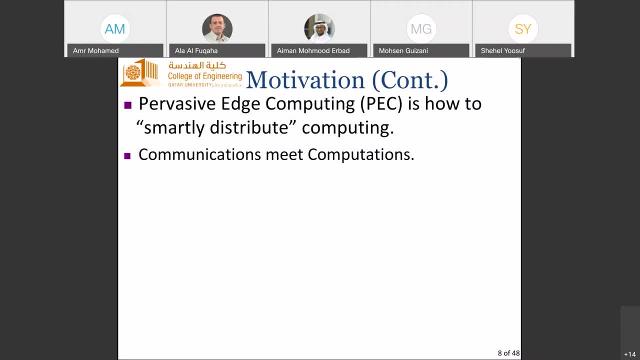 utilize the network resources and the computation resources efficiently. so when the, when we combine, uh, the pervasive edge computing with ai- and in that case we, what we try to do is to make the ai models more pervasive and more efficiently distributed amongst the iot devices of the central network, if needed we can record, for example, as i think the data base stations in 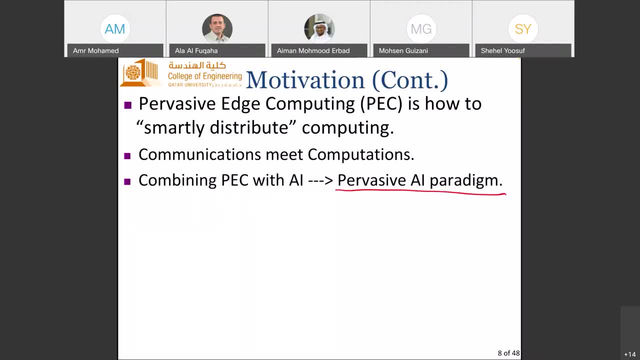 the network. if needed, then we have the product of pervasive ai systems. so as some examples of the operations that can be done on the pervasive nodes using ai, we can perform data cleaning and reprocessing. we can perform adaptive compression, where we can efficiently compress the data before transmission. hence, 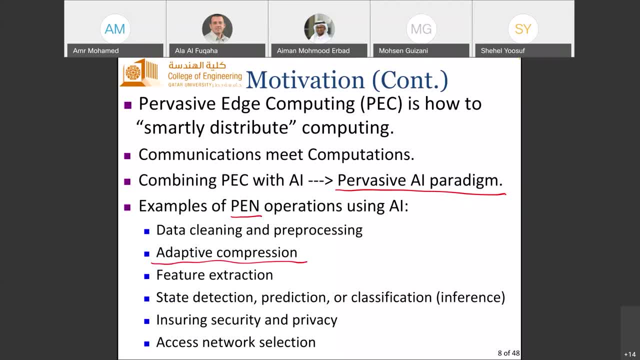 We can enhance the efficiency of delivering this information over the 5G network. We can perform some feature extractions. Instead of sending the raw data, we send features. We can detect the state of the user and we can predict the state of the user. 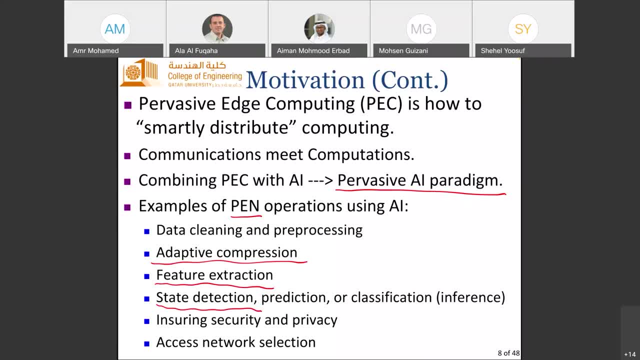 And based on that, we can do some inference or classification. We can ensure security and privacy by performing some security techniques of the data before we send it, And we can even perform some access network selection, as we will see. So some of these functions, these highlighted operations, are the ones that we will focus on throughout the remaining part of the presentation. 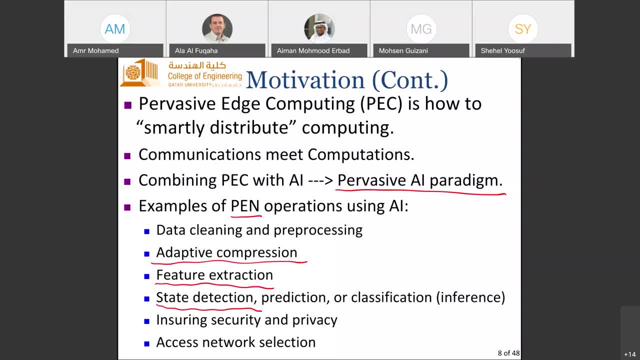 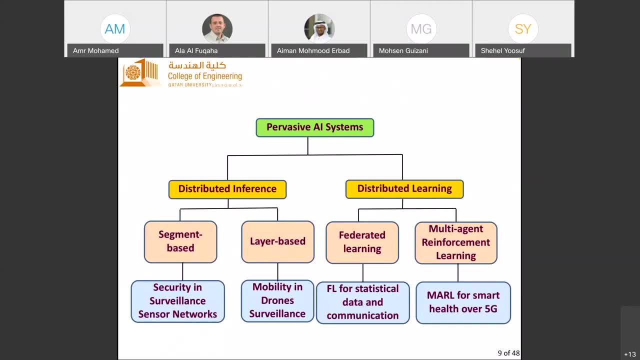 Some of them will be done using AI, as we will see. So with that motivation, we try to divide, or we try to have this taxonomy about the pervasive AI systems, where we divide the pervasive AI systems into distributed inference, And by distributed inference here I mean that we have a pre-trained machine learning model that we need to distribute amongst the IoT devices in such a way that addresses the resource constraints on these IoT devices. 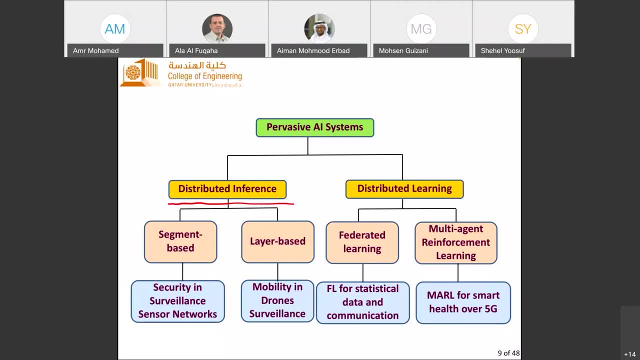 And minimize the time, The time Required for performing this inference, as we will see. So this in this branch, we will talk about distributing the machine learning model, safe based or layer based, and we will see the difference in the pros and cons for each one. 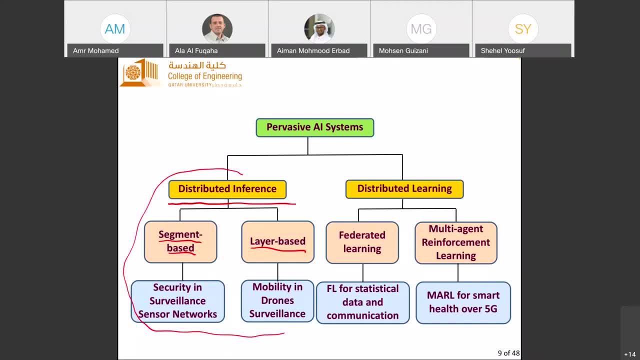 This, this branch, this area- for those of you who are trying to get into some distributed AI and machine learning areas. This area is not widely explored and I will talk about 2 use cases in this branch for IoT: security and mobility for drones. 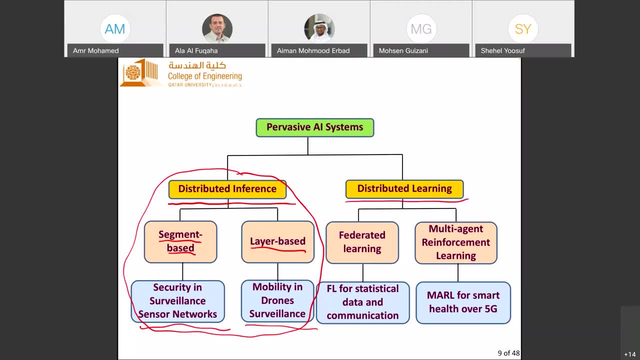 The other branch of distributed learning. in that case the machine learning model is not pre-trained. It has to perform the learning in a distributed way And this particular branch is very important. This particular branch is very important, is very, very widely explored in the literature. you have the well-established area of federated 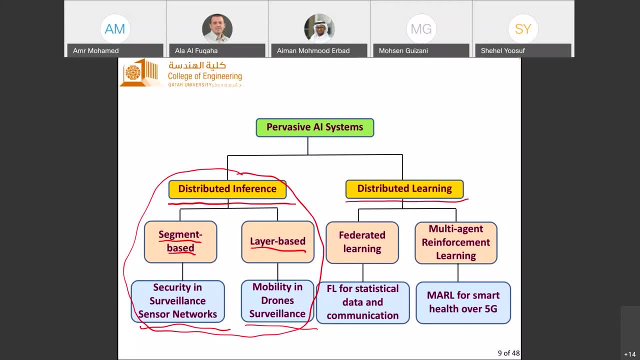 learning, where you exchange the machine learning model weights between the iot nodes, and you have the other well-established area as well, where we use multi-agent reinforcement learning to perform some distributed optimization using some distributed agents, as we will see. so i will talk about a specific use case for each of these sub-branches as we go, as we move forward. 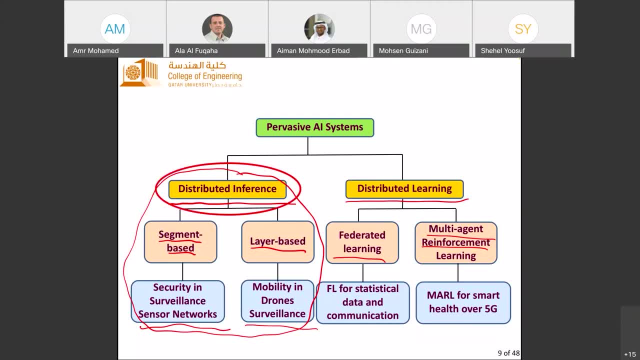 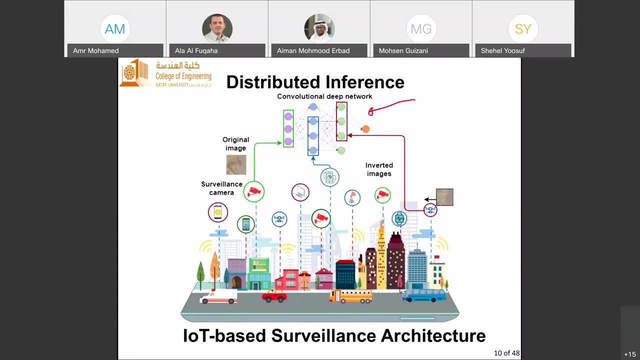 so first i'm going to cover the distributed inference where again we have some pre-trained model that we need to distribute amongst all the iot devices and in that case we have an intensive machine learning model like vgg16 or vgg19 or some of these intensive machine learning models. 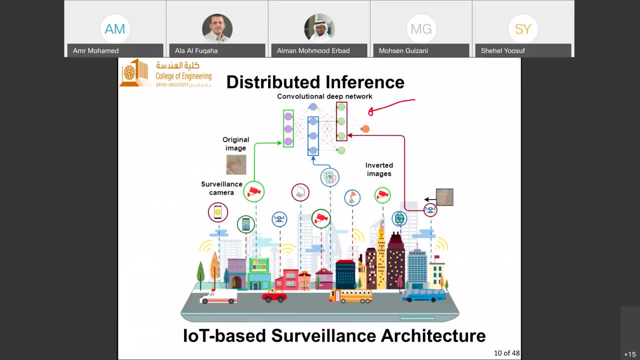 and the idea here is to try to divide this machine learning model strategically amongst all the iot devices in order to address a certain performance metric. so objectives here are to optimally distribute the machine learning model amongst the iot devices and to address the resource constraint of these iot devices in order to minimize 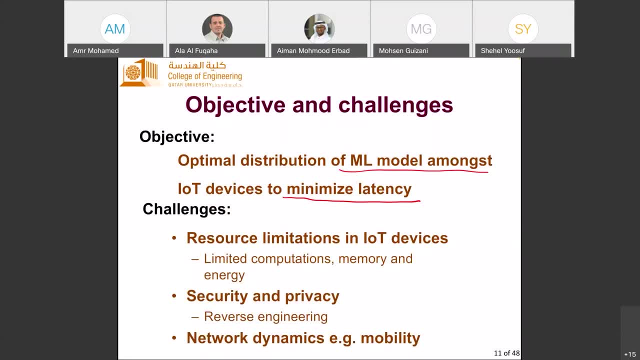 the latency and parallelize the computation amongst multiple requests, as we will see in a minute- and the challenges here are, of course, the resource limitations on these iot devices in terms of computation, memory and energy and so on, and also how to distribute this machine learning model in such a way that preserves the security and privacy and prevent any kind of black box. 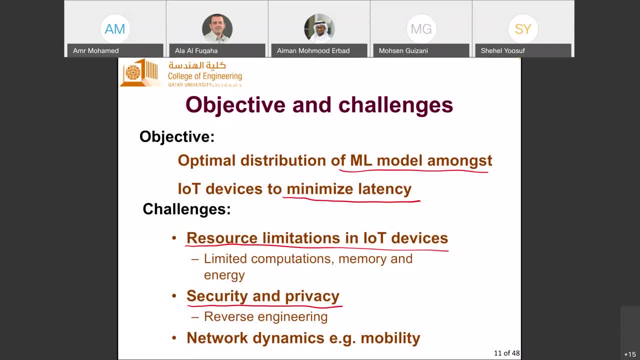 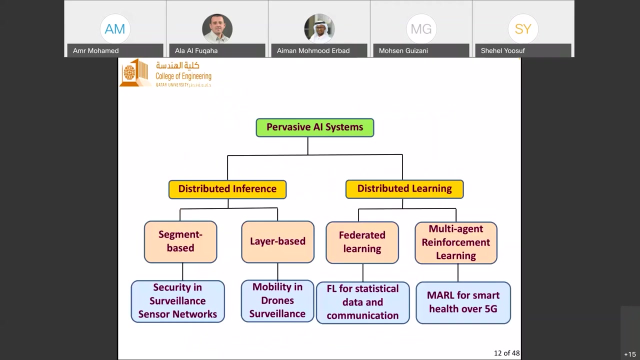 attack and any kind of reverse engineering to the actual data, as we will see. and on the other side, we address the network dynamics, such as mobility for the case of mobile iot devices like drones, as we will see. so, to talk about the first use case, where we need to strategically distribute the, the machine learning model, 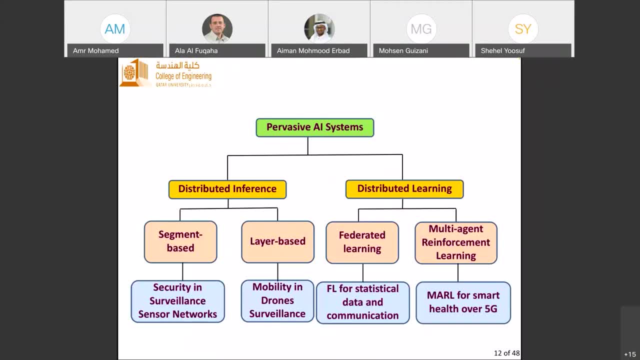 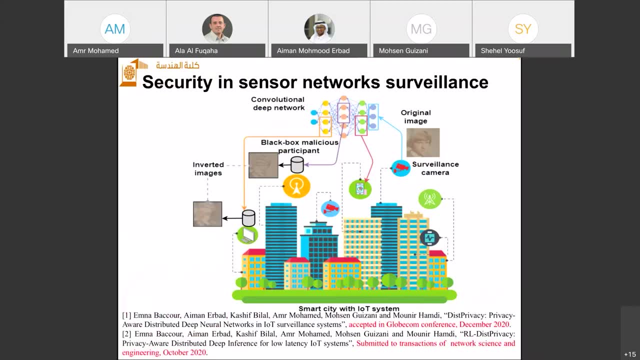 on the iot devices to address some security for uh for iot network. we have uh, we have the uh the this smart city iot system where uh you capture an image from uh an original uh an uh source surveillance camera and you need to uh identify the person in that in that image, uh through uh intense. 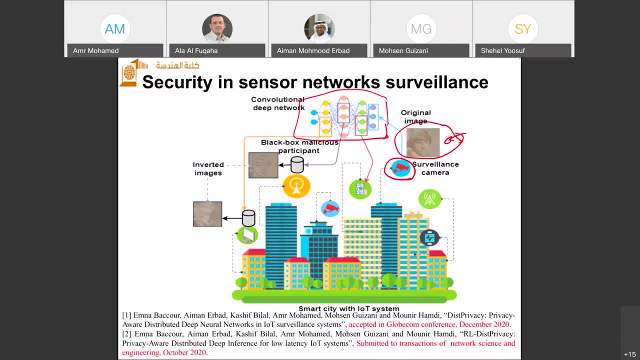 machine learning, uh operation, uh using, like, for example, uh vgg19 or some of these well-established uh machine learning architectures. so the idea here is that how to divide, how to divide uh the machine learning model into segments and uh strategically position these segments to the different iot devices in such a way that will minimize the latency. 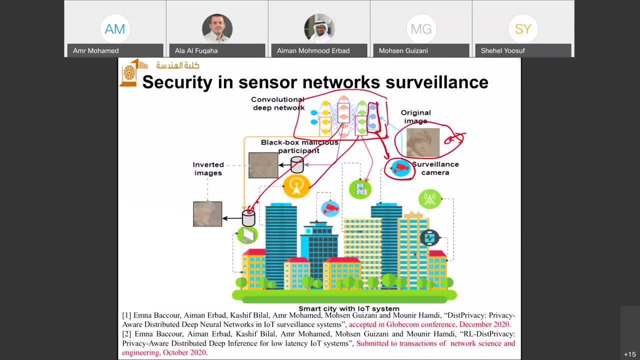 or the end-to-end time required to identify uh, the, uh, the, the, the person in the image and, at the same time, prevent or avoid any kind of reverse engineering from uh, an illegitimate uh, node, uh that tries to reverse engineer that image, so, uh, so by by segments here, by the way, we mean that uh, we. 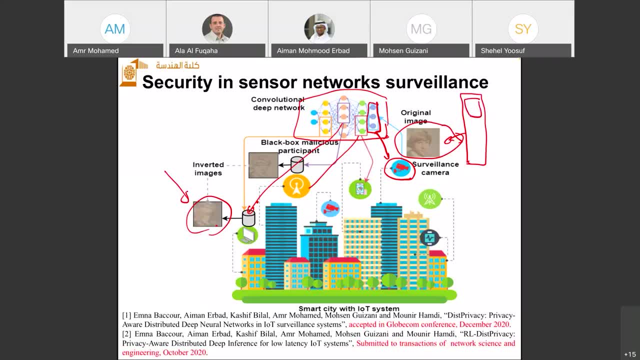 provide the actual layer into uh smaller segments, and each segment here includes a set of uh feature maps, or in other words some kernel filter in the using the terminology of convolutional neuron network, such that each segment can perform the operation uh separately. and we'll see how to do. 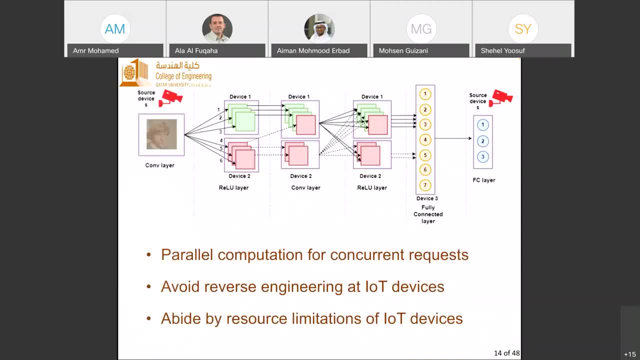 that. so the idea here is that, from the source node which captures, uh, the image, we need to divide the machine learning model into feature maps and we divide each layer into smaller segments in such a way that we have set of requests coming from different sources and we need to for. 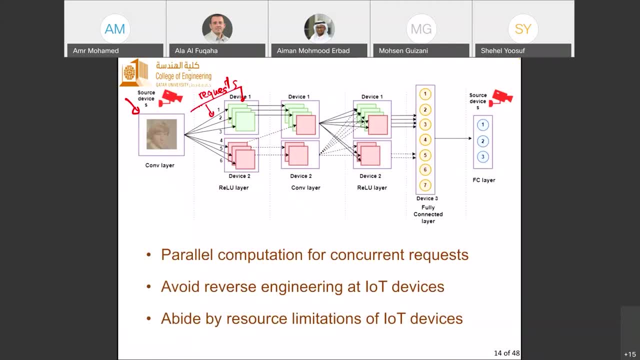 each request we need to perform the end-to-end uh inference operation, uh by dividing the machine learning model into segments at each iot device, so uh. so, for example, we divide the, the cnn model, into the, the vgg16 or vgg19 into uh, like the relo. 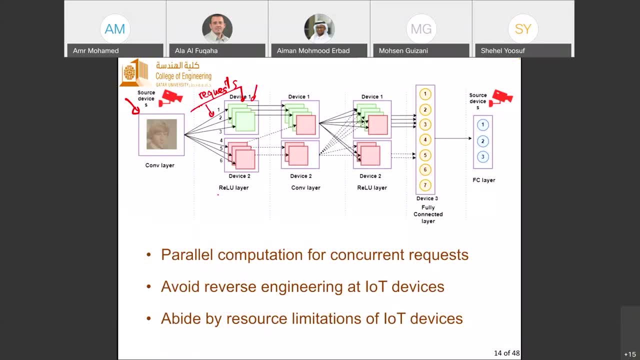 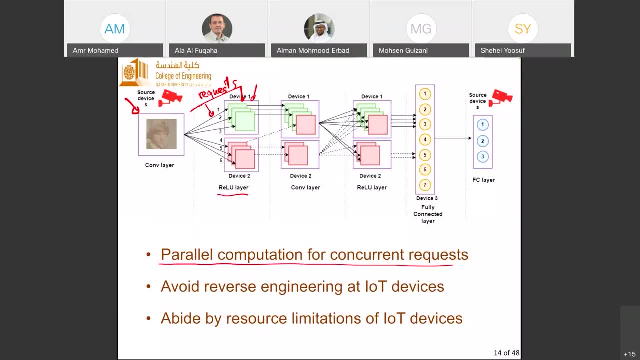 address the, the parallel computation for concurrent requests. so we have multiple requests coming from multiple uh source nodes. we need to do it in such a way that avoids that any uh tampering that happens at each or any of these levels, that if you try to reverse engineer the uh, the actual data 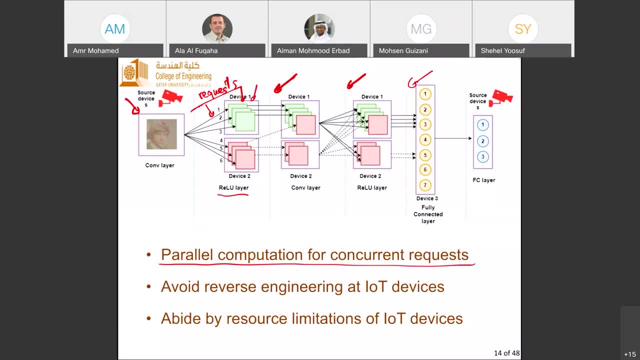 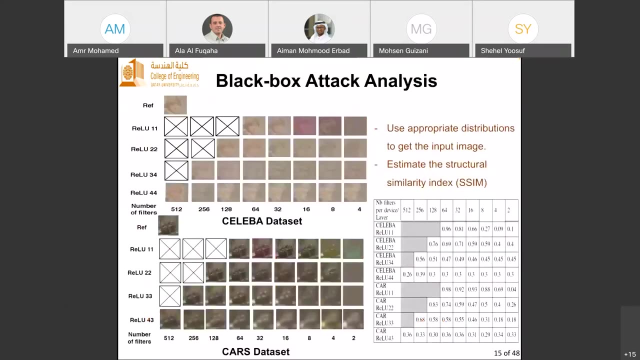 uh, from, uh, from, from any stage, that this needs to be uh avoided, this needs to be uh avoided, and we also need to need to abide by the resource limitation of these iot devices. okay, so, uh, so to do that, the first thing we have done is that we have conducted some 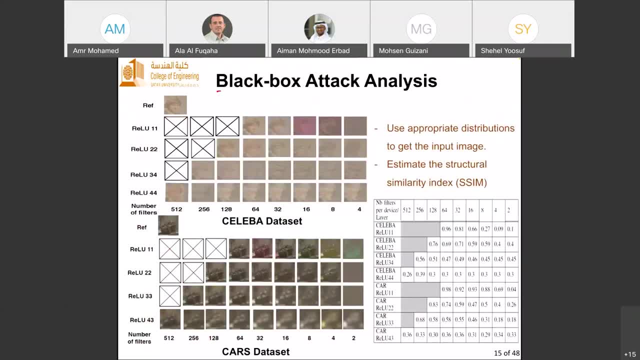 black box attack analysis uh, where we try to use uh a model, uh to to try to reverse engineer the uh, the actual image at different levels of the cnn model. okay, and the main conclusions uh that we uh have reached here is that if, if you, if you notice as you go deeper- and this actually makes uh uh perfect sense as you go deeper, 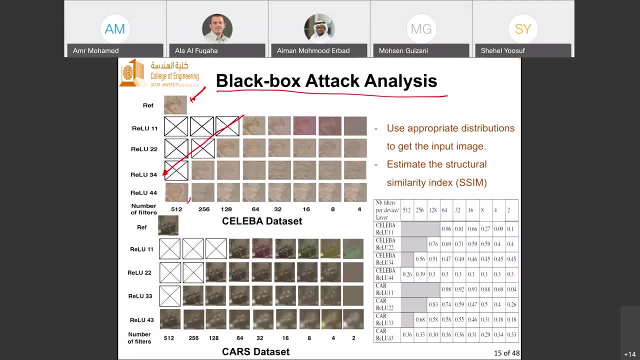 in the uh, in the layers uh, you will not be able to extract clear uh uh data or the reverse engineering would be uh hard. also when you divide each layer in segments, okay, so the less uh number of feature maps you have access to, again the uh, the harder the reverse engineering would be, and we have conducted this. 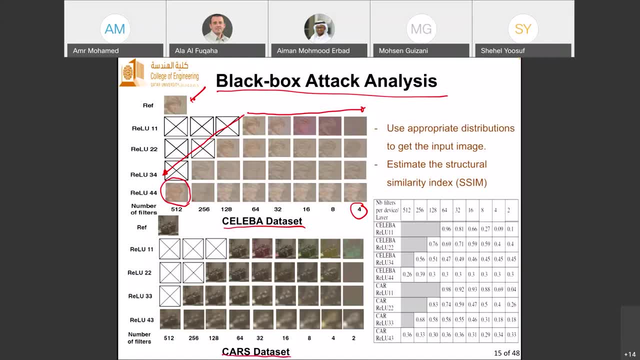 on two very uh, well established data sets. and and then we have constructed this lockup table using a metric called the structural series. similar model, the easel matrix, call the structural semitary similarity index measure, where we try to reverse engineer the uh, the actual input, store input. 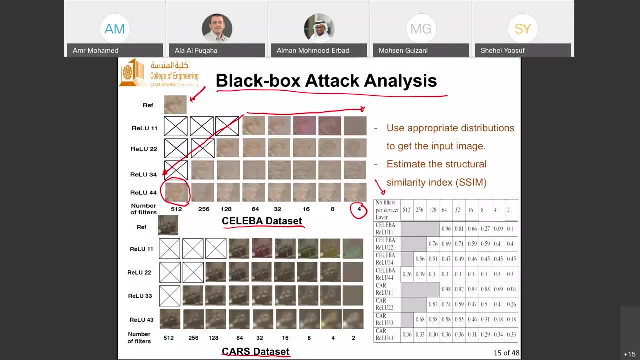 image from different levels and from different feature maps, and then we uh we try to estimate the similarity index. so, using this table, uh, we can uh then try to uh say if, if we need to to have a similarity of like, for example, up to 0.3, so we need to keep the similarity uh at maximum. 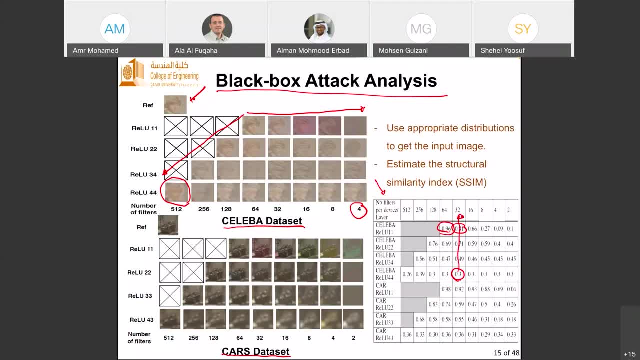 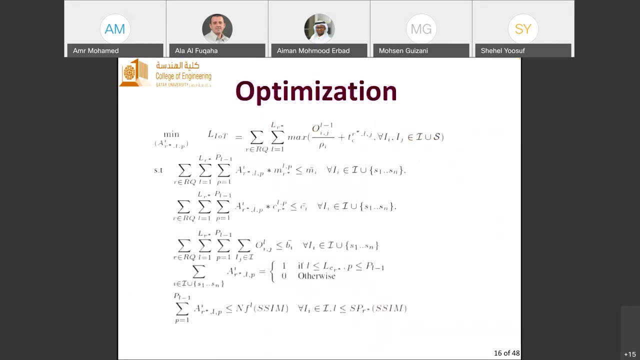 0.3. so in that case we need to have access to only 32 feature maps per per layer, and that will allow us to uh, to kind of identify the split point where we need to divide the different layers into segments. okay, so by doing this, we, uh, we, we try to construct this optimization problem, where we try 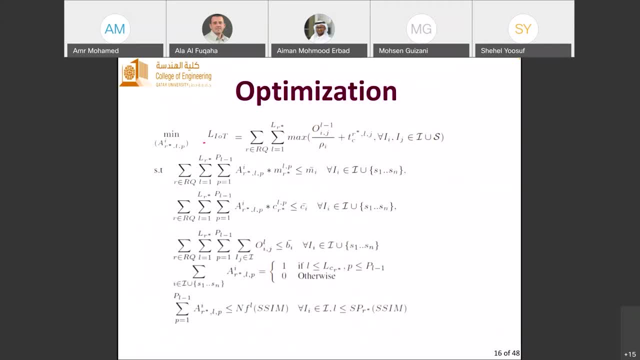 to minimize the latency of performing the entrance uh operation, uh end to end, from the source all the way to uh constructing the uh or performing the classification. and we try to minimize this latency which is a function of some uh uh network parameters like, for example, the, the length of the segment. 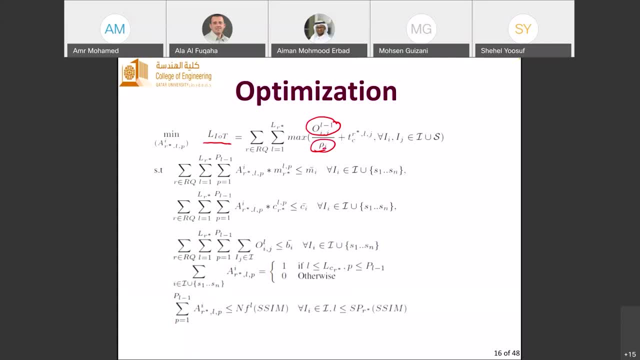 the actual data rate that this node has, the computation latency and so on. and, of course, this maximum is because we need to. each segment would have access to multiple devices, so we need to synchronize the data here, so we need to calculate the maximum, the maximum latency across the different uh devices, for that belong to. 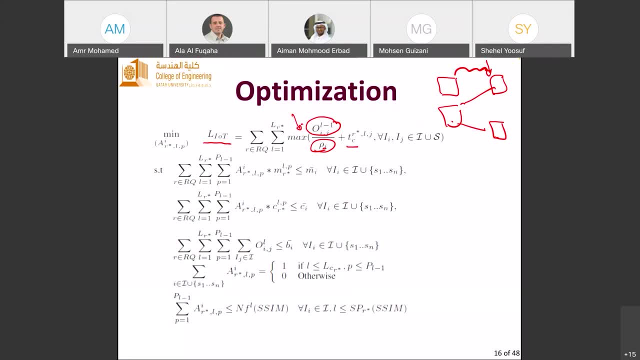 one specific layer. so with that, we need to minimize this latency end to end, subject to some constraints. the first constraint would be on the on the actual memory size of the iot device, so all the segments that are assigned to this iot device are are able to be stored inside this IoT device. 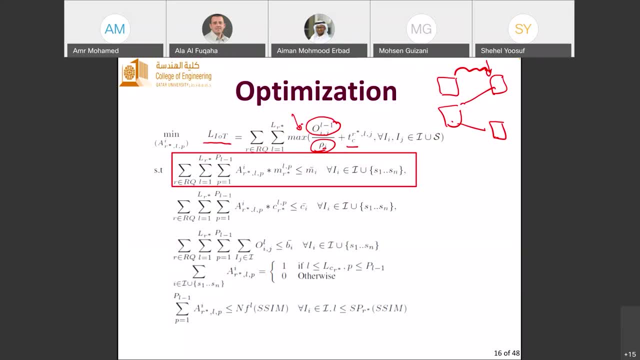 We have also some computational limitations on the IoT device, So this constraint meets the tries to guarantee that the computations required by each IoT device can be in fact performed, given the capabilities of this IoT device, And we also need to address the network bandwidth constraints that this device can have. 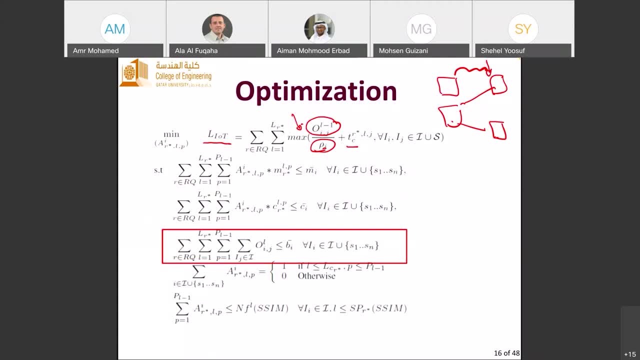 based on the radio technology that this device has access to, whether it's like Wi-Fi or 5G and so on. And, last but not least, we need to also meet the security requirements through the black box attack using the similarity index measure that we have conducted in the previous slide. 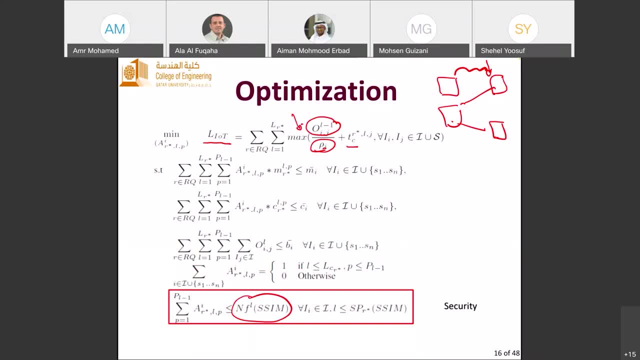 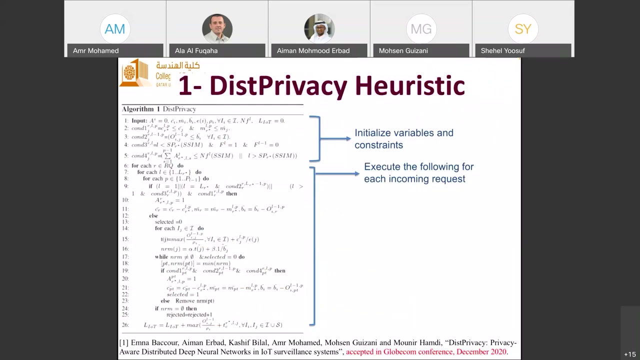 So of course this optimization problem is nonlinear in nature and also it has combinatorial complexity. So the proposed technique here is to try to devise a heuristic technique which can work in real time based on receiving a single request. So the algorithm is too long. 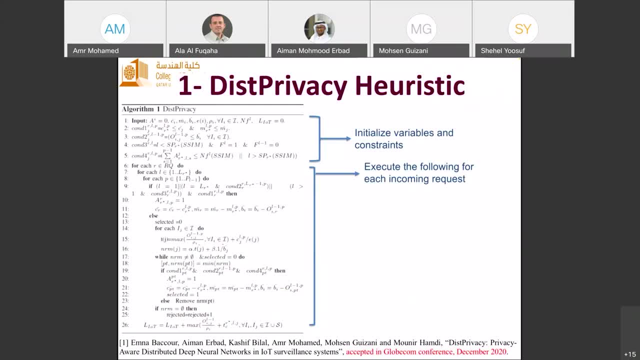 but, in brief, the way that this algorithm works is that first, after initialization, I receive each request and I perform this logic for each request And this logic, basically, is divided into two or three different parts. The first part is basically to for each request. 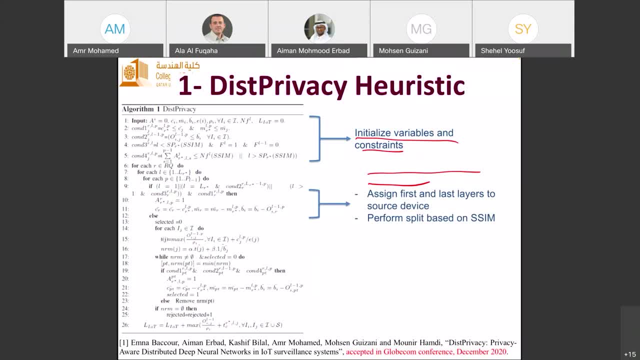 we assign the first and last layer- fully connected layer- to the source device and then perform the split point based on meeting the security or the similarity index measure, And then we try to assign the different segments that are split using the SSIM to some IoT device helpers. 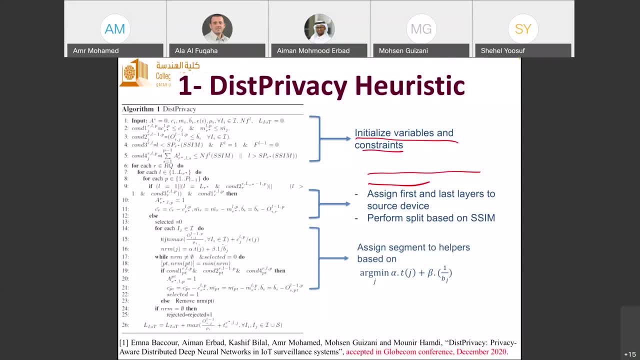 based on addressing the trade off between the latency and minimizing the bandwidth rate, The bandwidth requirement or the- sorry- the rate requirements on this IoT device, And we try to do that across the different split points, And if we can't, then we have to reject the request. 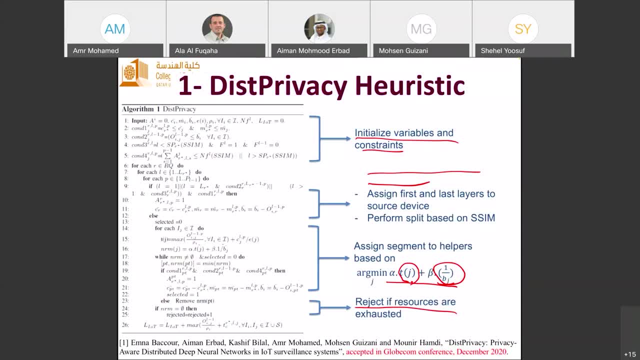 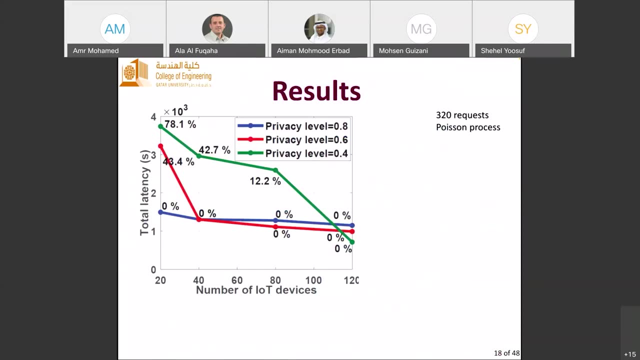 based on the fact that the resources on all the IoT devices are exhausted and we cannot accommodate any more requests. So the heuristic algorithm has been tested. So the heuristic algorithm has been tested. So the heuristic algorithm has been tested across different number of IoT devices And, as we can see that, as the number of IoT devices is low, 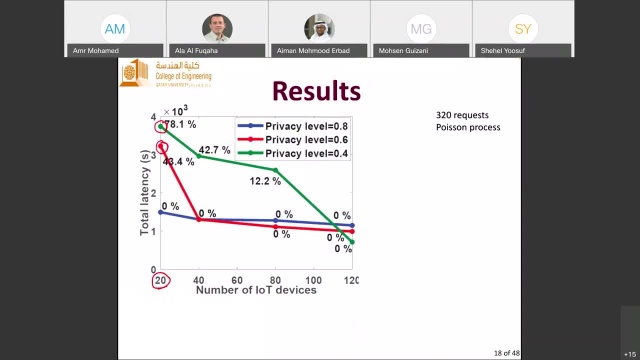 we tend to reject more requests. So we have to reject multiple requests- more than 70 or 80% of the incoming requests- because of the fact that the number of IoT devices available are small, So we don't have enough degrees of freedom to accommodate the 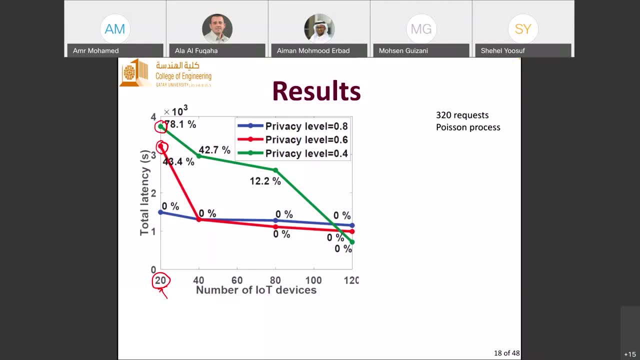 the different requests And, of course, as the privacy level gets more stringent. so for privacy level- point four- we have to of course divide each layer into more and more segments, which requires more devices to be engaged in the entrance operation. 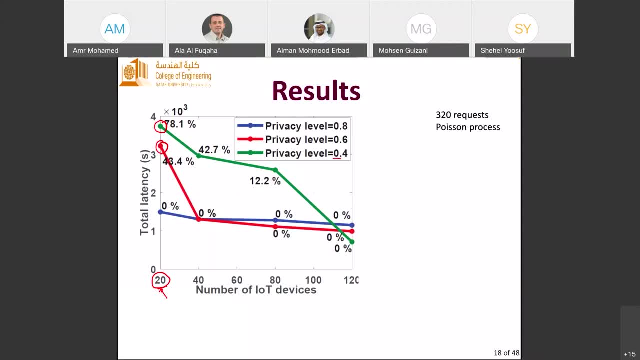 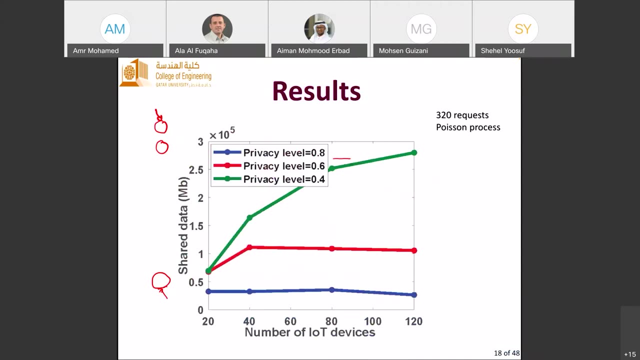 in which case the constraints become more stringent And we have to, of course, reject more requests, as we can see on this green curve. So this is despite the fact that, for privacy, level point four, or for more stringent constraints, we see that the amount of shared data between the IoT devices. 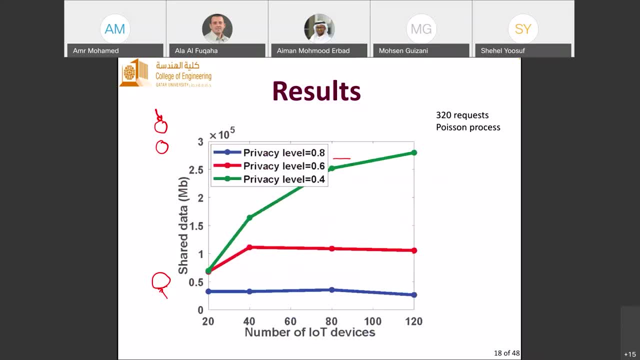 is in fact more, is in fact, higher compared to the other IoT devices. However, this shared data is allowed to be more parallelized And and in that case, more and more devices they get engaged into the, the inference operation. 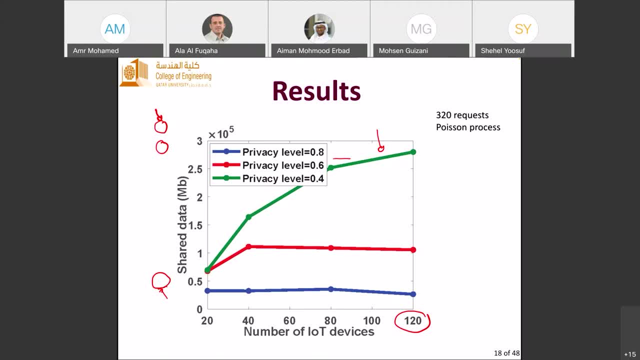 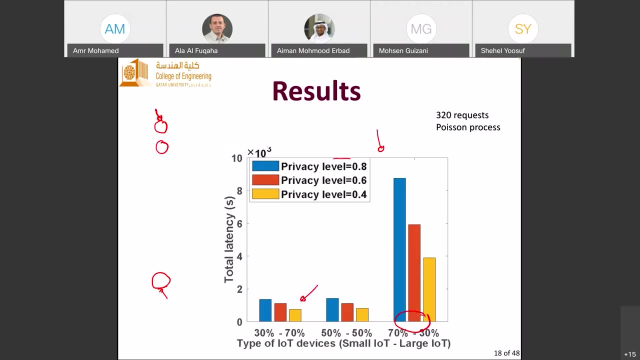 making the parallel computation of multiple concurrent requests possible in that in that case. So that's why the latency, for that's why we see that the latency- surprisingly or interestingly speaking, the latency for the privacy level- point four is- is actually less in that case. 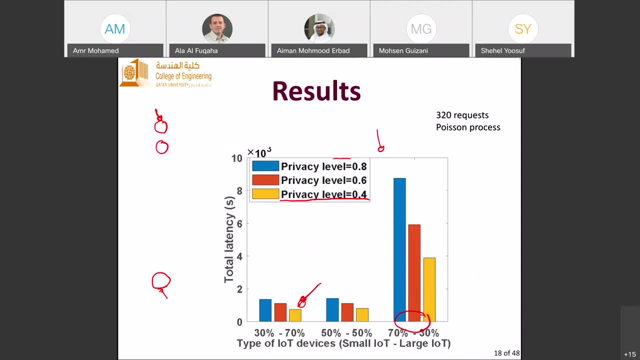 because of the fact that we, by dividing the layers into smaller segments, we need to engage more and more IoT devices, in which case they use different links And in that case, the latency would be less. Also, we have tested this under different kind of. 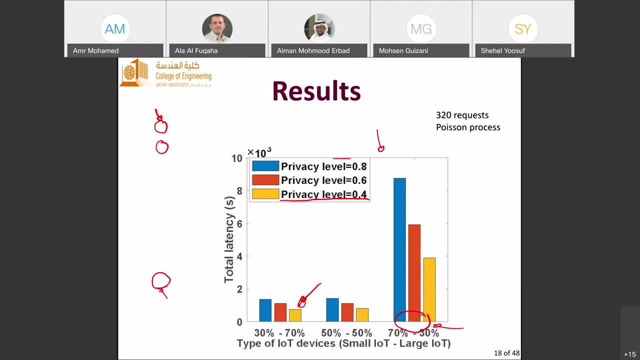 different IoT networks, different IoT networks, different network configurations. where we have in- in some configuration we have 70%- small IoT devices. By small IoT devices we mean like a Raspberry Pi, small Raspberry Pi with, of course, less resources. 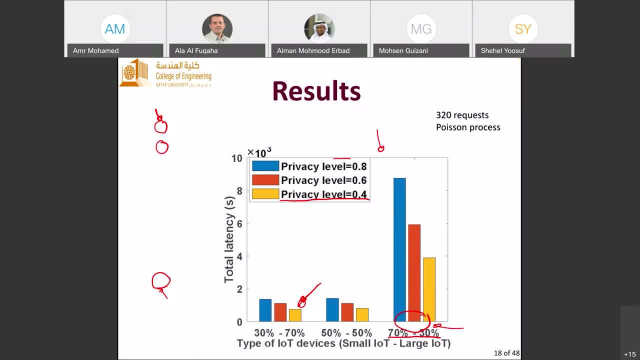 And 30% of the IoT devices would be like a Nexus mobile device, which has more capabilities in terms of computation and memory, And in that case, of course, when the small IoT devices are the majority of the IoT, the latency tends to be more. 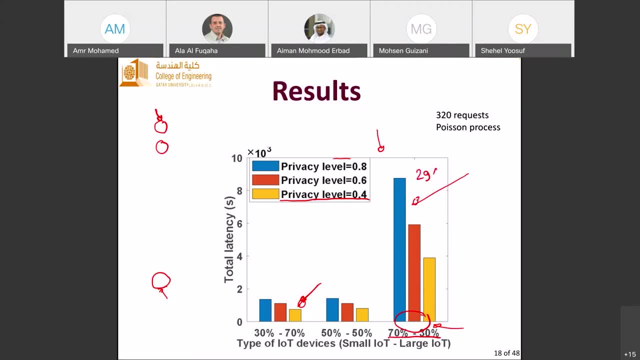 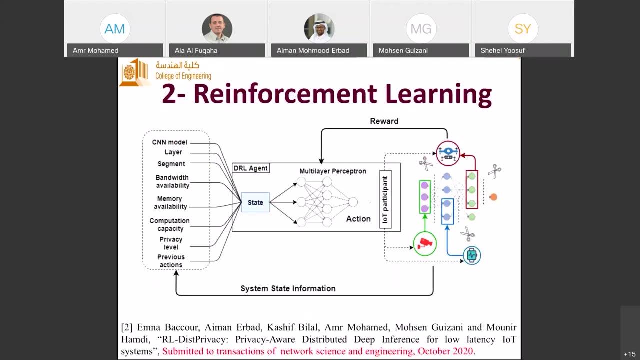 And not only that, we tend to have more rejections. So there is about 29% rejection of requests for the case of the majority of small IoT devices. Okay, So, so another approach, which is completely different, to solve the same optimization. 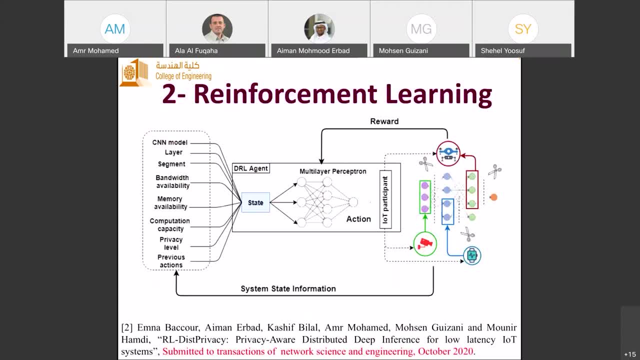 problem is using reinforcement learning, And I assume that you all have some idea about reinforcement learning as a tool, as an efficient tool to solve optimization problems, And in that case we resort to using a single agent- reinforcement learning- that tries to learn the evolution of 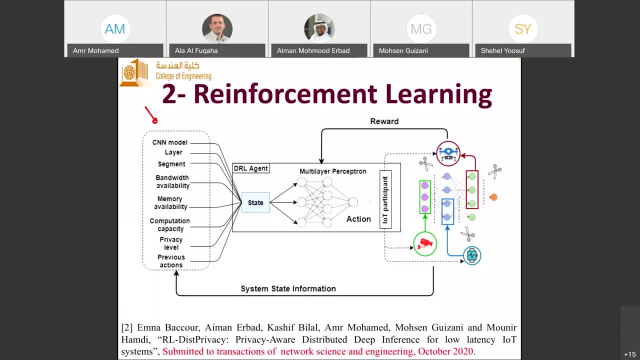 of the state transition in the system and tries to learn that- the transition of states- and then convert that to set of actions which constitute a policy over time. that tries to maximize a certain word through some suboptimal solutions or suboptimal actions. 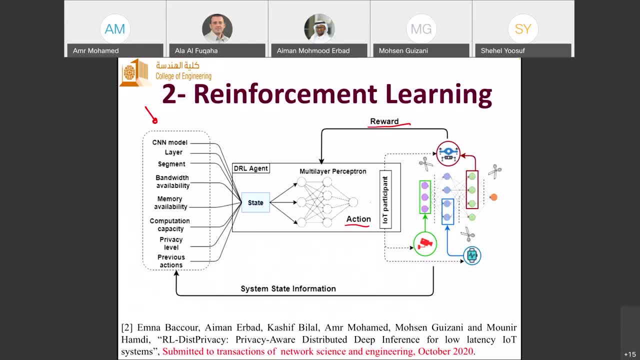 So the, of course, the reinforcement learning algorithm in that case, will try to learn the best set of distribution of these segments for the machine learning model across the IoT devices in such a way that meets the resource constraints and minimize the latency of the inference operation. 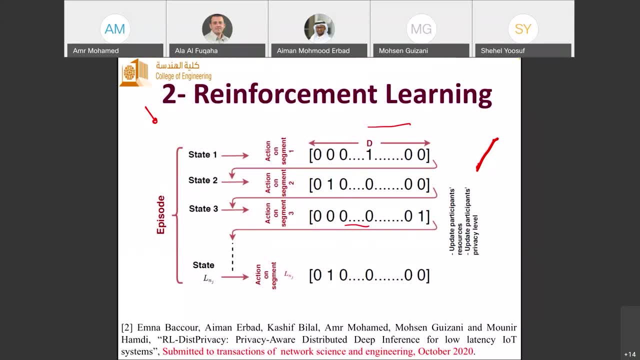 So the? so, instead of trying to devise a two dimensional matrix of actions that would try to learn the location of each segment in the IoT devices, we have done this in a chain operation like this, So we based on one state of the system. 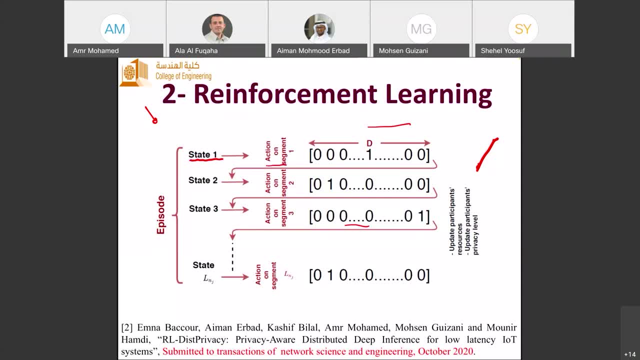 we try to allocate segment by segment, So the action of the agent at a certain point of time would be just a vector that would represent where this segment should be located in which IoT device at any point of time. And we do that iteratively until we allocate all the 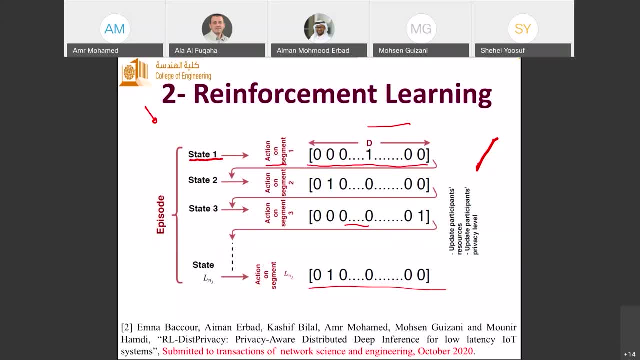 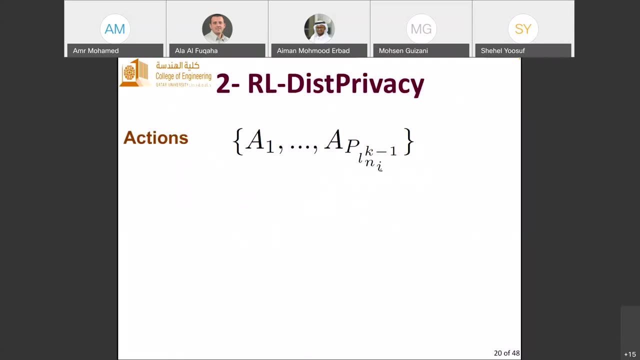 all the segments in the machine learning model, strategically across all the IoT devices. So, in which case, the actions for this agent is gonna be- actions of this agent is gonna be like a vector of binary, like a vector of binary, binary variables, which 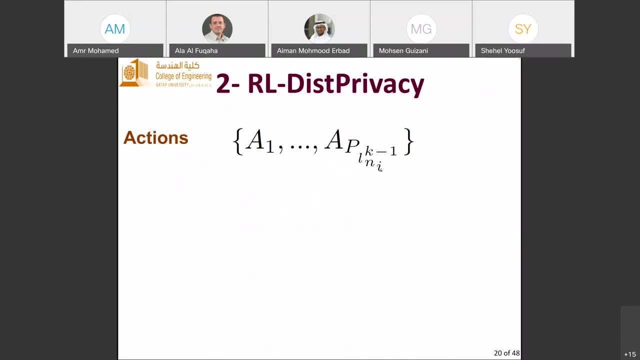 which represent where a segment is allocated on which IoT device in the network And, based on this action, we we get to a network state which which takes a specific CNN machine learning model, whether it's one of the models that we talked about. 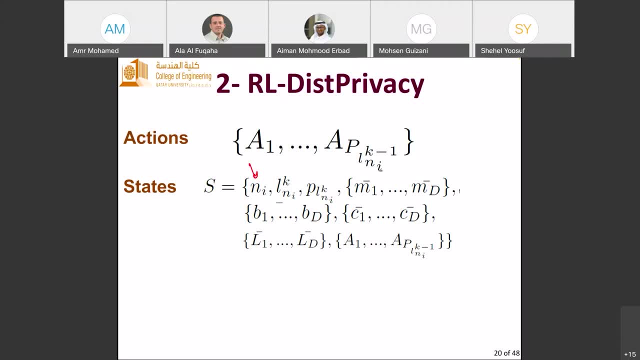 whether it's a VGG16 model or a, a VGG19 model or any other CNN model, And it puts the: and what is the current layer? what is the feature map? What are the memory constraints on all the IoT devices? 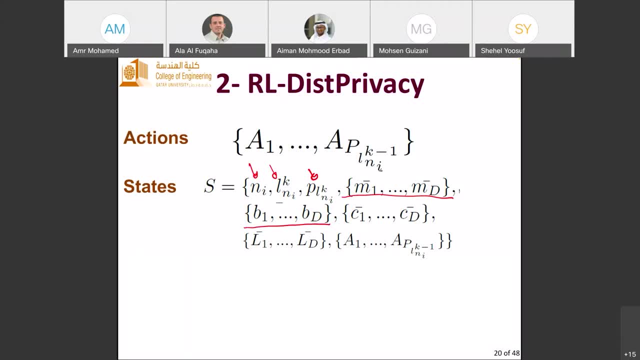 What are the data rates, What are the computational capabilities and so on on each IoT IoT device And based on that, we calculate a reward, based on the conditions or the constraints of the optimization problem and try to estimate the reward which is based on this formula. here, And for this case, this part tries to engage. 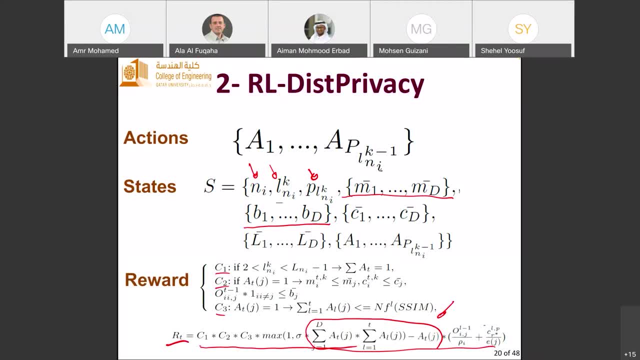 the minimum number of IoT contributors to the inference operation. And this penalty here constitutes the cost that I have to pay in order to position a specific segment in one of the IoT devices, based on calculating the data shared and the computation required by this IoT device. So we try to perform certain random actions and then, based on these random actions, 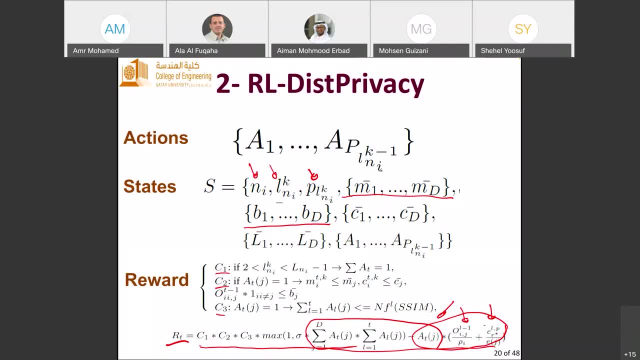 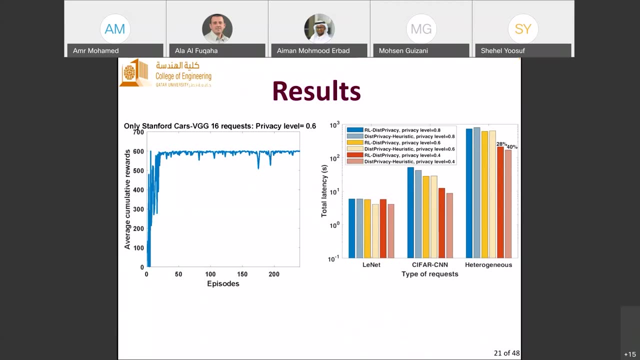 we calculate The states of the system and the reward that corresponds to this, And we keep doing that across the different episodes until we find, or until we reach to, an optimal policy that will try to minimize the latency subject to the resource constraint on the IoT devices. 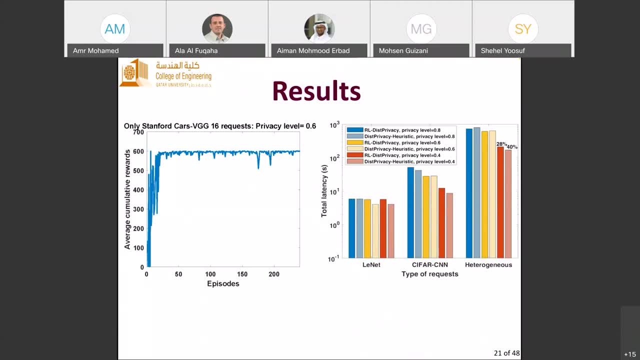 So, of course, typically the first thing we do for reinforcement learning is to analyze the conversions of the algorithm, And this result here shows you that the algorithm is designed to reduce the latency subject to the resource constraint on the IoT devices, And this is the result that I have chosen in this example, And this shows the conversions of the. 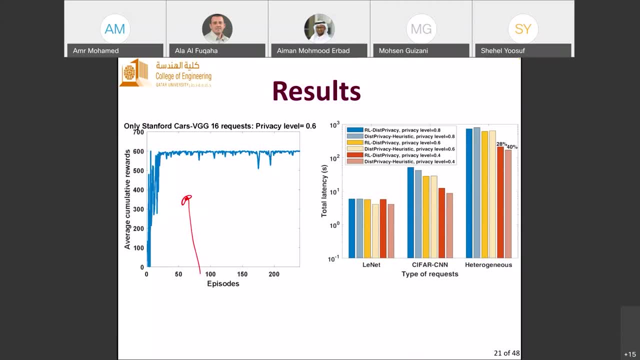 algorithm for reinforcement learning, Interestingly speaking, for the latency results here. if you notice, when we use one homogeneous machine learning model for all the requests, the incoming requests, we see that in comparison to the heuristic technique that we talked about before, the 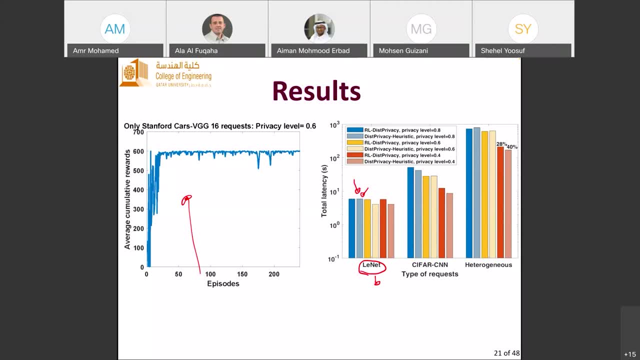 reinforcement learning model is the most efficient one, And this is because the algorithm is learning unexpectedly, does not outperform the heuristic. So that shows that, on one hand, the heuristic algorithm that we have devised before is really efficient and is really robust in giving good performance. 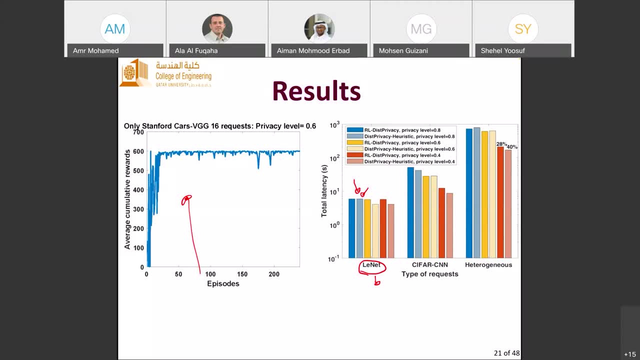 for the latency, But, more importantly, because of the fact that the requests are homogeneous, so there is no stochastic nature of these requests, where the machine learning model of the reinforcement learning agent does not have to learn a specific pattern of these requests. So that's why the reinforcement learning in terms of latency, 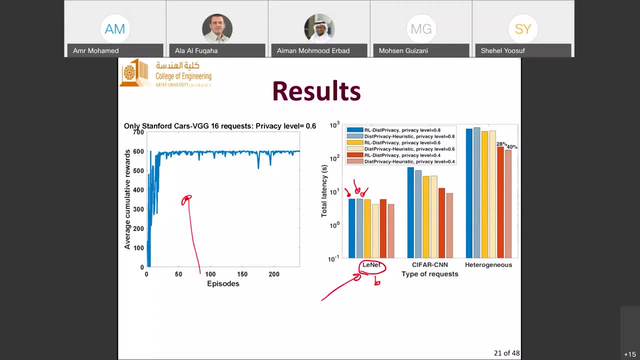 does not outperform the heuristic technique as we would have expected. That's why we tried to study the heterogeneous case where the incoming request- That's good- actually have different CNN models based on some probabilistic aspect. So that's when we start to have some performance enhancement. 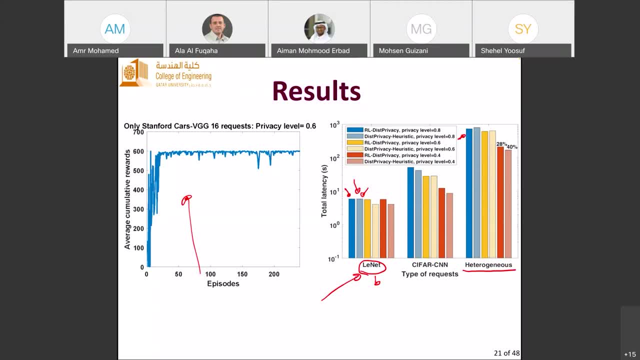 for reinforcement learning And we started to see some less requests rejection as opposed to the heuristic technique. So for reinforcement learning we started to see 28% request rejection as opposed to 40% for the case of the heuristic technique. So that gives us at least some insightful conclusion. 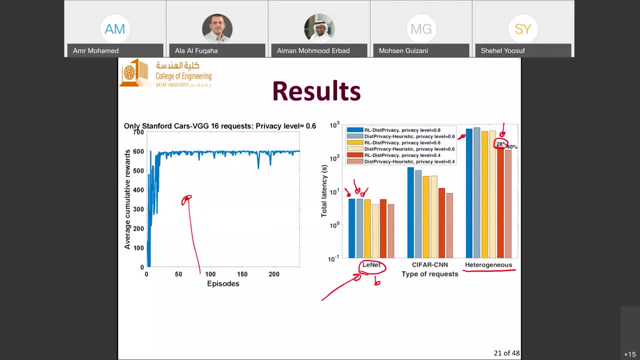 that reinforcement learning is not really the magic word for all optimization problems. So if your problem has some stochastic nature and there is some stochastic process that it needs to be learned by the deep reinforcement learning, that's when reinforcement learning really becomes an efficient tool for optimization. 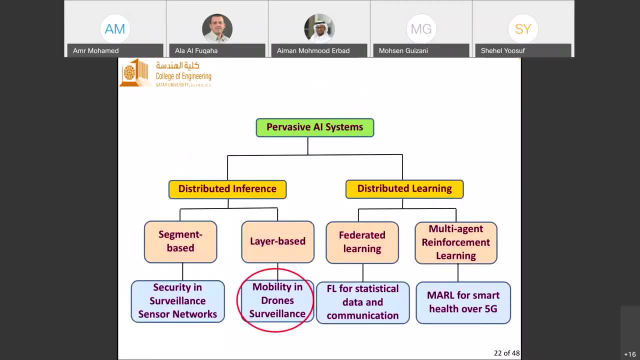 All right. So moving on to the second use case where Dr Amr, I don't know if people have questions at this point. Yeah, yeah, But I was wondering, just to give maybe 30 seconds people, if people want to reflect. 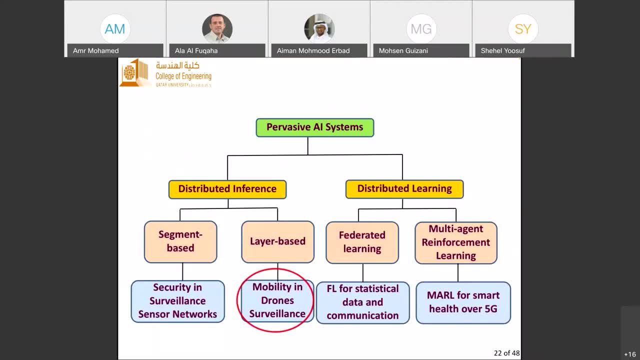 Yes, Yeah, I think you have a very good point here. Yes, So I need to pause here and wait for some questions, if you have any, And I would be glad to answer any question you might have. Yes, Yeah, So go ahead. 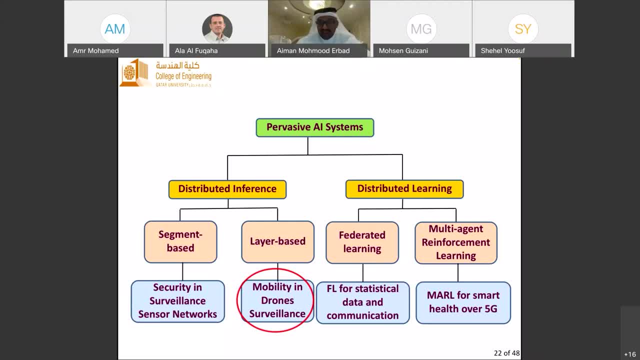 Do you have a question? So does anybody have a question? So I have a small question just related to so. do you believe, Dr Amr? Yes, Yes, Yes. Do you believe the reinforcement learning in this case will give you better outcome with more complex 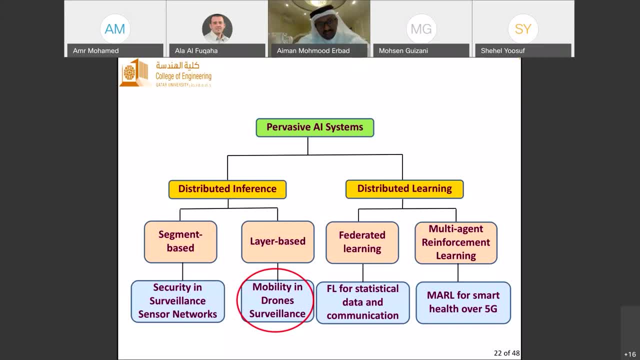 like you are seeing here, with maybe VGG or maybe with more complex type of machine learning model, Do you think it will get better results? The real value of reinforcement learning comes when you have- when you have, uh- A probabilistic state transition off the system. 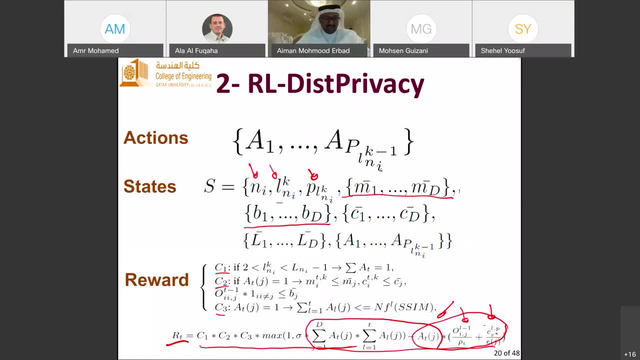 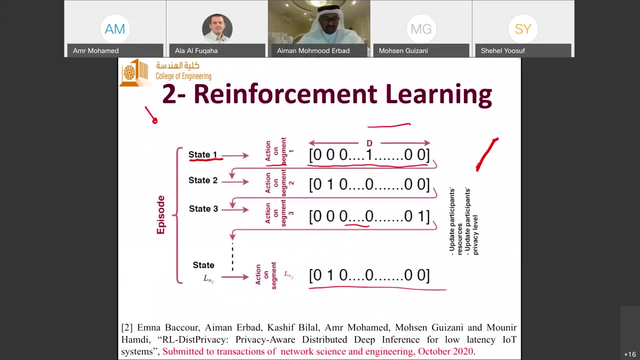 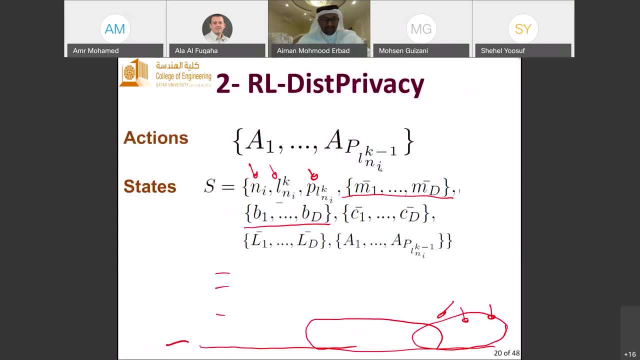 Okay, so the system is not deterministic, because if the system is deterministic, really reinforcement learning does not, uh uh, it's not that efficient, or it doesn't really provide the, the performance that you would expect. So that I I actually explained that, um. 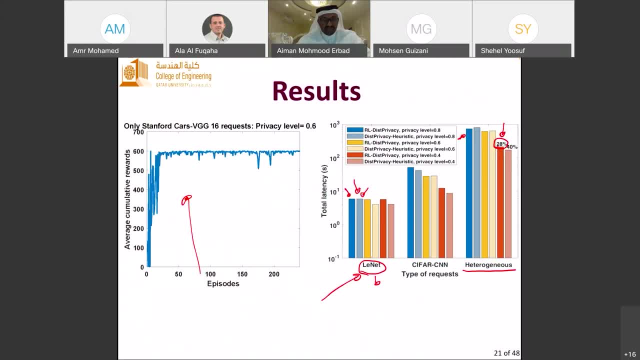 Here in the results. so if you, if like, when, when you have incoming requests that use the same type of machine learning model, So in that case, regardless of the arrival process of these, of these requests, these requests are homogeneous. 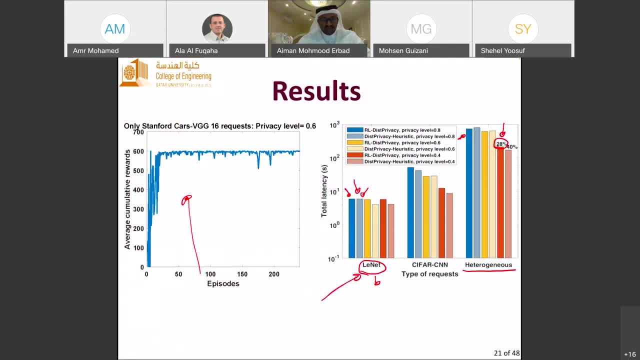 In which case the requirement, the requirement for each request, is actually deterministic. So you know exactly beforehand what machine learning model you want to distribute At which point of time. Okay, because they are all the same right. So that's why actually the the reinforcement learning, as you can see here in terms of latency. 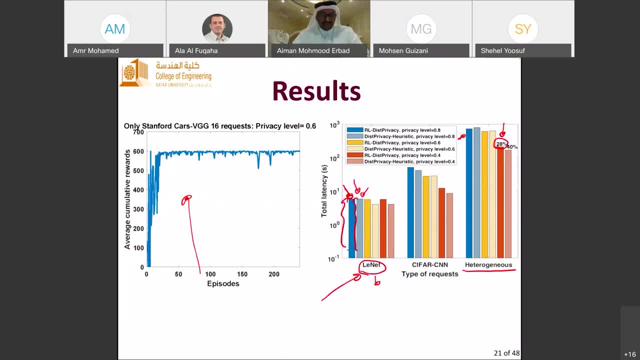 The latency here is is similar to the heuristic, and in some cases it's actually uh uh. in some cases it's less, slightly less, and in some cases it's more, Okay, so uh uh. so in this case, for example, the heuristic outperforms the reinforcement learning. 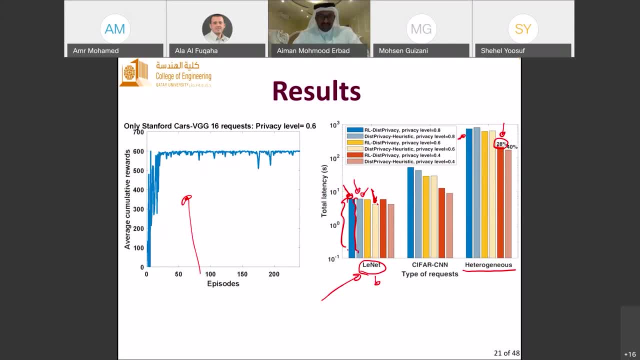 Okay, The heuristic based on greedy uh uh uh algorithm that we have explained really slightly outperforms the reinforcement learning, because the requests are homogeneous. homogeneous in the sense that they are. they are all based on 1 machine learning model, which is like, for example, or, uh, or something like that. 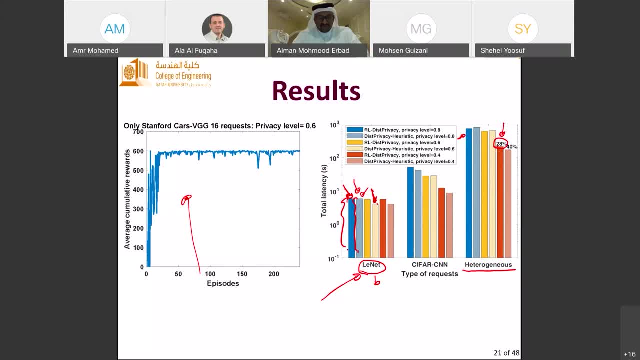 Right, if the incoming requests They probabilistically use Difficult, Different machine learning models, then you have to. you have to kind of predict, You have to have a sense of prediction. Okay, like after some time, after like 2, 3 minutes or something, most probably I'm going to have a which is very, very intensive in terms of computation. 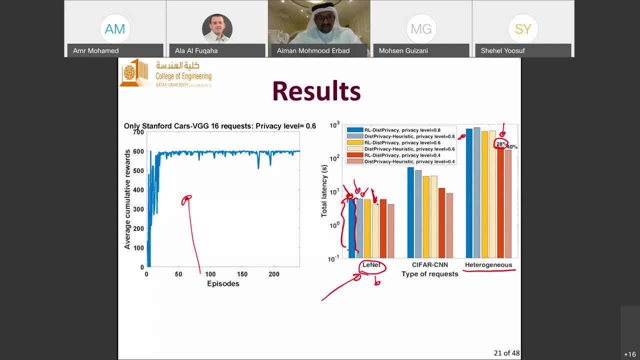 So I better try to clear my memory of the devices from now So I prepare myself beforehand For the upcoming intensive request. That's what reinforcement learning is good at- Right, yes, but if, if there is no such prediction required And everything is deterministic, the greedy algorithm is good enough, In fact, it may actually, in fact, in some cases outperform uh reinforcement journey, because reinforcement learning is based on sub optimal actions at specific point. 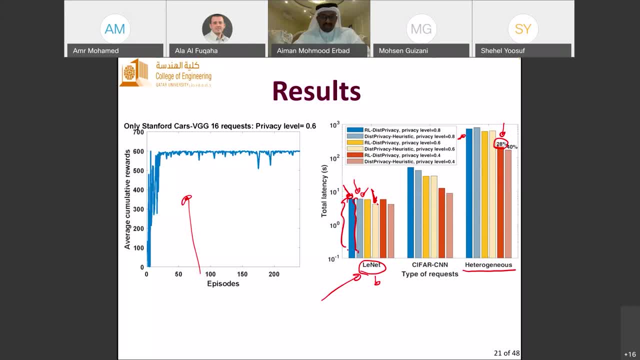 Of time, but, but, but. these sub optimal actions are are believed to lead to very good performance on the long term, not on the short. Yes, right, so that's that's where reinforcement learning is really powerful. if you don't have this configuration in your system- and the states of your system is kind of deterministic- reinforcement learning is not going to give you any- uh, any- better performance. 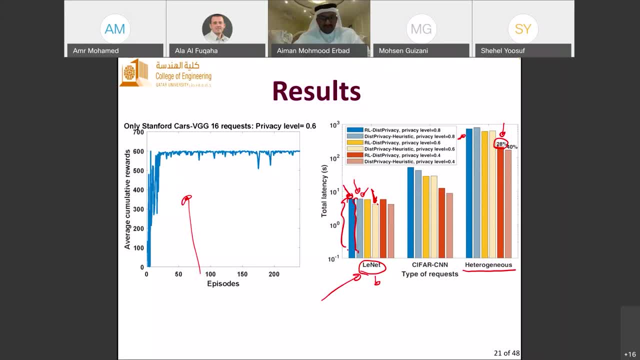 As you would, as you would, as you would expect. Okay, so yeah, this is based on the fact that reinforcement learning uh are fundamental, fundamentally based on uh the market decision process, and it's uh the fundamentals or the key engine of reinforcement learning is based on market decision process. 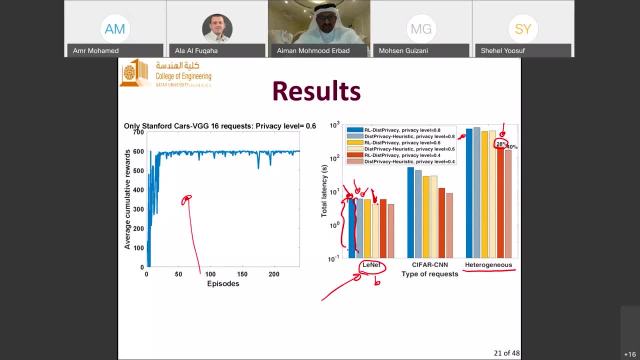 So it's based on the fact that the state transition of the system is stochastic and there is certain transition probabilities from 1 state to another. So what reinforcement Learning tries to do is to device the policy that would lead to the best transition from 1 state to another that, over time, would lead to a good performance. 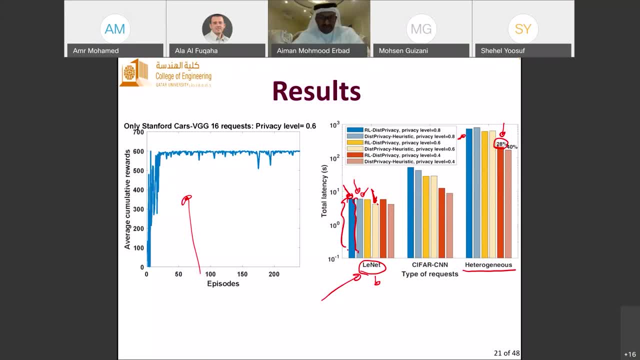 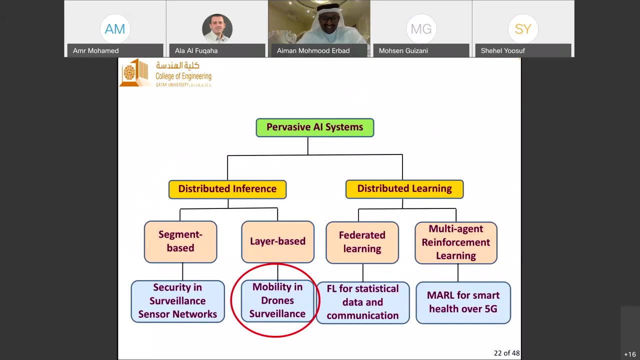 Yes, yeah, I, I, I actually Yeah. and recovering reinforcement claiming requires requires a full course on its own. here We're just trying to move fast. Yes, so the 2nd use case, and I have a question. 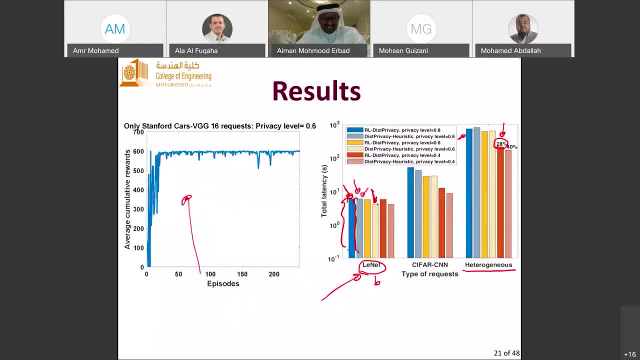 Sorry, Dr, how are you doing? Sorry, Yeah, so, and I just want to elaborate more on this reinforcement, So, in this case, so the probabilistic here is terms of: uh, the request that's coming. So, yeah, this is your probabilistic. 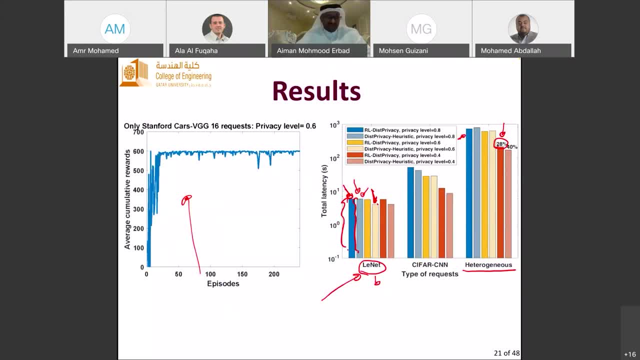 So you have in your request some like uh mark of model process that your reinforcement, learning and try to detect. That's what this, that's what it say, That's right, Exactly, Exactly. So the probabilistic nature in this context here is based on the fact that 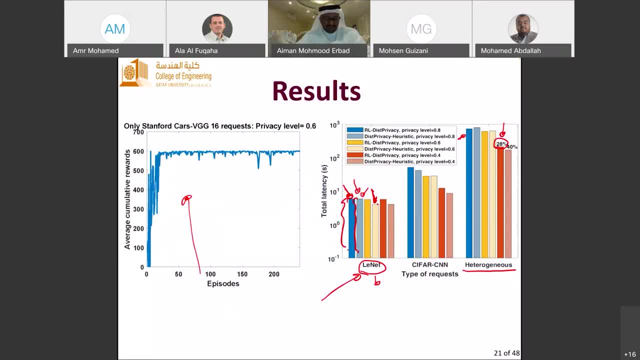 You don't know what is the machine learning model you will distribute next. It could be, uh, it could be like it could be a lead, could be anything, and Yeah, so that's the probabilistic nature. That's really reinforcement. Learning starts to have some performance enhancement and backings, But if all of all of the requests are the same, they are homogeneous. 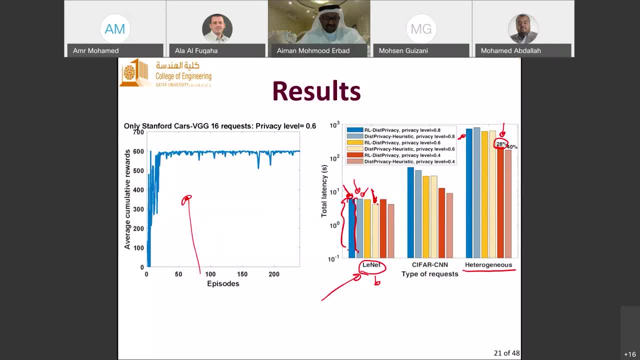 Okay, then there is no benefit of using reinforcement learning and the heuristic technique Can perform, uh, the same, if not, if not even better. so sorry, i mean, maybe my question is kind of behind me. so if the so and understand that you are trying to to select which iot device you are going to pick, 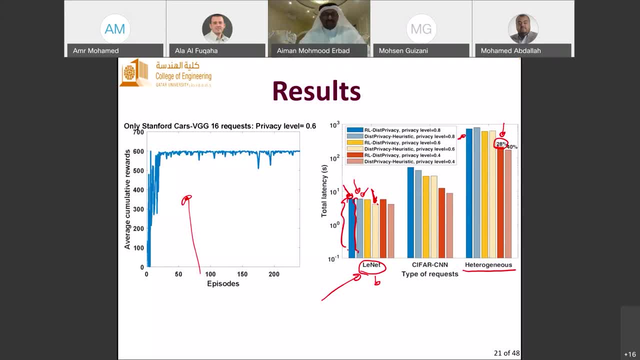 to optimize your resources. that's right. to optimize your performance of them. so does the reinforcement learning authors trying to learn this? yeah, i mean how he is going to optimize or find the optimality, or is always trying to detect what's coming and then so i need to know how, how? 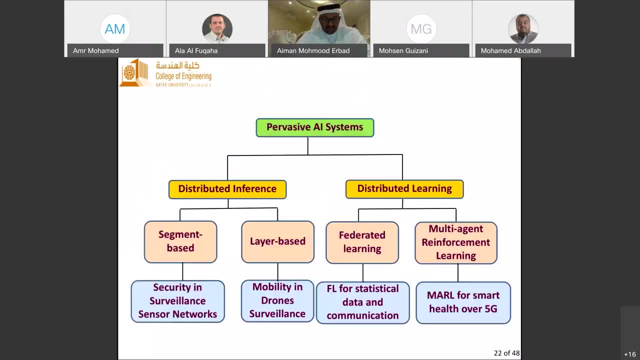 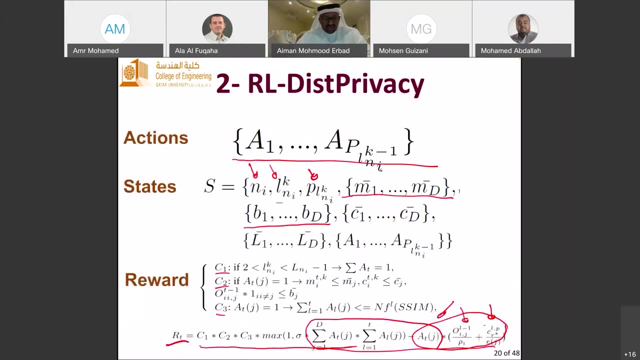 the reinforcement learning with the two system are working. oh what if? oh sorry, oh sorry, i need to go back. uh, so the objective here dr muhammad is to try to, is to try to perform an action, and this action, in that case, is what segment of the machine learning model, okay, run on a specific iot? 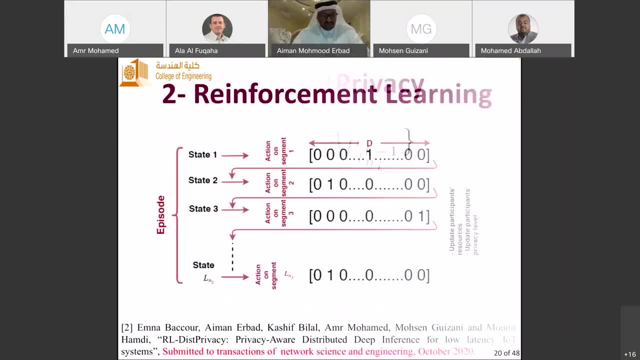 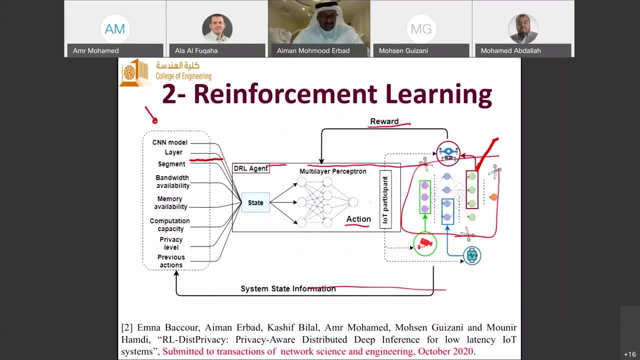 device and by exact learning model here. yes, so we have, we have the, we have. this is the tree learning model. okay, it's a complicated model. okay, so we divide that cnn model into small segments. okay, okay, yes, yes, yes. so these segments should be strategically distributed on the iot devices in such a way that minimizes the latency. 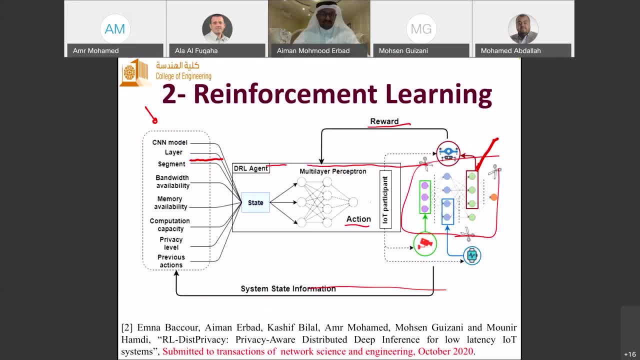 of the inference operation end-to-end. yes, okay, so, based on the incoming request, this drl agent will try to learn that now these segments should be positioned on these iot devices in that way so that in the future, when i get more intensive requests, i need to position them on different iot devices so that. 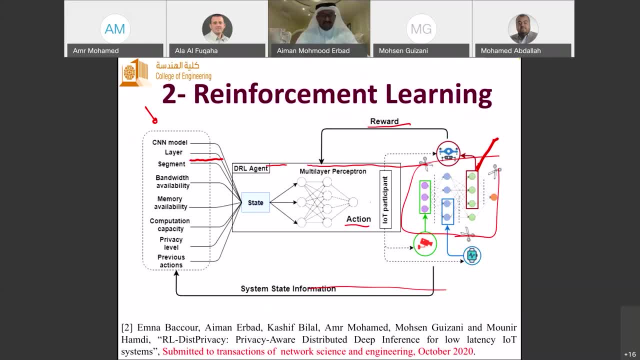 i enhance the performance in terms of end-to-end latency. is that clear? so that's yeah, so that's yeah, exactly, and thanks a lot. uh, gains for both of these segments. this time about cloud reserve and 일반 house. this is the same, so theosed. 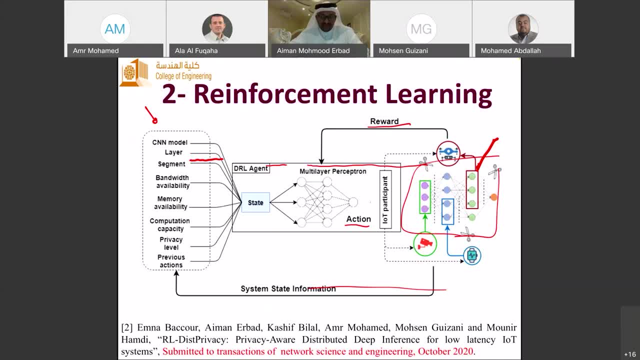 how to processlaubes for job support, data performance, but but try to optimize the. yeah, you see what I mean. So you optimize the log. if you look at the whole, it's a log term over average. Yes, So you can estimate what's coming next. 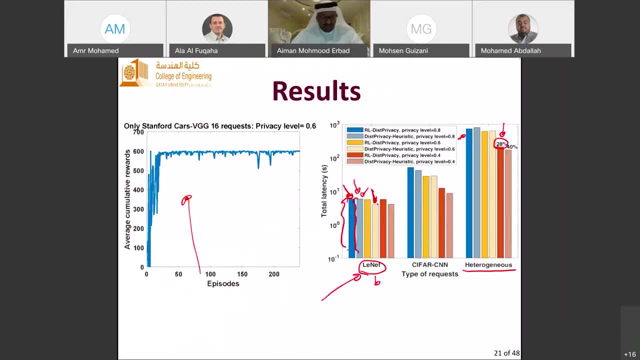 So, when you look at the whole, when you're trying to optimize the total latency, so you know what's coming next, So you can your decision now. you know cause you need to, you need to. you are predicting what's coming next. 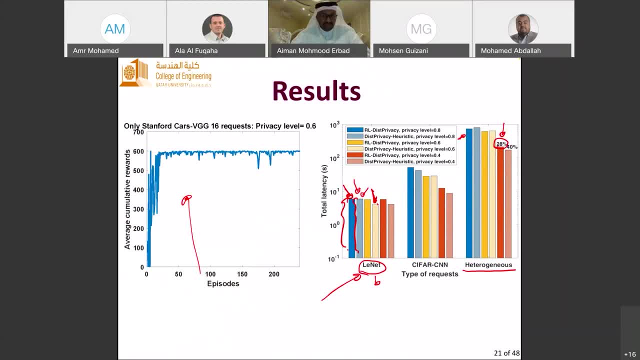 So your resources are optimized. taking the solution: what's coming next? okay, I have one, I'm sure if I, I have one last question, Manrosh. So I didn't understand the part of privacy here, How this privacy is captured in this. 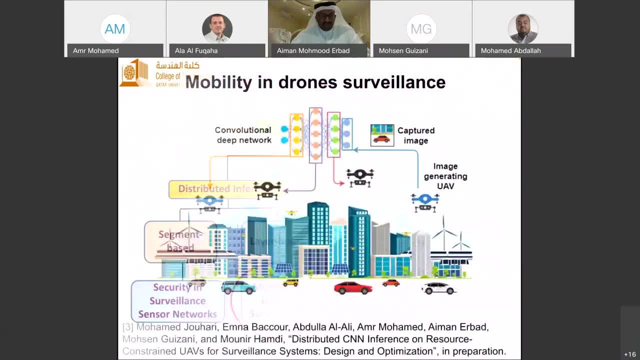 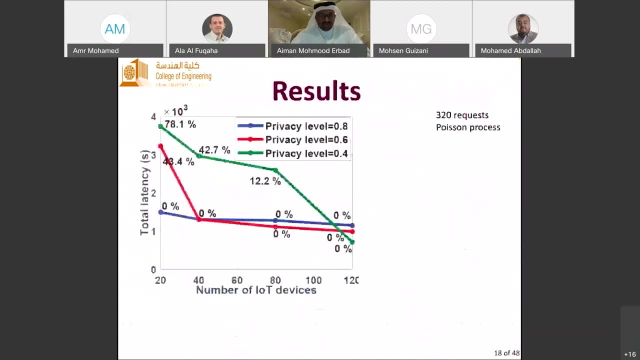 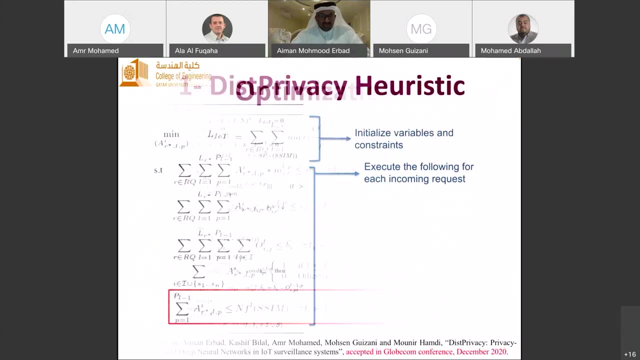 The. this is a good question. Let me, oops again, let me, let me try to explain that part again. So by privacy here we mean that if if I, for example, I put one segment in one IoT device, okay, 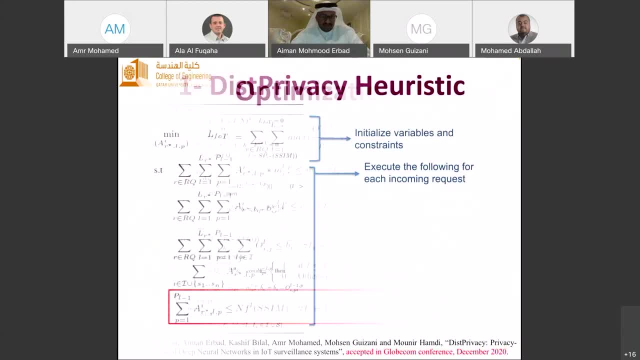 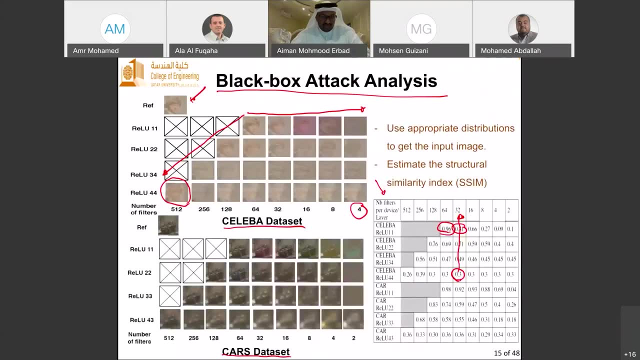 Any, any. anyone who tamper the output of this segment can easily, can easily try to reverse engineer and get to the original image. So so so this is the original image. okay, So we conducted analysis using black box attack, okay. 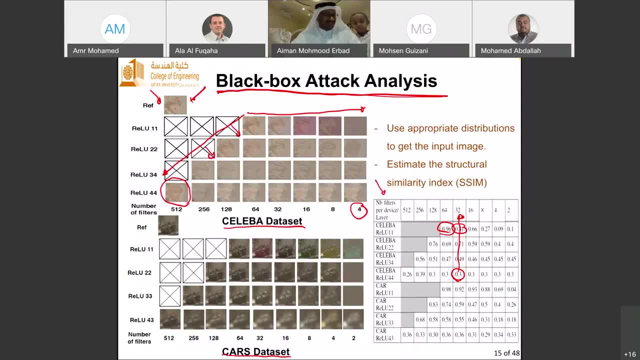 Where we try to reverse engineer the image at different layers, okay, Mm-hmm. So so logically, if we the the the deeper, okay, the deeper in the model we go, okay, the more difficult the reverse engineering would be. 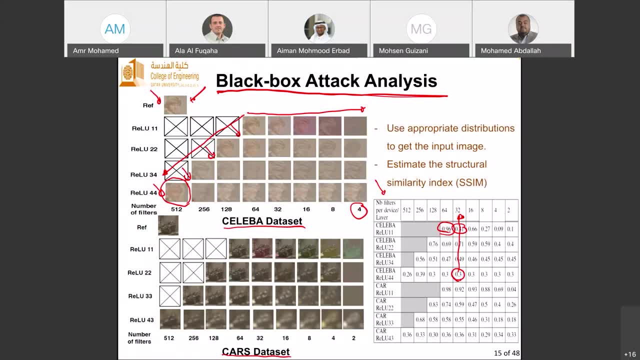 And that's. that's a fact, and this is proven through this analysis. So deeper we go in the model, okay, the the harder the reverse engineering would be. So this suggests that you need to position more layers, okay, in one device, okay. 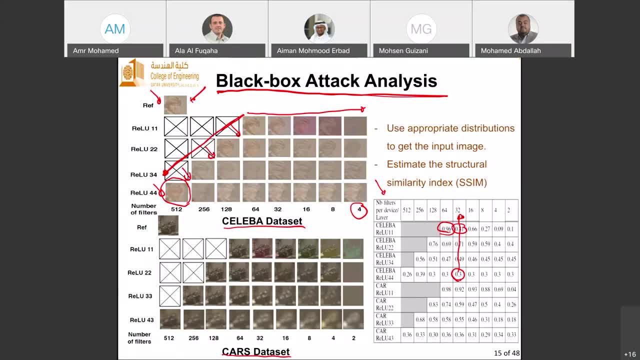 But of course, this will not give you enough degrees of freedom, because you do not have the memory and the computational requirements on one IoT device, right. So we also conducted the same black box attack if you try to divide each layer into smaller segments. 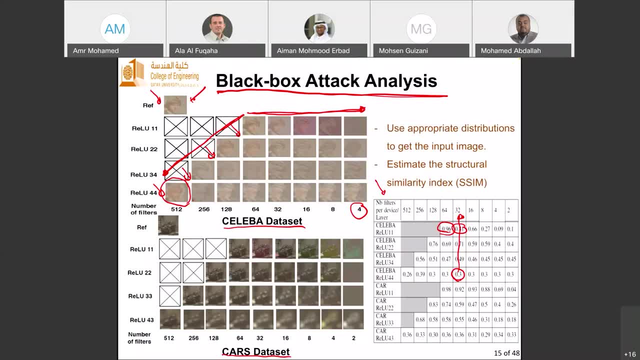 By segment here, yeah, Dr Mohamad, I mean that you have access to limited number of feature maps, basically kernel filters. Okay, fish map of features, Yeah, yeah, Which are basically kernel filters right In one device, for example, So I need to fix my computer okay. 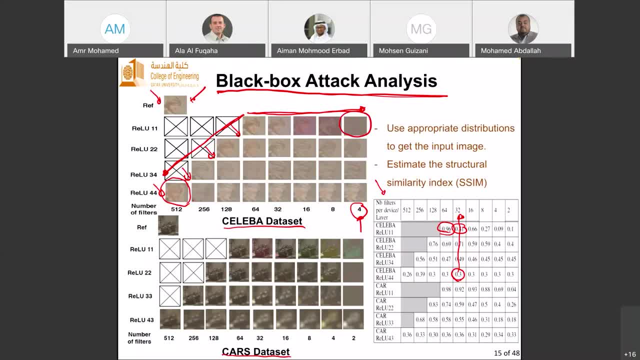 the cnn layer. so if you have access to four filters only, you cannot really reverse, engineer and get to the original image by any means. what you get is nothing related to the image. so this suggests that for security it's better to divide the layers into segments and distribute the feature maps across. 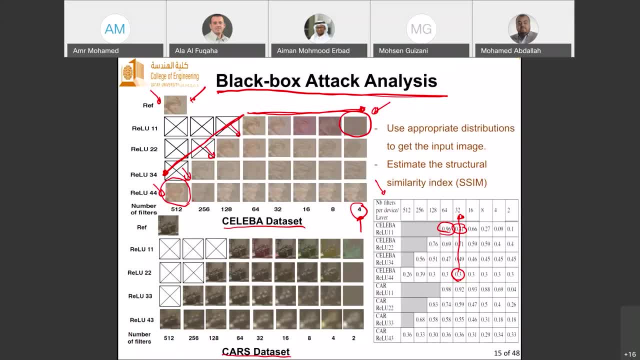 across more and more iot devices. this way you can address the privacy issue, okay. so that's why, for this particular context, we say we, we categorize it under the segment based distribution. okay, but this is related only to images, or this can apply to any type of- yeah, machine learning model or and. 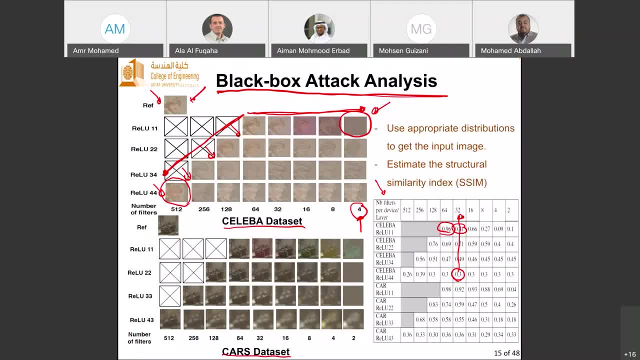 this is the understanding. yeah, it depends. it depends, you're right, it depends on the application. so in this particular application, we are using a surveillance application using uh this, uh cellipa data set or cars, and for that we use uh cipher and uh, sorry, we, we use the specific machine. 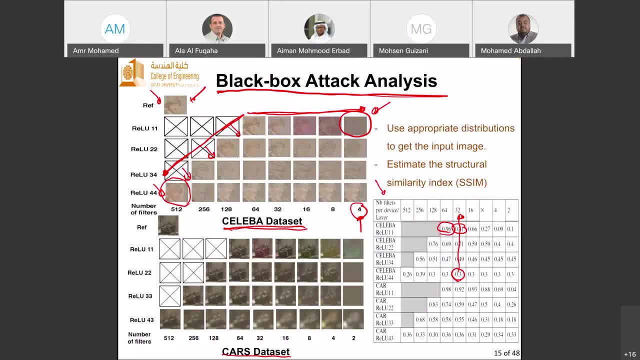 learning models like vgg16, vg19, leonard. these are some well-established machine learning models. you're right, if you for for other applications, actually distributing the segments is not needed. you can run the whole machine learning model in one single application. you can run the whole. 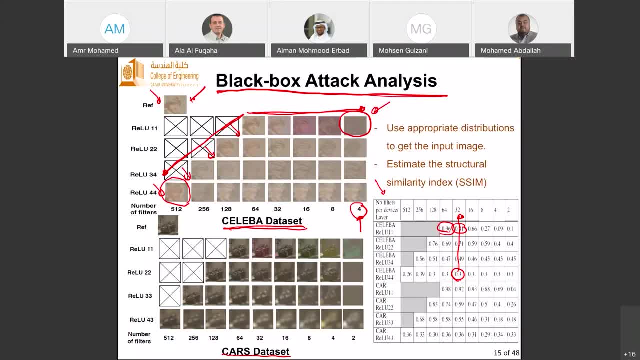 machine learning model in one single application. you can run the whole machine learning model in one machine learning model in one device and that's it, so you don't really need to distribute the nodes, in which case you can run all the machine learning model in one device and 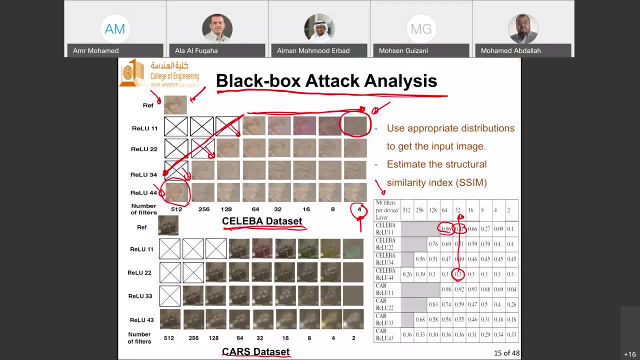 that's it. and then this is in fact the case pretty much for simple machine learning models like lenet. lenet has only two layers, two cnn layers, so you find that you can- you can really run this simply on one device. however, for security you may want to divide these two layers into segments in some 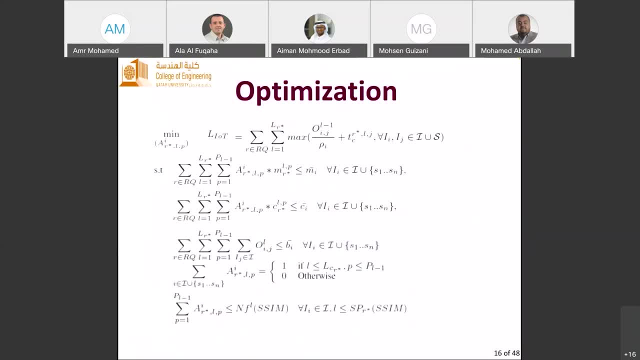 cases. okay, uh, in the results, in the results in the paper- by the way, i can send the paper to you because it's not published yet- uh, or at least one one. one of the uh based on the optimization is is accepted in globecom. uh, we, we provide the rigorous results and analysis based on. 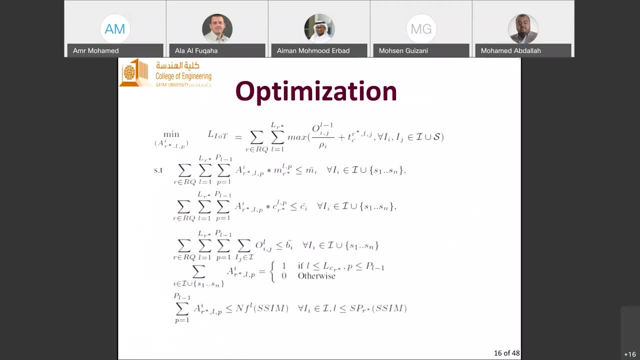 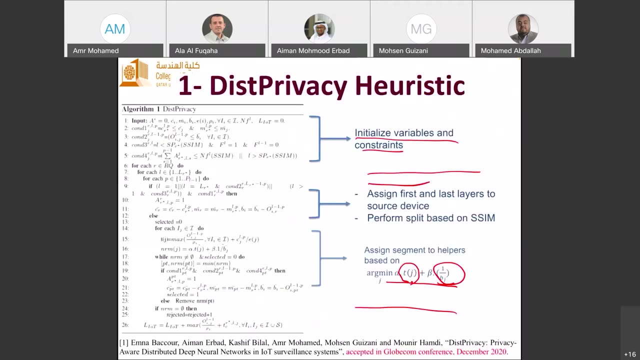 the different types of machine learning models and how they can be distributed across the different iot devices, and how many device you need to parallelize the requests and the computation for the inference operation. uh, that's excellent, yeah, good. good, i understand it better. yeah, i'm done, but unfortunately i need to leave to cover another lecture i need to give now. 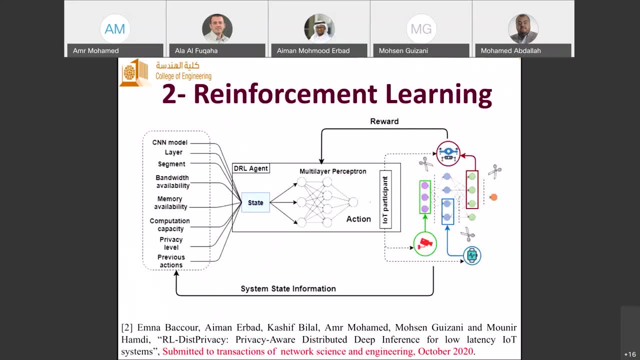 please, i, i, i need, i need to, i need the recording. huh, it's very nice. yes, yes, keep the recording. thank you, thank you, thank you. i like questions as usual. yes, very, very much for the questions, because the questions really helped to illustrate. no, you're not going fast actually, but, um, which are the amount of information? 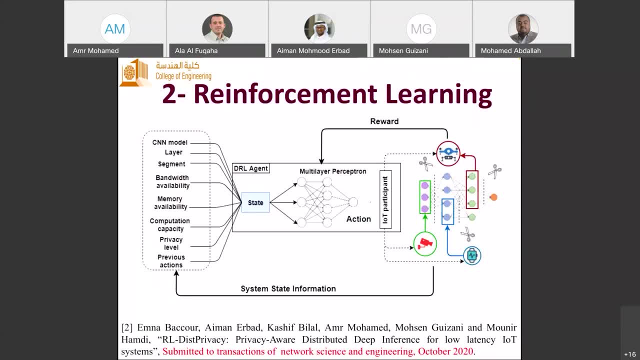 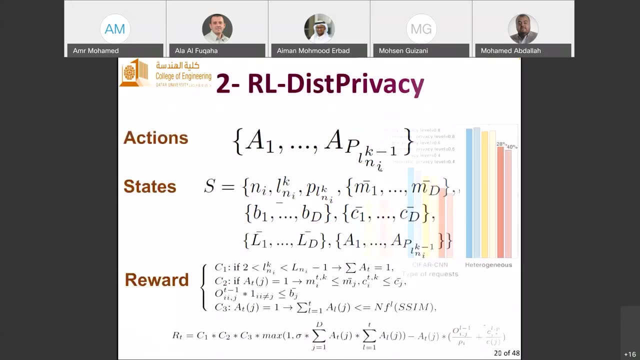 reading very well indeed, it's like we cannot- and for me i cannot- digest all of these nice things. yeah, but it's very nice and you know you're talking very well and masha'allah, okay, okay. thank you very much, Dr Amr. I have a question if you don't mind. 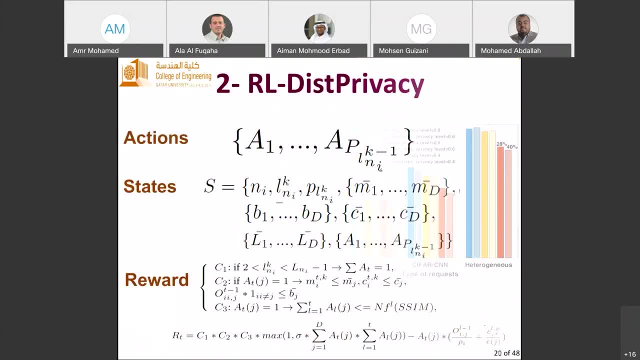 please, please. so yeah, thank you for sharing the work. you know, I don't know if you recall Amr back in the days, like I remember meeting you. I believe it was in Spain when you were talking about this stuff, just verbally, you had this vision talking about it. 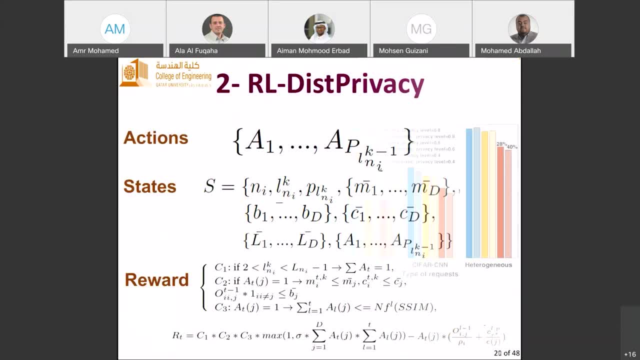 so now I see it in action, it's really very nice to see it coming along and all of this progress made. so my question is the following: I would like to carry your idea to the extreme: what happens if we just take a single neuron and just let every single IoT 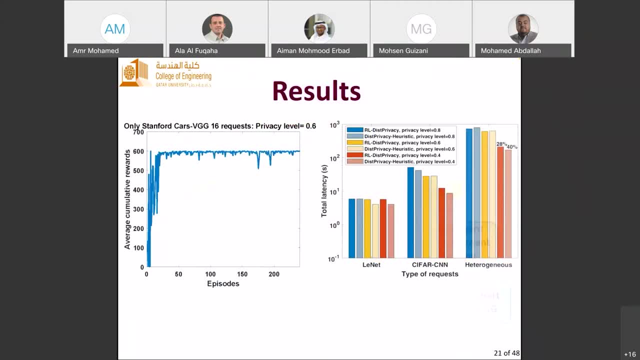 node coincide with a neuron. I know that communication will be much more, I know that latency will be much more, but do you think this kind of structure in which really the neural network is totally distributed, do you think that there is a class of applications that might benefit from this? 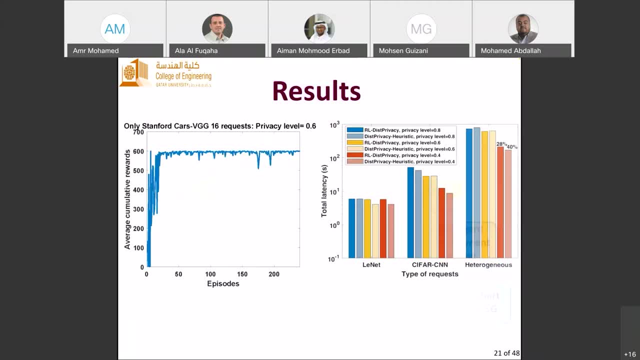 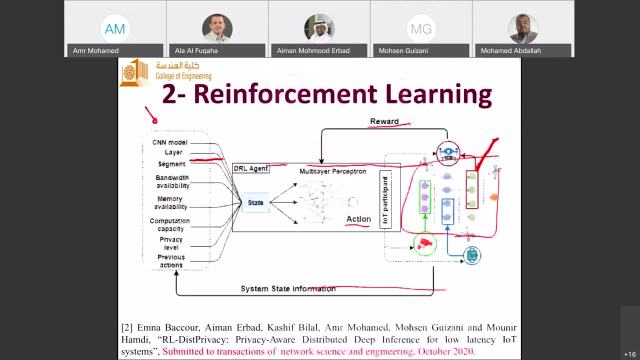 and another thought that I want to ask you about is the following: like, how do you handle the reinforcement learning? how would it handle churns? like you know, like IoT nodes come and go right, so the environment, essentially, is dynamic. so there is so the policy that you learn. 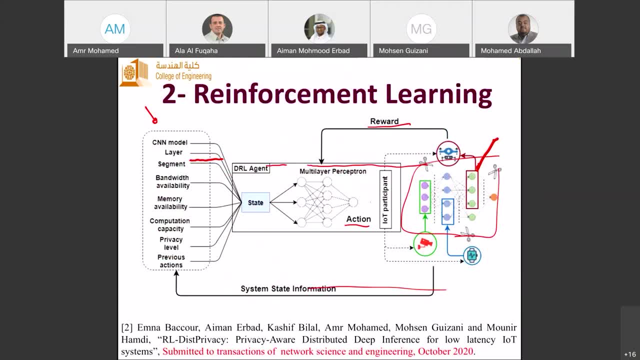 needs to- I mean, adapt to the environment as well- over time. so is that something that will delay the the policy itself or the development of the policy over time? this is a very good point. let me start from the last part. Dr Alaa, yes, you are perfectly right. 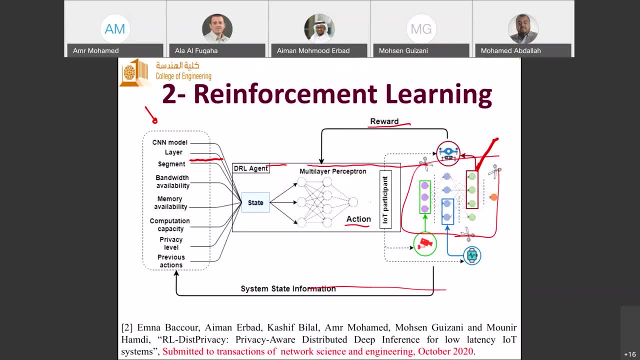 the network dynamics that we have now is very important to us and we have addressed here- are only based on the heterogeneity of the incoming requests. but you are perfectly right, if nodes come and go, that creates another dimension of network dynamics that is not addressed in this work. 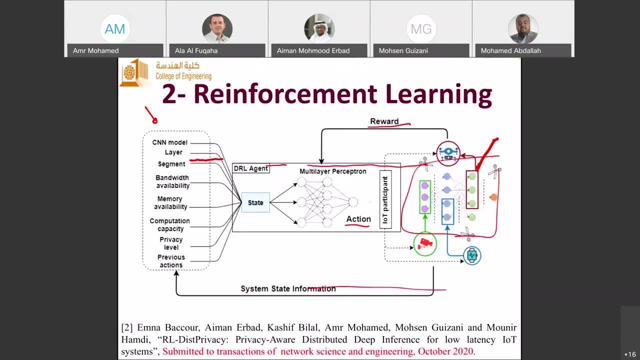 however it could. it could be really taken into consideration by again removing or adding IoT nodes into the network, probabilistically, over time, okay, and again perform the same reinforcement learning, okay on how, what is the pattern of removing and adding these devices in the network and based on that, we can, I believe, 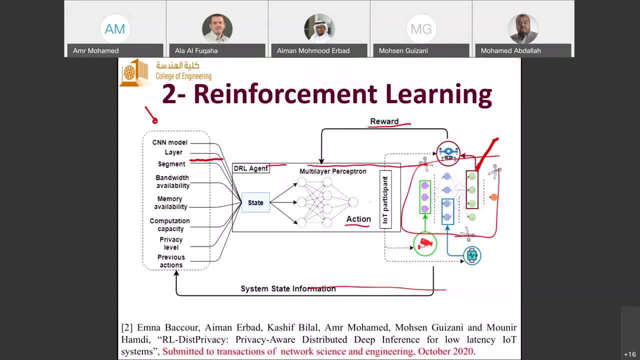 that reinforcement learning would really be a very powerful tool in that case. that would enhance the performance even more. so, the more dynamics and stochastic aspects that you introduce into the system, the more powerful the reinforcement learning will be. that's what it can do best, but again, because of the fact that 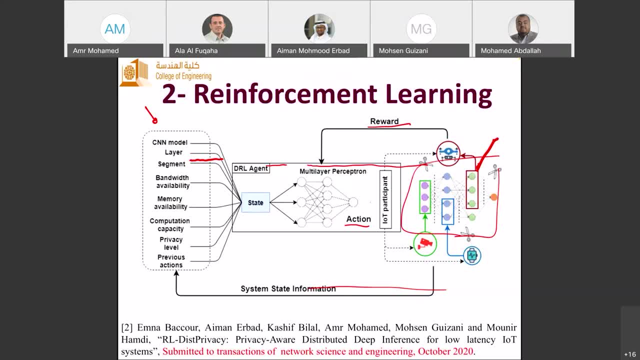 the requests were totally homogeneous at the beginning, so we did not see any performance enhancements. but you are again. you are perfectly correct. if we introduce network dynamics by adding and removing nodes, we should start to see more performance enhancements: performance enhancement for reinforcement, learning compared to the heuristic. As for 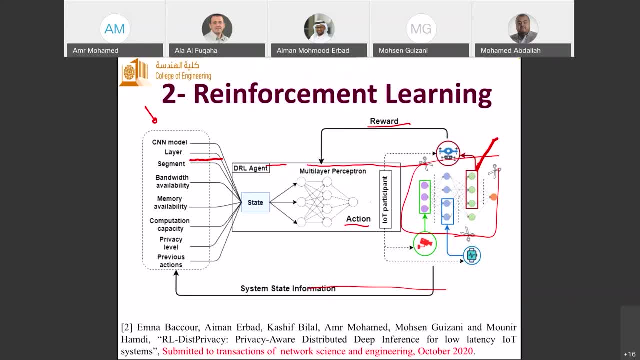 the extreme case. that's an interesting point. I really don't know, and I do not see a specific application for a single neuron IT device. I don't see why we need to do this, but it could arise in the future. I really don't know, But what we can learn from this work, by the way, 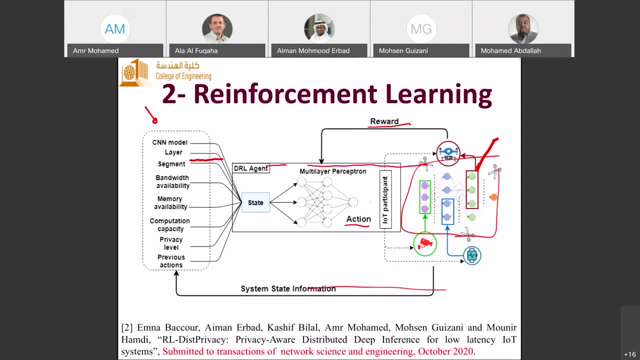 is that the smaller the segments are, the more interesting scenario you're going to have, because you need to distribute more and you need to engage more and more devices, which in fact leads to less latency. end-to-end- okay, But here what we did is that the segment 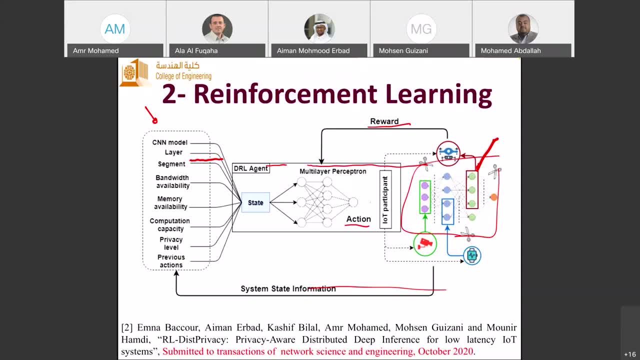 is proportional to the computational and memory resources on the IoT device. okay, So if, for example, the memory and the computational capabilities on the IoT device can handle only one neuron, then we can do that. We can do that. It's part of the work, But of course, the assumption. 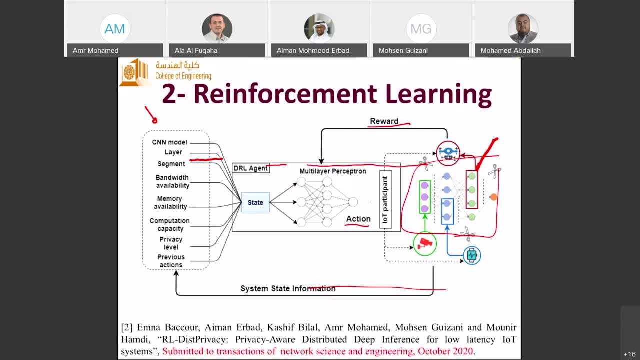 is that we have significant resources, at least even the Raspberry Pi. it has like two gigabyte memory so it can handle. So it can handle a really significant number of segments and process different segments for different requests. But for single neuron I don't know. really to be honest, I don't know if there. 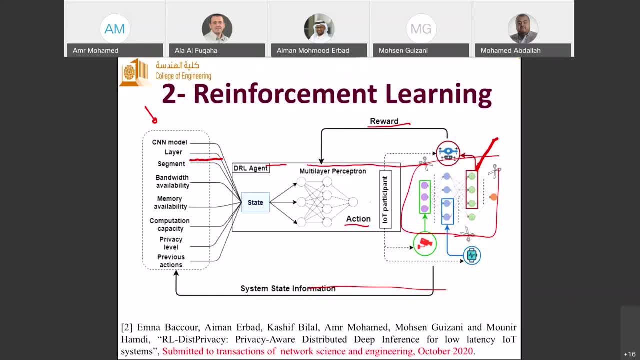 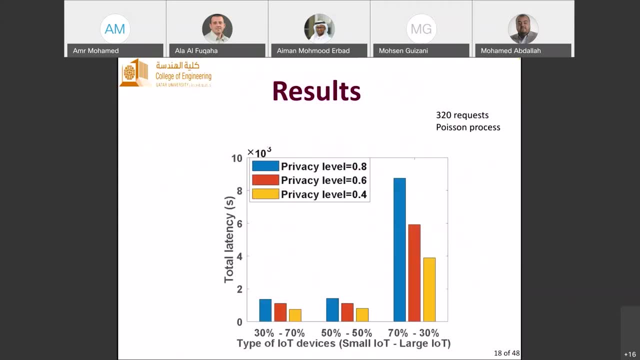 is a specific application for that. So, Dr Amr Al-Dak, don't you think that synchronization will be an issue here? Like you know, I'm concerned about synchronization is not an easy problem in here. Yes, I like these questions very much. You are perfectly right, Dr Sah. You are, you are. 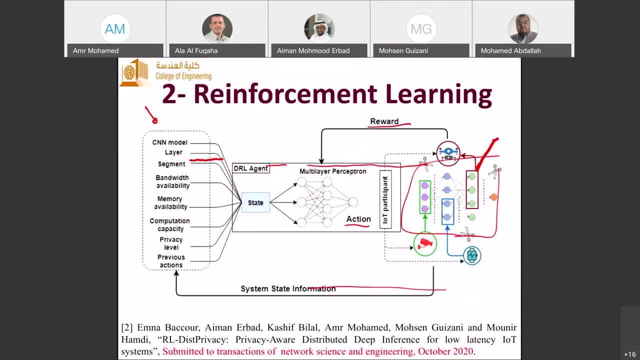 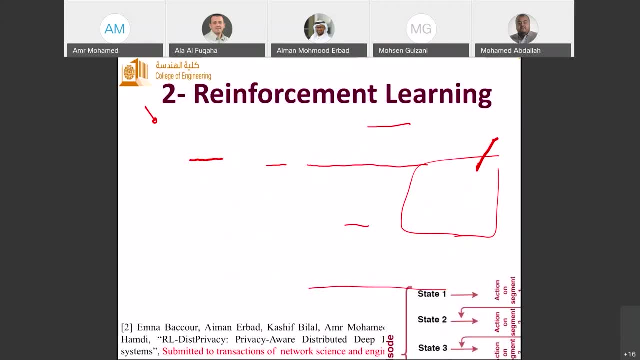 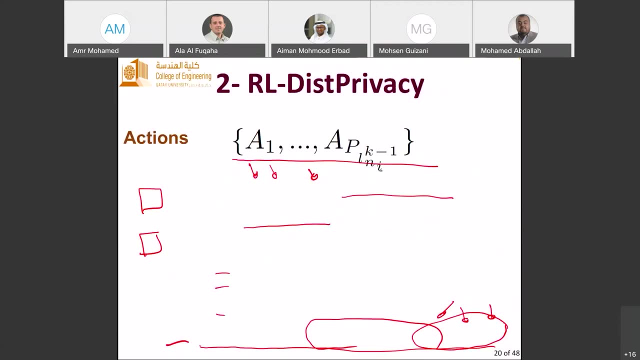 really hammering the nail really. So, yes, so so, if, if, if, here we assume perfect synchronization, because if we- I don't know if I have an empty here- if, if, if you have like segments, and then you, you, you try to distribute these segments, you're going to. 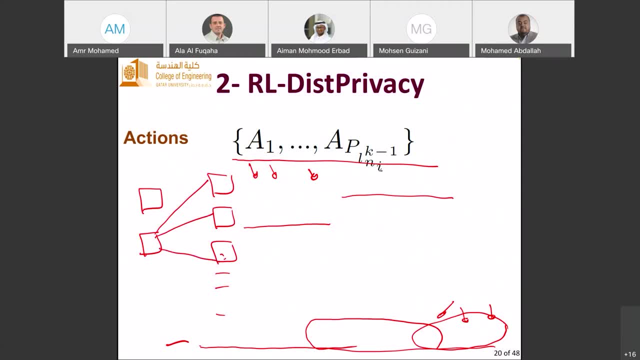 have scenarios like this where one segment would be connected to three devices in the next layer Right. So you have to assume that there is perfect synchronization here to perform the entrance operation, okay, that the output of this segment would reach all the three segments. 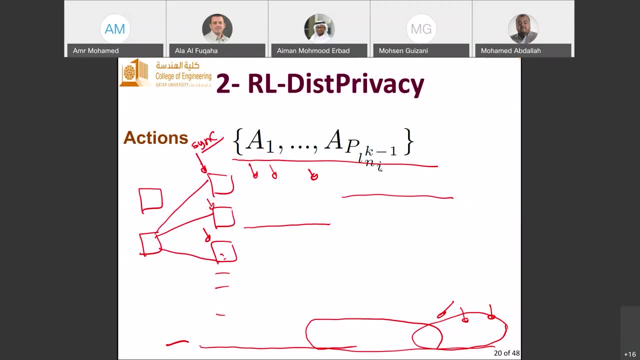 all the three devices, sorry, okay, pretty much at the same time, So you can perform the entrance. So this synchronization is implicit in this, in this model It would be. I thought about this. it would be really interesting to analyze the. 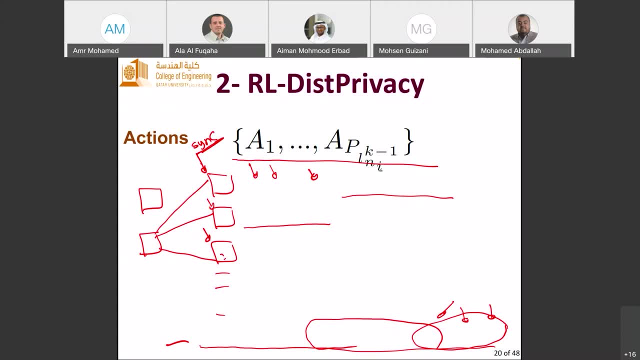 the synchrony. as part of this problem which we did, we did not address. we did not address What is the effect of asynchronous communication where the outcome from some segments they arrive at different times at different IoT devices. What is the effect of this on the 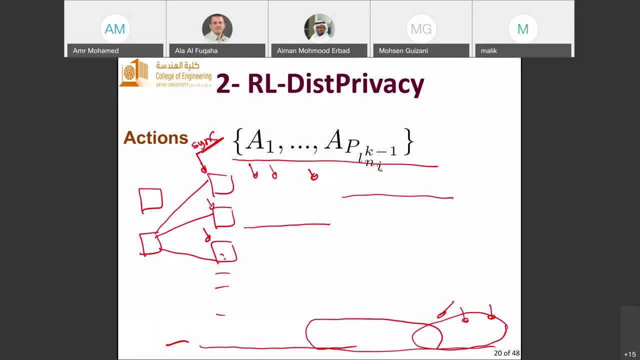 entrance operation end-to-end. I really we did not analyze that. Yes, yes, this is a really rich problem, you know. like really it's interesting. What I really like about this work is that it's different from what I see in the literature. It takes like everything that we see in the literature takes 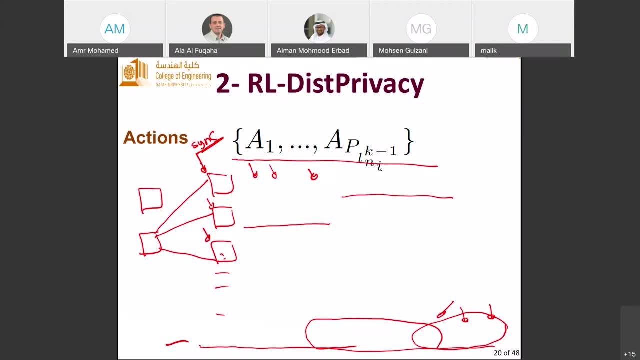 the branch of learning, the branch of, like you know, inference. I don't see much work, So this is really interesting in this sense. to be honest, Yes, that's what I highlighted at the beginning. I really for those who are interested. 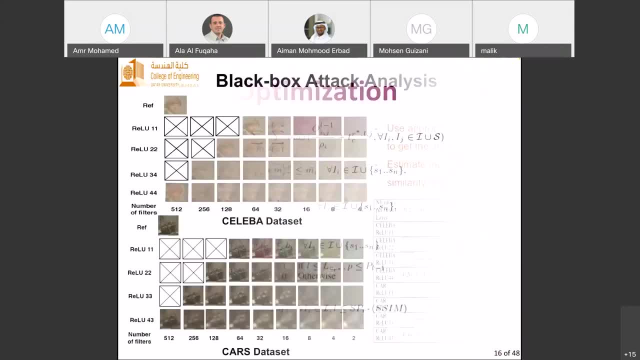 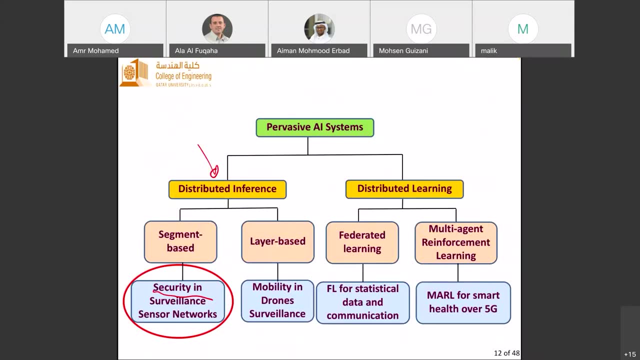 to tackle some interesting areas. the area of distributed inference is not really that widely used, uh explored, especially distributed entrance, where you have a pre-trained model and you try to distribute the entrance operation across the different iot devices. that's not, that's not in. 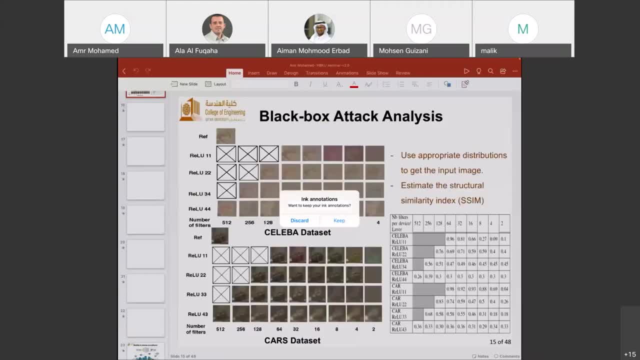 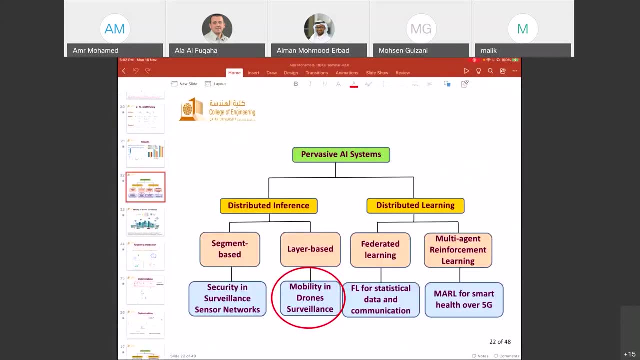 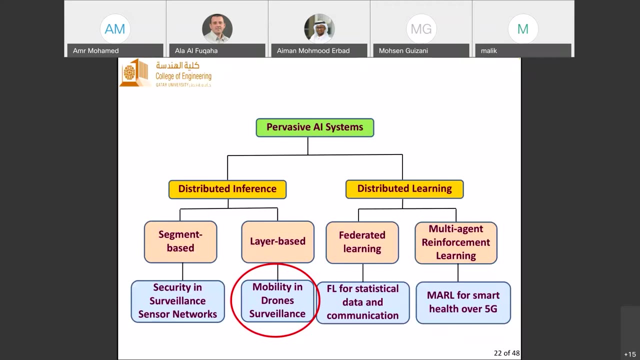 in the literature and we, we plan to have a paper about, about this particular work. really, um, i don't know. do you, do you want to move to the next one? so maybe if we will take a break for, uh, maybe five, ten minutes, and then, uh, we continue with. 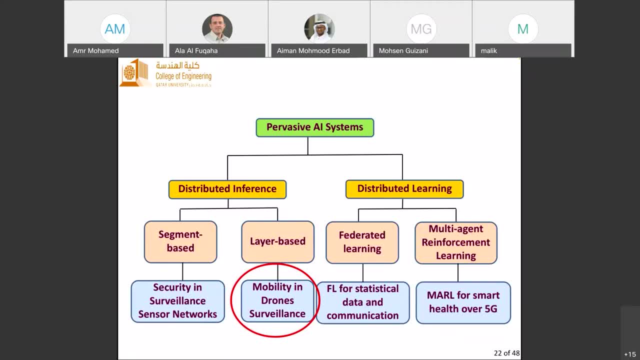 whoever wants to continue. i think our students are here so we can continue with them. uh, but what do you feel? because i feel it's some other time, so maybe, maybe we need to take uh like maximum 10 minutes and then continue with the students, but if your second part will, 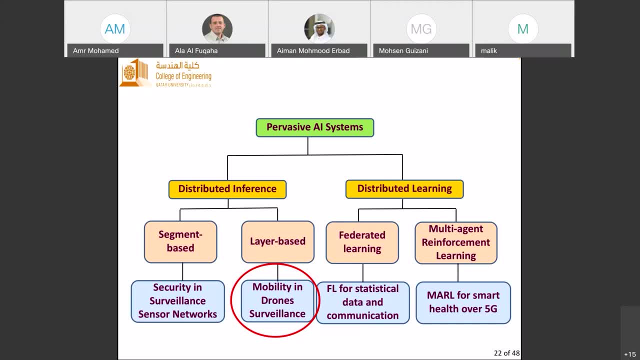 finish quickly. maybe we can finish it and then take a break up to the doctor. we have finished one quarter, okay. okay, then, because they know that we have three minutes. no, no, inshallah, we'll continue with this, so with the students and anybody who wants to continue. so 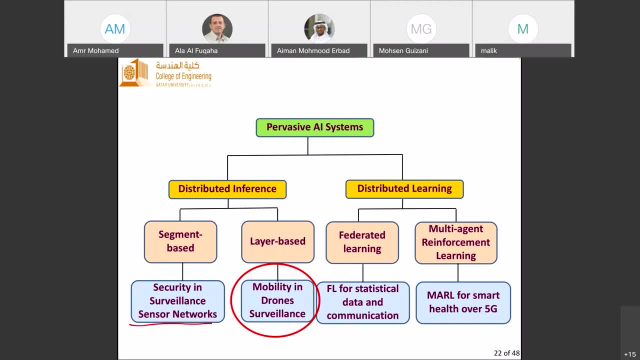 we'll take maybe 10 minutes break, we will go pray, we'll come back at 5: 10.. okay, let's try to come back. i can cover. i can cover the layer based model, because this one is uh pretty quick, and and then maybe leave the distributed learning to to another time. it's up to you, yeah, but we can decide after. 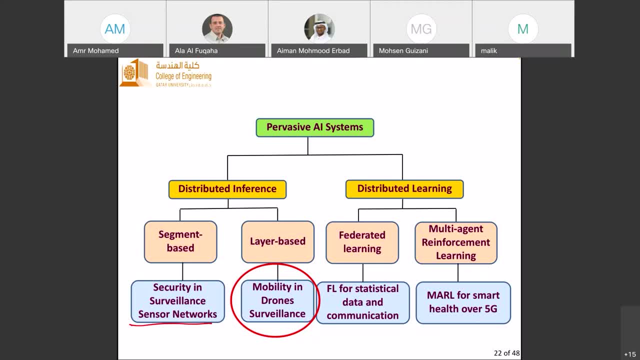 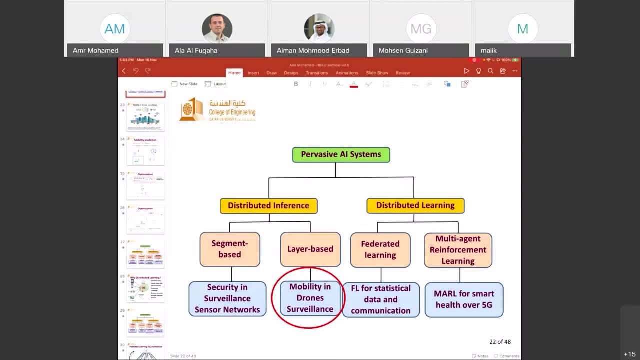 we come back inshallah, so we'll have to. yes, yes, inshallah, thank you, thank you. so we'll be here, we'll be back in 10 minutes and then we will continue with the distributed inference, and maybe it's a beautiful learning, thank you. 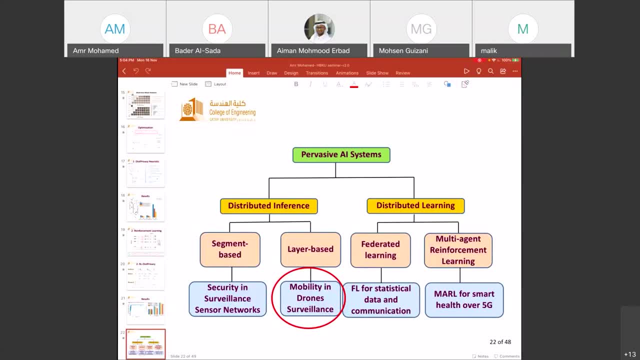 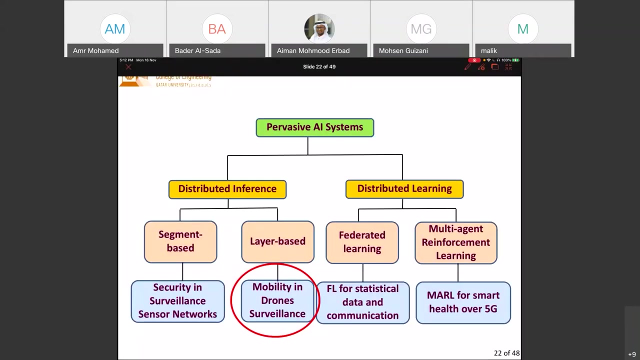 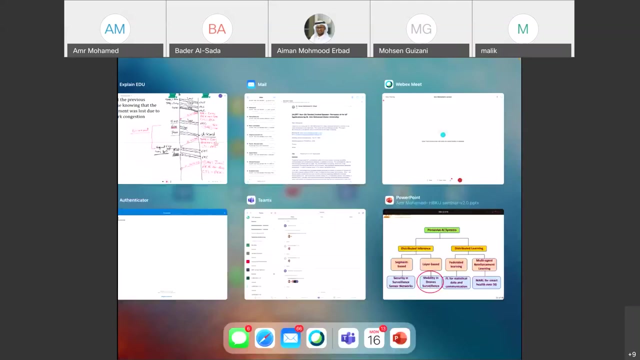 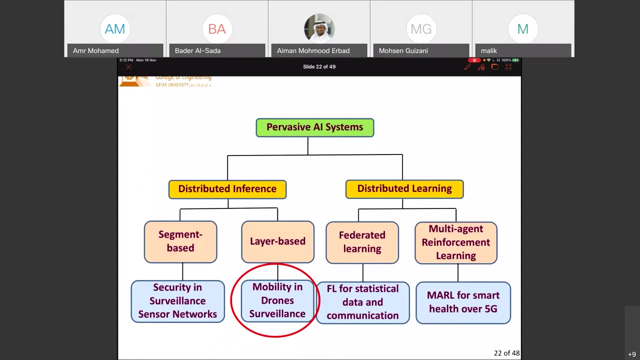 you what? so? our student and actually a lot of our uh audience is with us too, so so we'll start go ahead. i hope we did not uh. poor people with lots of information and they got bored. it was. it was very good actually for that paper. it was very good, but it took its time. it's like a whole piece of work. 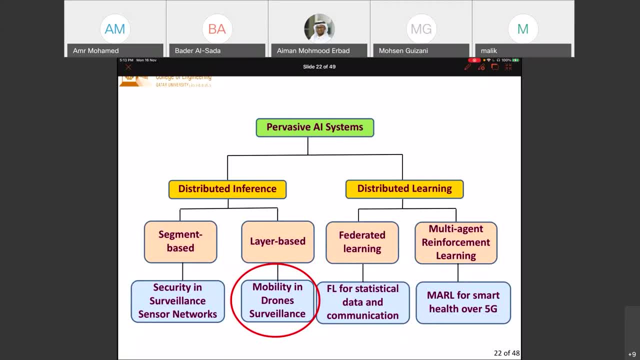 yes, um, yeah, yeah, i covered actually two papers, not, uh, not not one. yes, two papers, yeah, yes, and i tried to train, to train myself. in the meantime, i can wrestle. uh, writing too too much lines on the, on the, on the slide, and i was not able to clear them. so i i knew how to do that. so 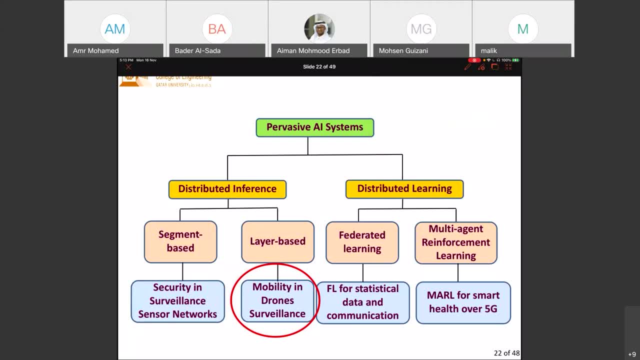 i'm learning new tricks anyway. so, uh as another, uh, uh as another, uh. sub branch for, uh, the iot network. we have a distributed inference where we talk about layer base. so we have motivated the segment based distribution. uh, for the machine learning model, for the particular case, for: 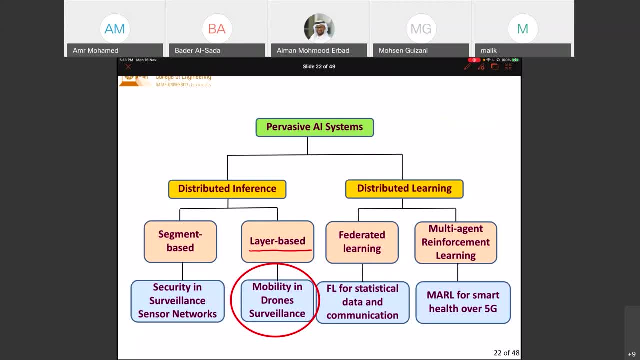 addressing particular issues related to security, and we have shown that through the black box analysis that we have done. if, if security is not an issue, uh, for uh, the uh, the iot network, in that way the layer base is actually possible and, in fact, uh, it's even more desirable because, if you have, 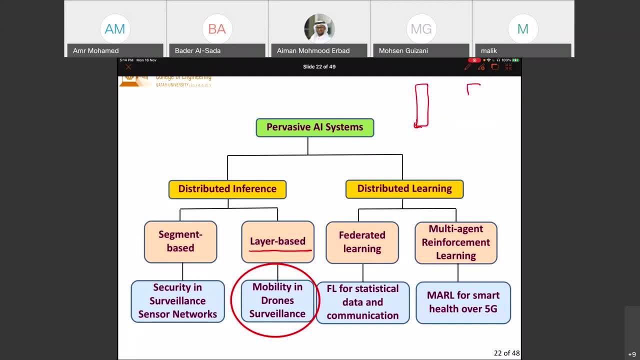 a layer uh in one device, another layer in another iot device, so have one to one communication link so you don't have this one to many uh communication links that you need to address synchronization and all of this, so that doesn't have to be addressed for the layer of this. so the layer 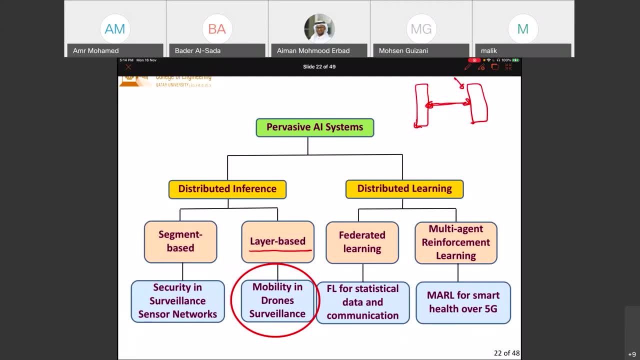 layer basis is a cleaner way of distributing the machine learning model. however, it's not possible in all cases, particularly for security issues. so this layer base tries tries to address another aspect or dimension for network dynamics, which, in that case, mobility in a multi-drone system. so again, multi-drone systems are. 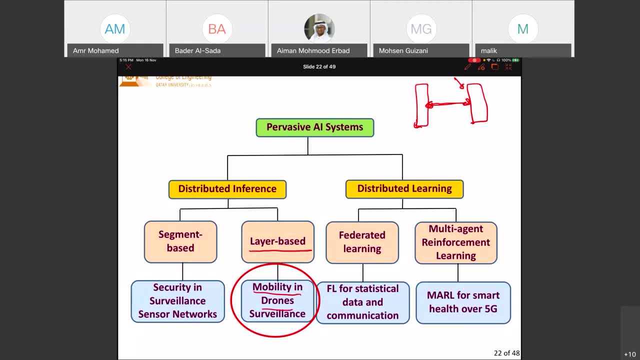 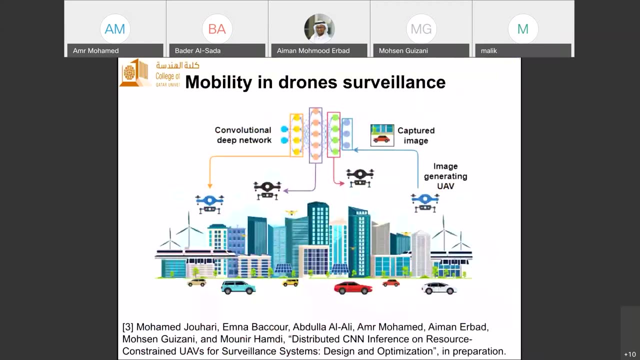 very commonly known to perform intensive surveillance and inference operations and in that case the drones: they lie and they they. they are mobile in nature. so for that particular case, we need to divide the machine learning model. in that case, layer based distribution, where we divide the different layers. 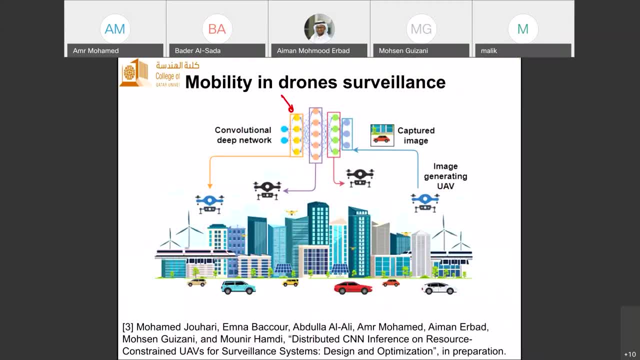 across the different drones. in that case, while we try to address again the resource limitations on each drone in terms of memory and computation, but more importantly trying to address the mobility aspects of these drones, because if you assume that you have one here and one layer here and these two drones, after like two or three seconds, they come, they, they become out of range. 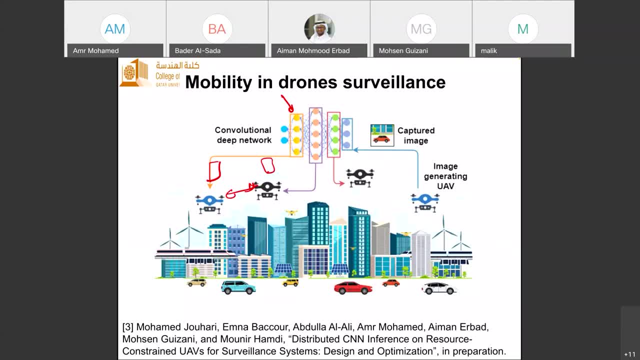 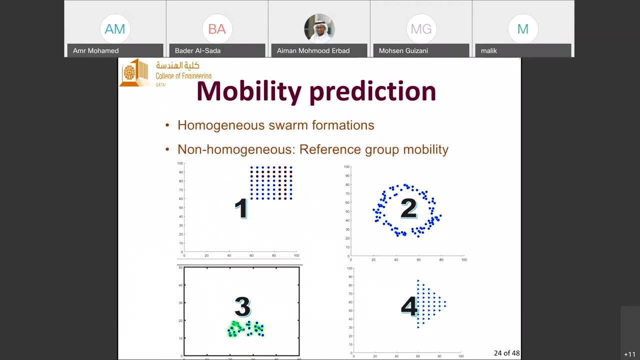 or out of range of each other. the inference operation will not be feasible in that case. okay, so we have to strategically position the layers in such a way that takes into consideration the mobility patterns of these drones. we have done some mobility analysis in that case, where we studied the different 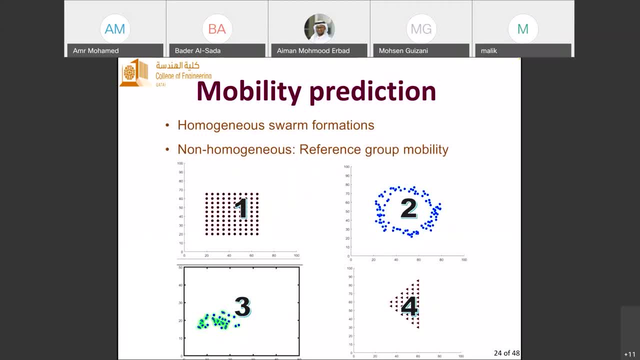 mobility patterns for the drone swarm formations, and we we classified the mobility aspects of the drone into home form formations. homogeneous swarm formations are like one, two and four, where they are, in fact, fixed in relation to each other. okay, so in other words, the distances between any two drones does not change over time a lot. that will, in fact, help us to try to position the layers. 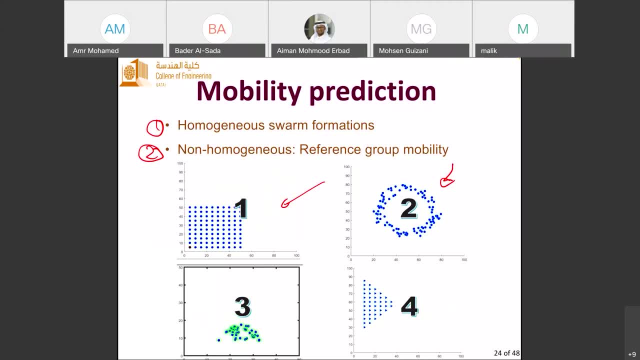 on the drones without having to worry so much on the- uh, the mobility patterns of these drones, because for homogeneous formations they are not the same as the other two drones. they don't change their positions in relation to each other. a lot other mobility patterns like they actually move in groups in such a way that, uh, they change their relative position. 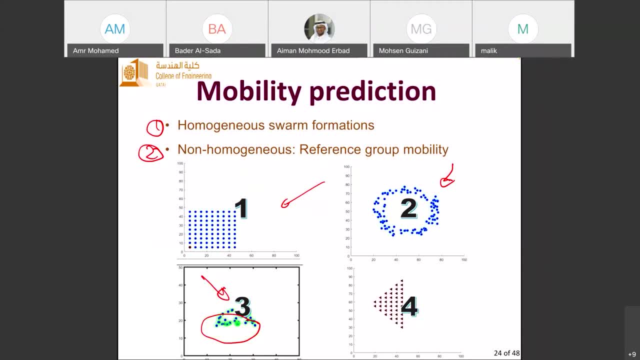 uh, with respect to each other a lot. however, because we are talking about swarm formation, they, they actually move in such a way that their position in relation to each other a lot in groups, they, they move in a group or two groups or something like that. so this type of challenging for the layer distribution and they require special 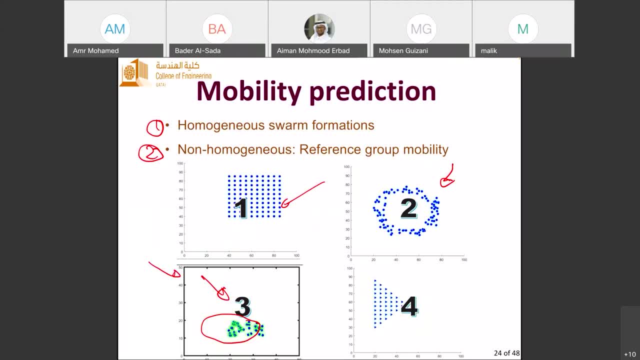 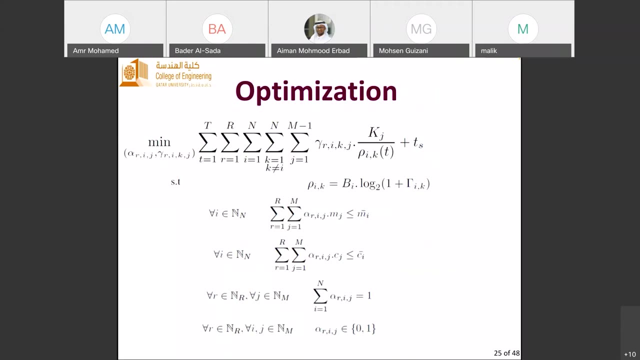 handling in terms of trying to predict the relative positions of the drones in the future in order to allocate or to distribute the layers right. so, in with that said, we try to again model this problem, but this time the objective itself changes significantly because, as you can see, here, there's no, as you can. 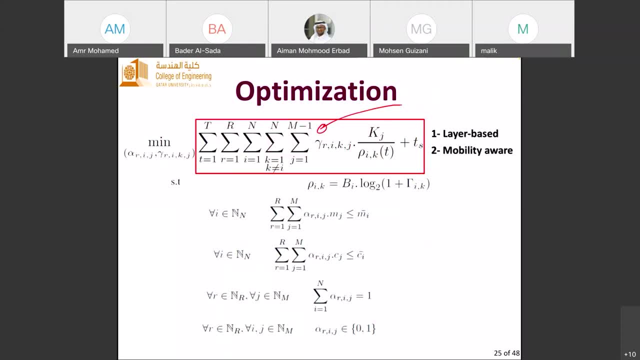 see there is no maximum because, again, it's not segment based, it's actually layer based. so we try to minimize the latency in terms of the time required to move the outcome of one layer to the next device, and we try to do that layer by layer. we try to find the best combinations of the drones on which we 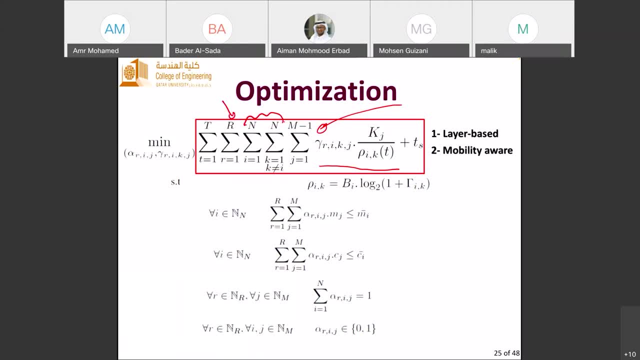 need to allocate these layers to a group of incoming requests are where ours is, from one to capital R, which are the total number of requests coming into the system, and maybe we can actually add to the top on Here. we do not have security constraints, of course. Security is not an issue in this. 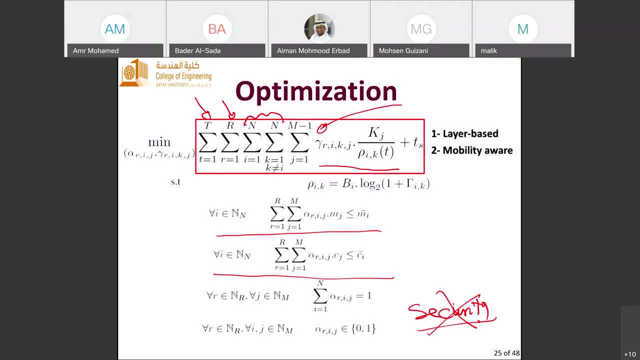 particular case. So therefore the layer-based distribution is possible. We tried to estimate the rate between each two drones based on a simple path loss model which takes into consideration the destination between the two drones, and the rate would be estimated based on that. So very quickly we see that for homogeneous 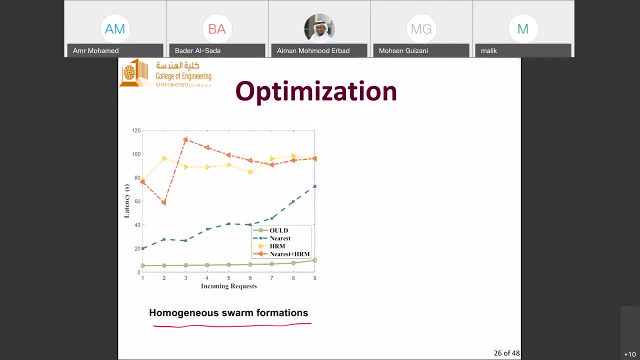 swarm formations. we don't really have to worry so much about the future time because the relative positions of the drones, as we have seen, is not significant and it does not change frequently. Okay, So here we have compared the optimal. so this is the optimal, green one is the optimal. 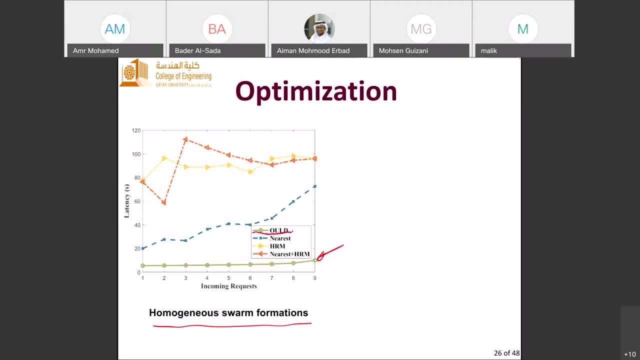 the solution to the optimal problem, to the optimization problem. and we have compared that with three other heuristics where we distribute the layer to the nearest drone in a greedy manner: Okay, So the next layer always goes to the nearest drone to me, okay, or the highest residual. 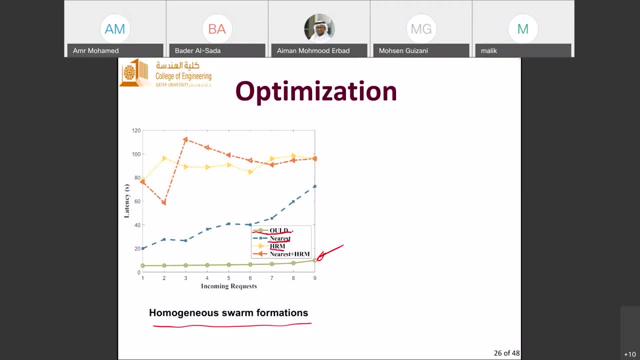 memory, or the drone with the highest remaining amount of memory, okay. or with a combination between the nearest and the highest residual memory in a trade-off manner, Okay. And as we can see for the for solving the optimization, it gives the best performance in terms of minimizing the latency and there. 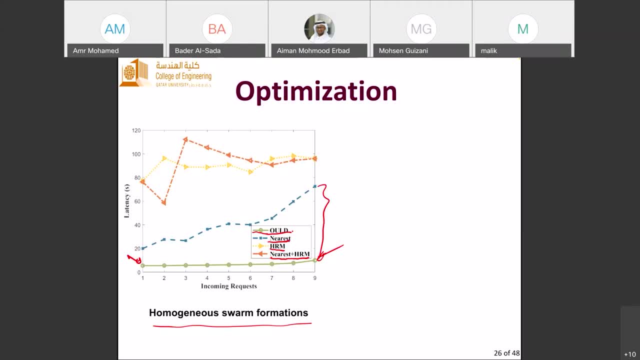 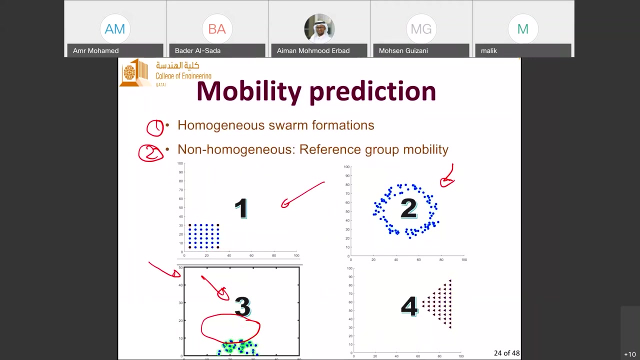 is a significant performance difference between the optimal solution and the nearest heuristic. Of course, this becomes even more challenging when the drones are mobile in a stochastic way, like using the- using this reference, a group model, lower number three. okay, so in that case, the relative positions of the drones. 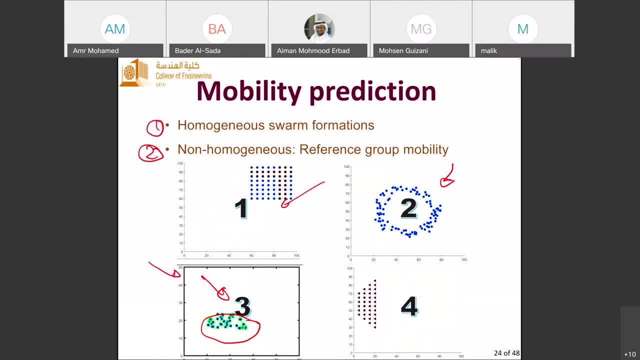 it changes a lot and in that case, the having a mobility prediction has to be part of the optimization problem in order to distribute the layers on strategic nodes that will not change the relative position to each other in the future. okay, so, uh, i have a question. yeah, go ahead. 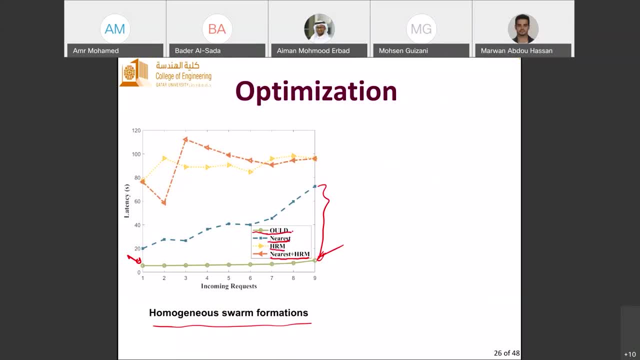 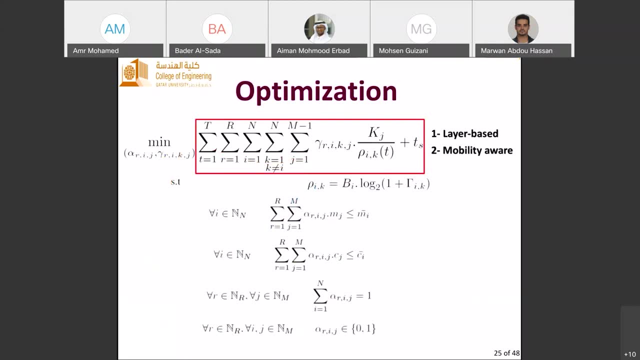 yes, uh, can you go back for one slide? it's a slide, the 25.. yes, you are. you are minimizing according to the number of requests. so the number of requests here is distributed in the system according to what, the what is this the scenario that you are following in the number of requests? 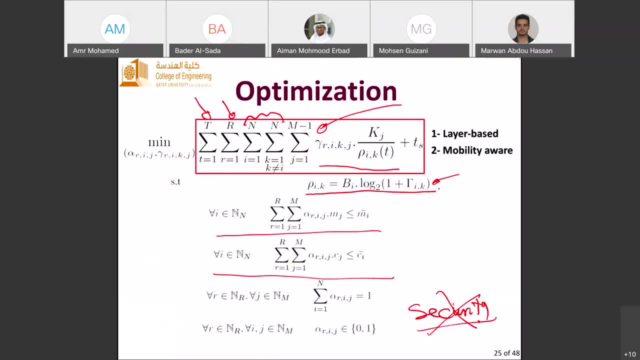 that you have. you have a set of incoming requests. the incoming request is defined by a request to perform an inference operation from the source mode. okay, all the way to the uh in system, which in that case it could be like the command and control system on the ground. 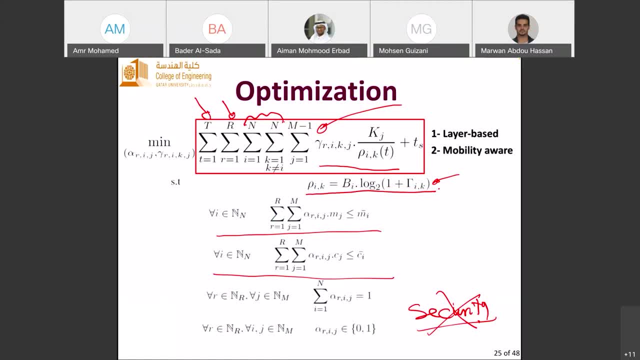 so you are- you are really trying to perceive a scene by the drones, okay, and you are trying to interpret what that theme is all about like, for example, uh, a set of uh intruding people to the borders. okay, so you are trying to detect using computer vision. 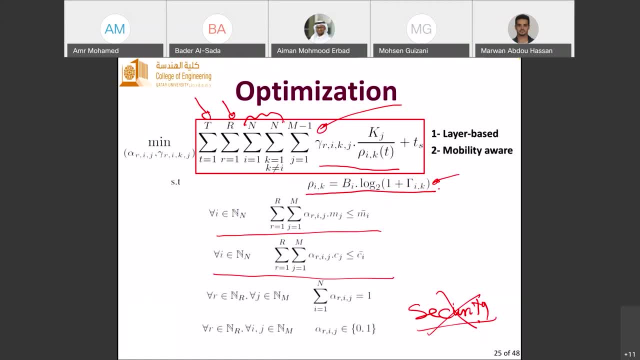 okay, so the machine learning model itself is is not of big concern to us, except that we need to distribute this machine learning model across the drones. okay, but the request is a request for detecting a specific scene context. okay, using this machine learning uh model. okay, i'm not sure. 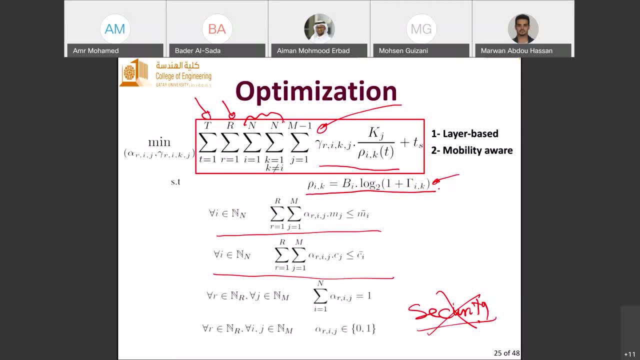 if that's uh, of the, if that's clear. so you have incoming requests to the system. each request represents a request to perform inference to a specific scene. context is that clear? yes, thank you. thank you so much. okay, but the the new aspect here, which has not been addressed at all in the previous. 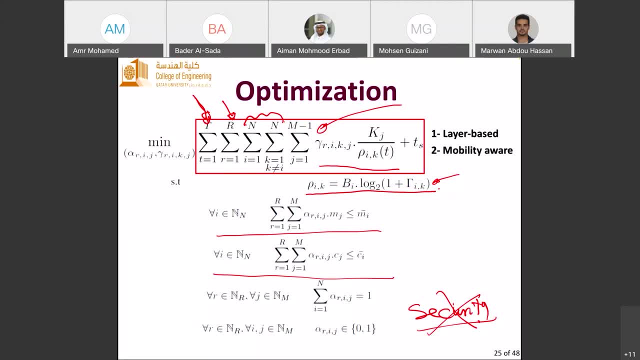 work is the time aspect, and the time aspect here is addressed because of the mobility nature of the uh of the drones. so we want to make sure that when we distribute these uh layers across the drones, that these drones will stay connected in the near future, at least for the next. 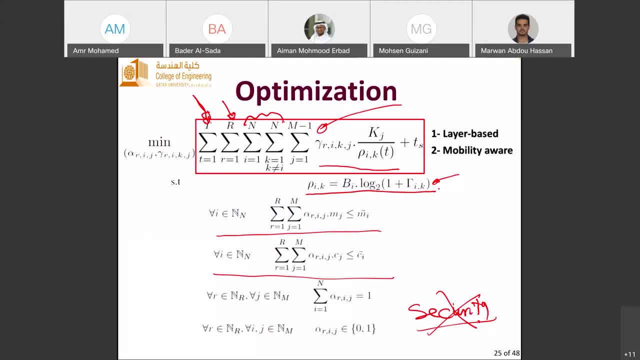 10 to 20 seconds or 30 seconds, they will still be in range to each other. okay, if, if the swarm formation is homogeneous, we don't have to worry about that, because the again the relative position between the drones, it does not change much, although the whole swarm formation it moves in a specific direction. 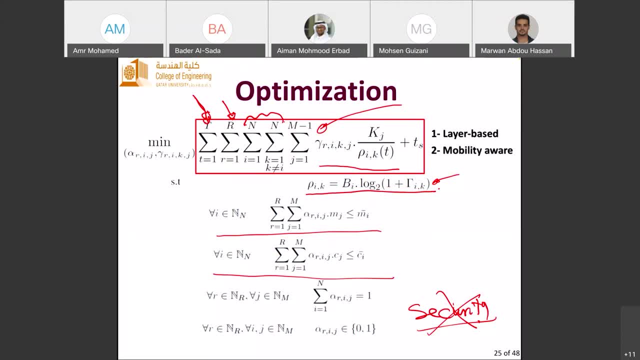 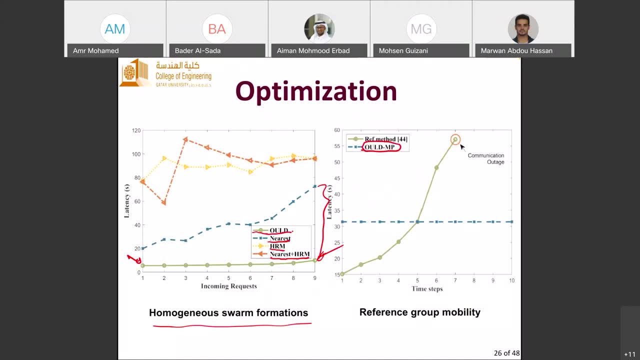 however, they don't change the relative position to each other. okay, so we have compared the same of these models and if the wild spores with the这个形状? um, the stanford question- uh, my name is bulan san- colors the relative location of the drones in the near future. 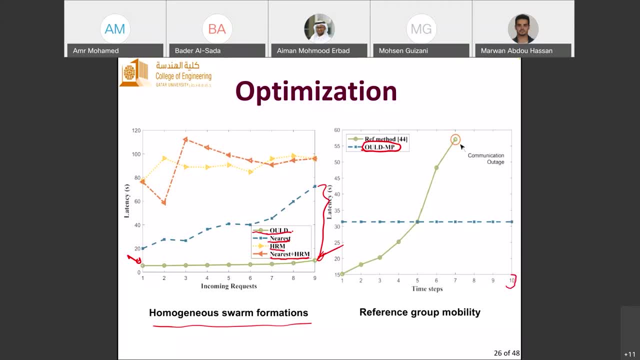 And we tried to do that for 10 future time steps. Okay, so at this point of time, we have performed mobility prediction. We knew the locations of the drones with respect to each other in the following 10 time steps And based on that, 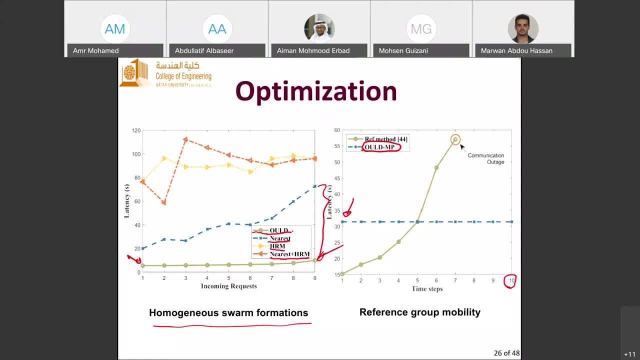 we have distributed the layers across the different drones, So that's why you see that the latency is almost fixed for the entire 10 time steps, because we know in the future that these drones will still be in communication with each other, Unlike another state of the art technique. 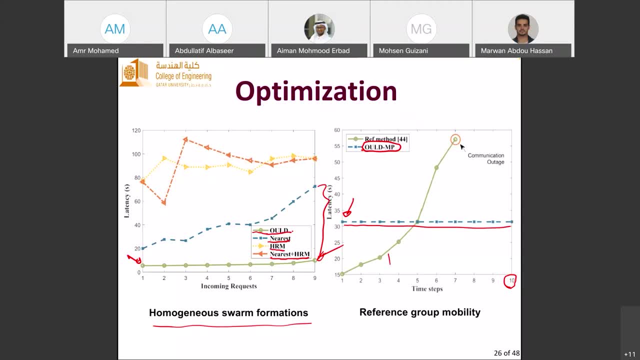 which is in the literature, that does not take into consideration the mobility prediction. So we see that the latency start to increase at some point. the drones, they become out of range from each other And in that case the communication is totally disconnected and the inference operation is totally halted. in that case, 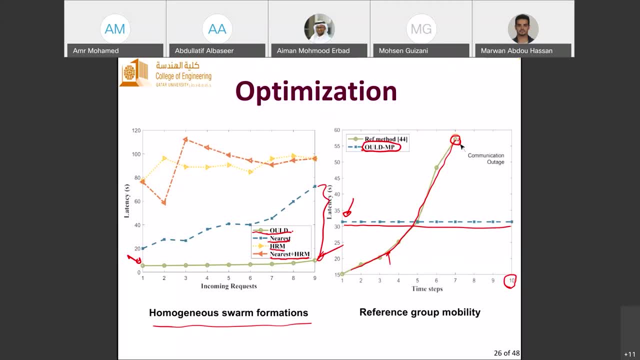 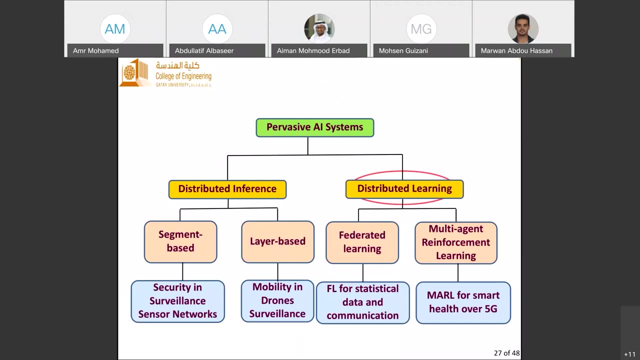 Okay, So that's the, again the distributed inference, And at this time we addressed the mobility aspect of the drones. So What about the performance with respect to the number of layers? That's a good question. This is done using homogeneous requests. 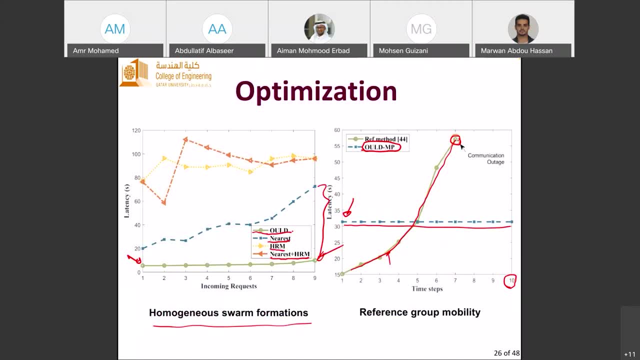 where we know beforehand that the request is a machine learning model using like, for example, Linet or VGG16 or something like this. Okay, So, regardless of the number of layers, as long as we have enough drones with enough computation and memory capability. 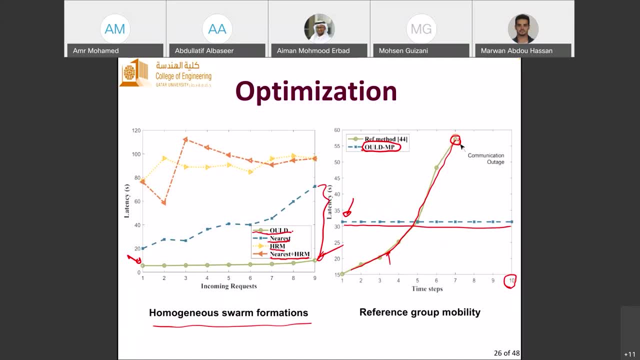 to handle the layers in the machine learning model. that's what this distribution algorithm is all about. So the number of layers will affect again the number of drones needed to accommodate these layers. Also, the latency will be affected by this. Okay, 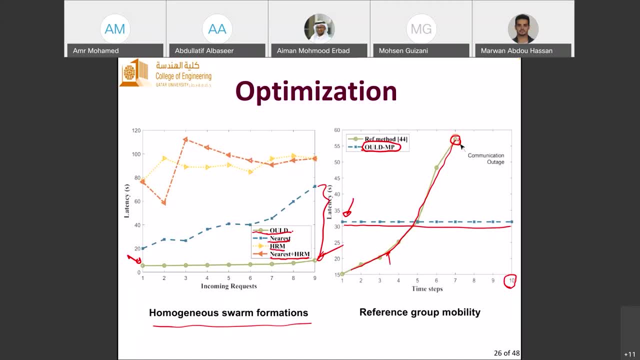 Also, the latency will be affected by this. Also, the latency will be affected by the number of layers. Yes, yes, you are right. You are right. In the paper, by the way, there is, yes, there is- some result to estimate the latency. 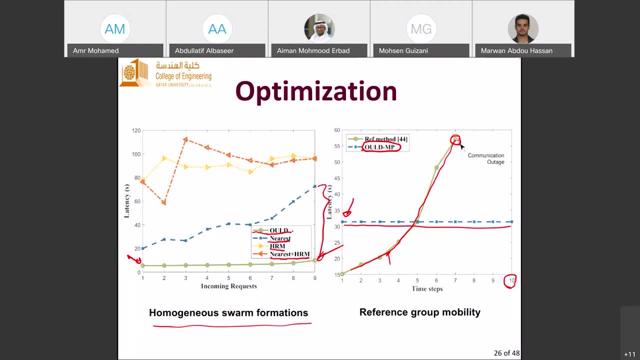 as a function of the number of drones. You are perfectly right. So, and you are perfectly right that as we have more and more drones, the latency should be reduced, particularly the number of rejected requests, and the number of requests will be reduced okay. 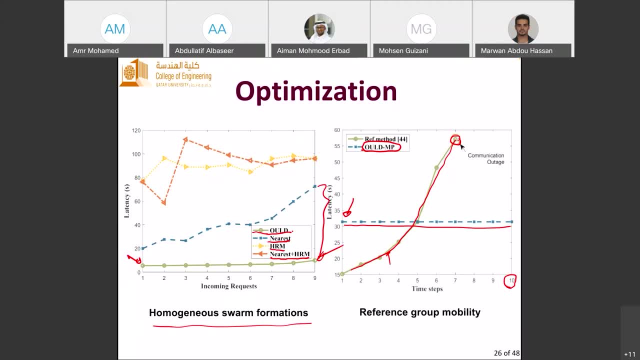 More importantly, the number of accommodated requests should be more as the number of drones grow, more right, And if you have less number of drones, then the degrees of freedom that you have is less, and in which case, at some point, 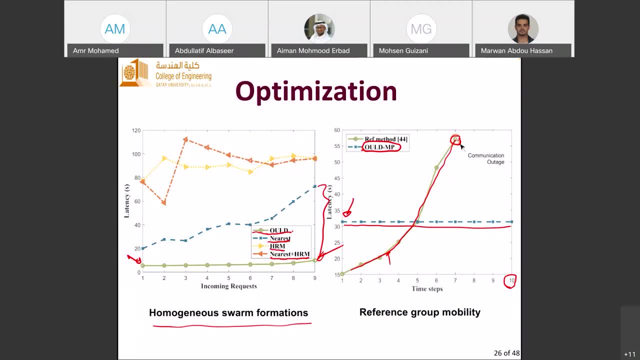 you might have to reject many requests, many incoming requests you have to reject because you do not have enough drones to handle this. Okay, Yes, We can have adaptive structure for the number of or compared to the number of drones available. Yes, so, yes, so the if you want to change the optimization problem. 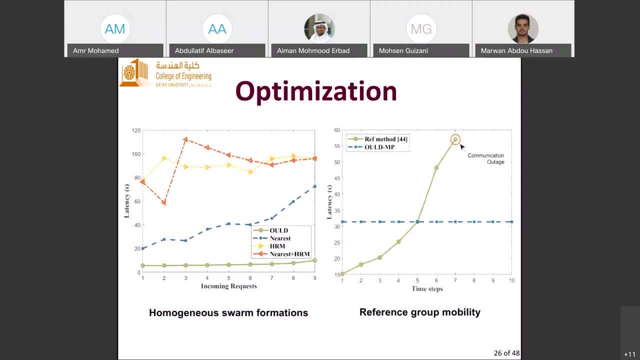 instead of minimizing the latency, you could actually minimize the number of drones engaged in the inference operation. Yes, That's a different objective. Okay, Thank you, That's a different objective in that case. okay, So currently the objective is to try. 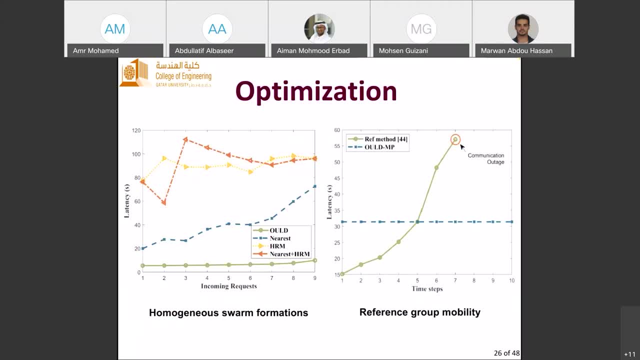 to minimize the end-to-end latency for the inference operation and the layers are allocated such that we meet the computation and memory constraints on each drone. But if you want to minimize the number of drones engaged, that's a totally different objective, okay. 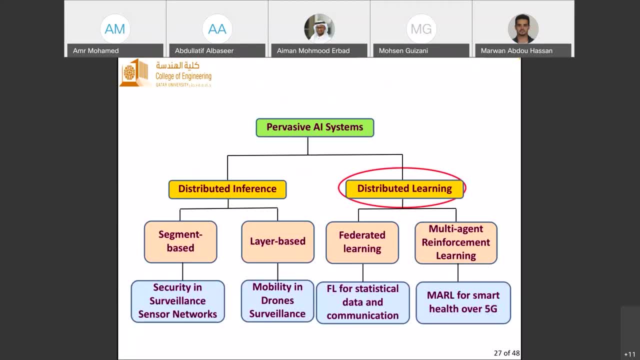 Thank you. So the mobility part was maybe a little bit less comprehensive because we are still working on that, By the way. another approach to address the mobility, because it's another stochastic dimension for the network dynamics. So another approach, as you can imagine. 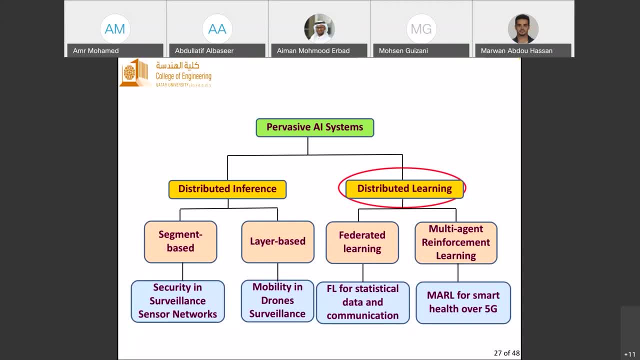 to solve the same optimization problem is using reinforcement learning, So that's a different topic. So that's what we are trying to do now And really designing the reinforcement learning agent to learn the mobility pattern of the drones automatically is a very interesting piece. 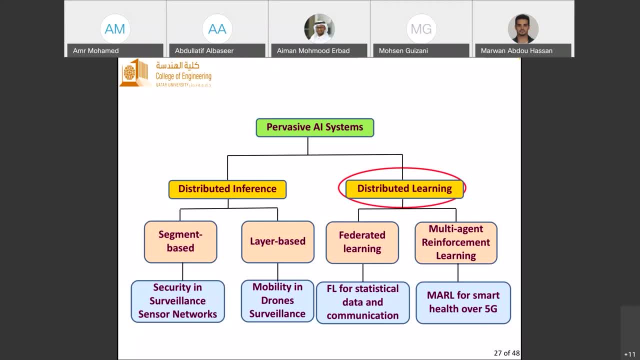 of work that we are currently trying to work on. Okay, So, Dr Ayman, what do you suggest? Should we move on Or should we stop at this point? It's up to you. No, no, continue, continue. 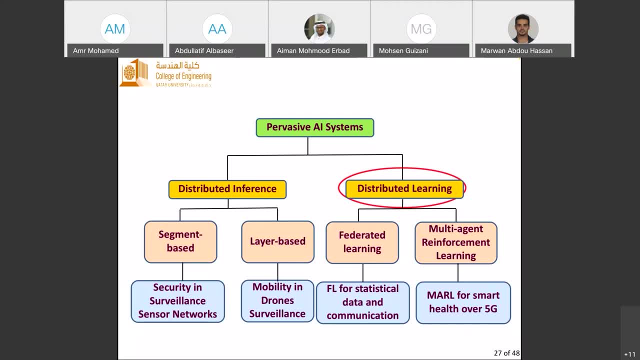 I think you are picking up the speed. Yes, continue, continue, doctor Interesting, Okay. So the distributed learning part: here, the machine learning model is not even trained, okay, And we are trying to learn in real time in a distributed way. 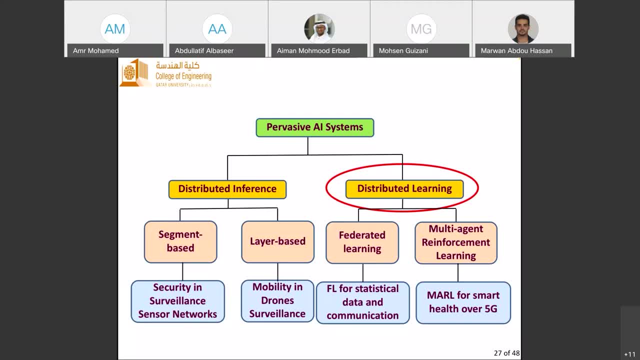 And here, as I said before, this branch is quite intensively addressed in the literature In two sub areas, including learning, where the machine learning model has some weights that change over time, And we are trying to calculate the weights in a distributed way, as we will see. 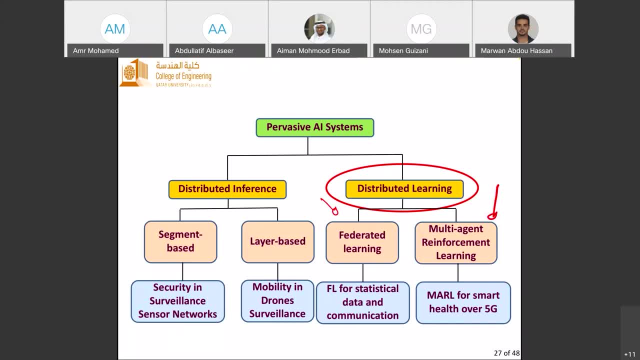 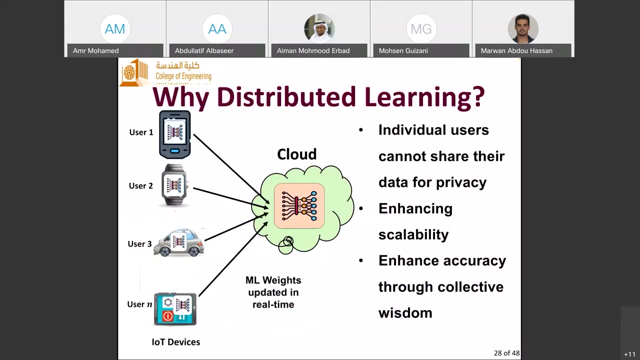 And the other branch here is multiagent reinforcement learning. So, unlike the single agent, we can deploy agent in a agents in distributed manner to perform some, some distributed optimization, as we will see next. Okay, So what is the motivation? What is the motivation behind distributed learning? 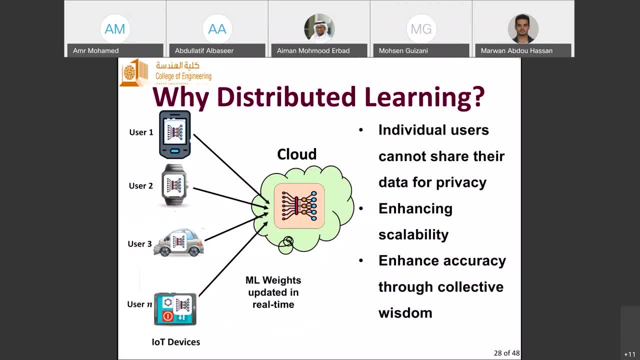 So why not send all the data from the IoT devices or from the devices themselves, send these data to the cloud and, in the cloud, perform the training? Okay, And that's it. So why not do that? Why we shouldn't do that? 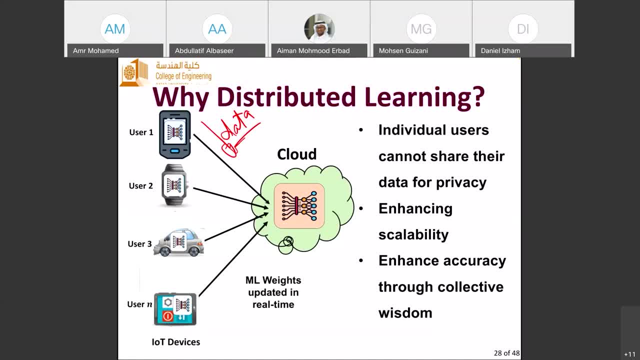 We shouldn't do that because in many application, individual users cannot share their private data. They cannot, Okay, So their data cannot be shared with the cloud, So they cannot send the data to the cloud exposed, because this will have some privacy issues, Also due to some scalability, as we have seen before. 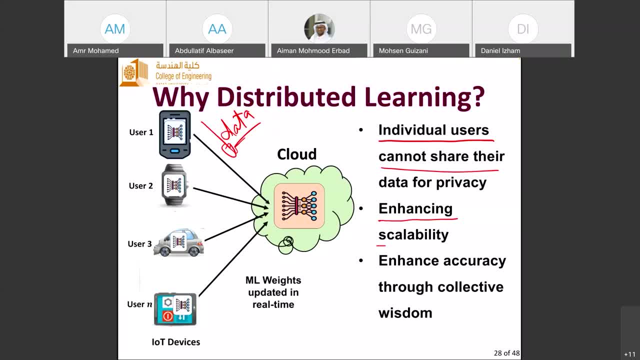 and I have explained this in the motivation part- that this will have an effect on the scalability by having massive data streams between the IoT devices and the cloud, And in that case, scalability would be an issue. Instead, what they try to do is that. 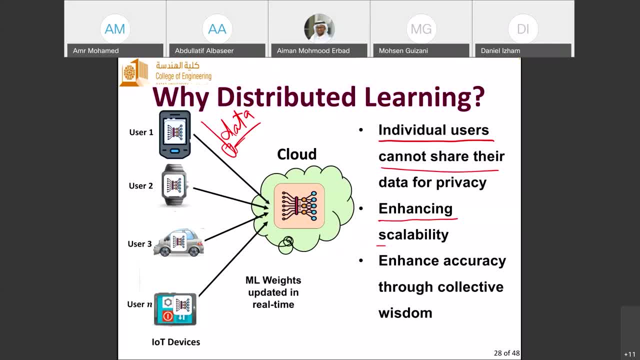 they don't actually send data. They send model hypercars, Okay, Hyperparameters. They send the machine learning model hyperparameters as opposed to the actual data. So in that case there is no privacy issue And the distributed learning here tries to enhance. 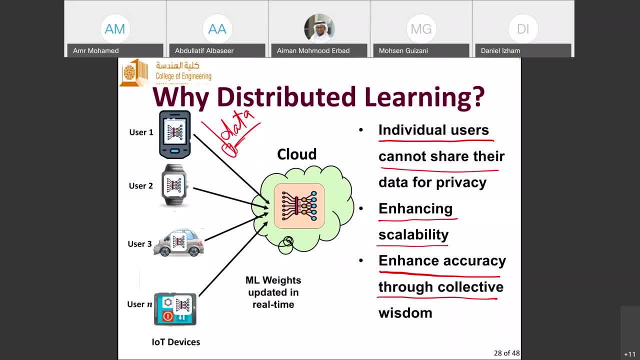 and maximize the accuracy through some collective wisdom. So here we are trying to learn from massive number of users Like, for example, I can tell you an application like we are trying to detect a pandemic like COVID-19.. So we are trying to do this through data. 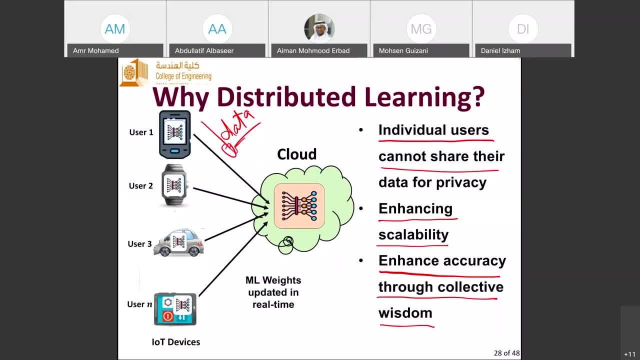 from the different users right. So one way is to get the data from all the users and then perform all the prediction at the cloud, which will have some privacy issues, Although in some cases, privacy issue privacy issues might be breached. 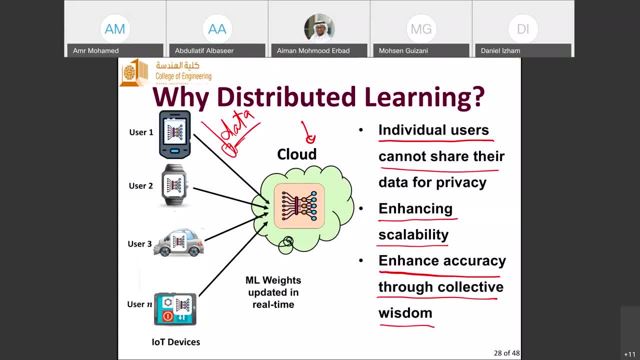 But, in other words, the privacy is in some cases, very important And we are trying to learn or predict this pandemic through massive data coming from hundreds or thousands of users in the country. Okay, So in that case, instead of sharing the data, 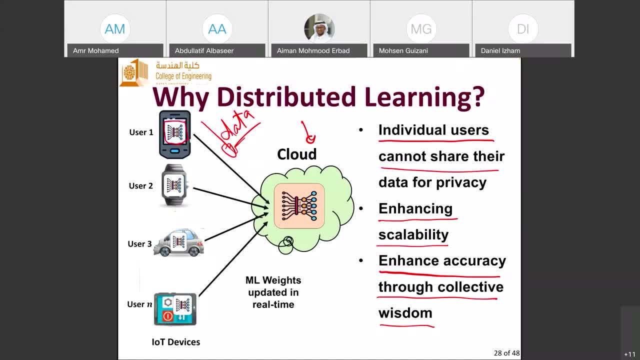 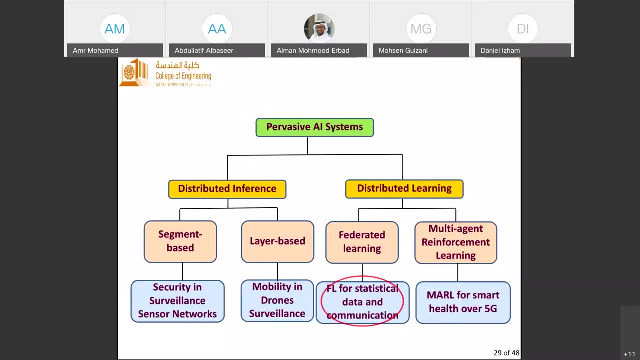 we have prediction model deployed. we have prediction model deployed on the user level. Okay, And instead of exchanging data, we exchange model hyperparameters. So, more specifically, so for federated learning, for example, the idea is as follows: So the individual devices will receive data. 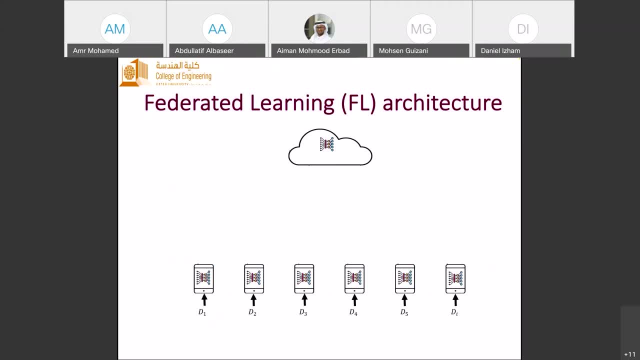 or will use specific data nature. so, of course, the the data experienced by individual users are inherently and statistically different. okay, and then this data can be used at every single device and we can perform weight updates. so for machine learning, we have, we know that we have weights and biases and these are: 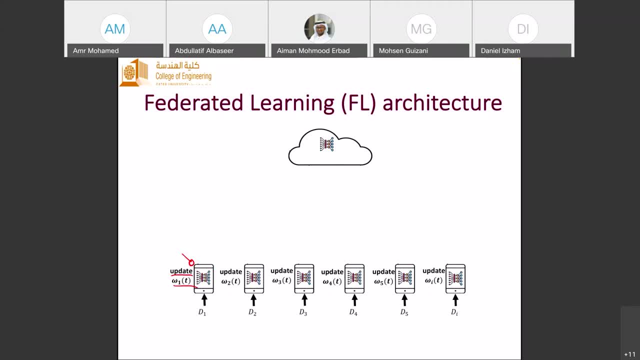 the uh, the parameters that can be iteratively estimated at each device level and after certain amount of iterations or episodes we actually perform, we actually send the weights themselves okay to the clouds. so this is not the actual data. in that case, it's the weights okay, uh, and at the cloud level. 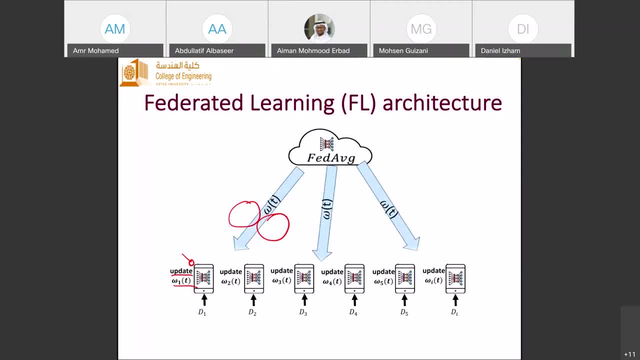 what we do is that we use a very well established uh theory which is called federated average. so we perform, basically, uh estimation for weights at the cloud level, which is the average of the weights provided by each user. okay, and then, after estimating this federated, we send it, we send the. 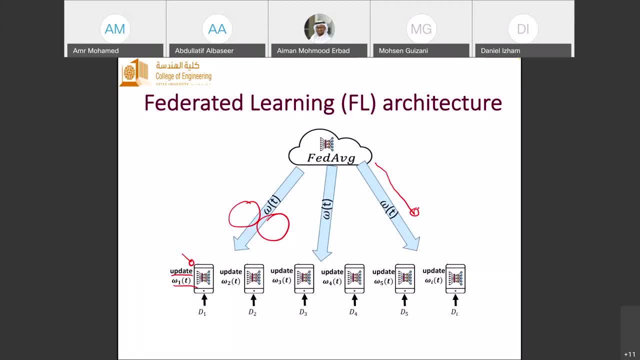 weights back to the individual users and, supposedly, by doing this iteratively and uh uh in a cyclic manner, uh over time, we, uh uh, we do the learning in a in a more efficient way and the model accuracy will be enhanced through uh gathering or collectively understanding the. 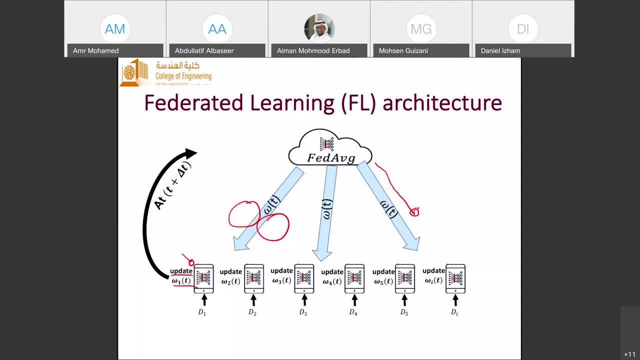 statistical aspects of the data from hundreds of users, so what we call the collective wisdom. so learning through collective wisdom, okay, and then we do that in a cyclic manner, and then we do the learning in a more efficient way, and then we do the learning in a more efficient way, and then we do the learning in a more efficient way. 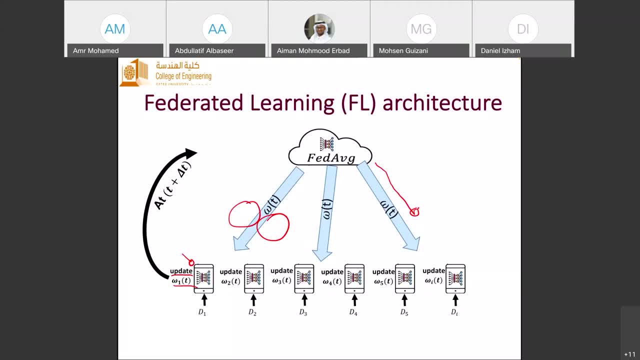 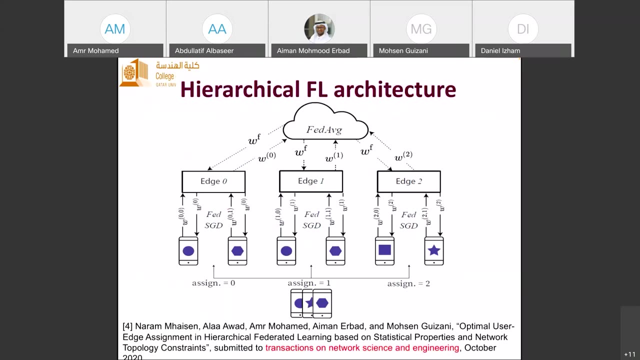 so over time we should converge uh, uh, uh in such a way that we maximize the uh, the accuracy of the entire machine learning model. okay, so the learning process in that case is done iteratively and in real time. so the state of the art when it comes to federated learning is what we call hierarchical. 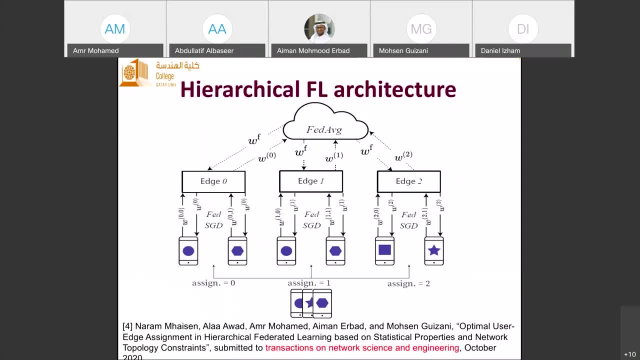 federated learning. so for hierarchical federated learning we did. we have edge nodes which are close to the uh, to the devices, okay, and and then we perform the same learning operation in a hierarchical manner. so first we perform an iterative estimation of the weights at the device. 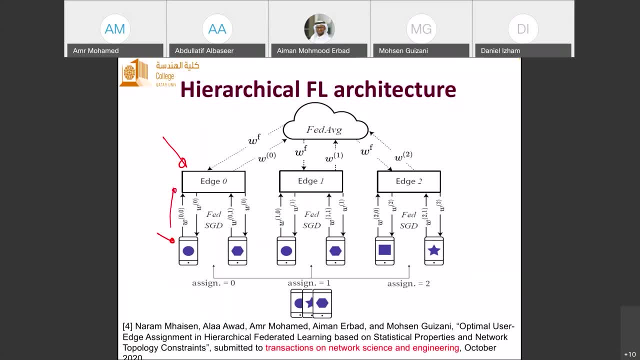 level. we send this weight to the edge first, and then the edge would perform a federated average step- okay, and then this edge would perform a federated average step- okay, and then this edge will uh, then send the uh average weights to the cloud, which again it performs another level of. 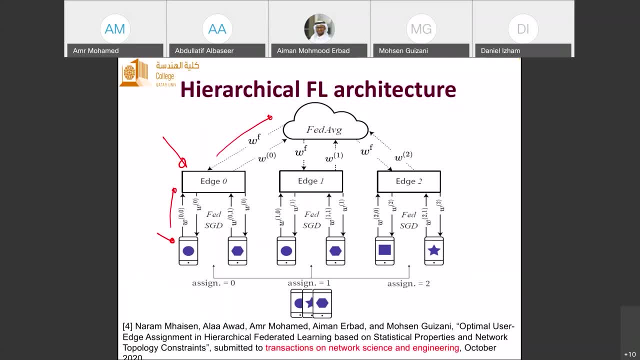 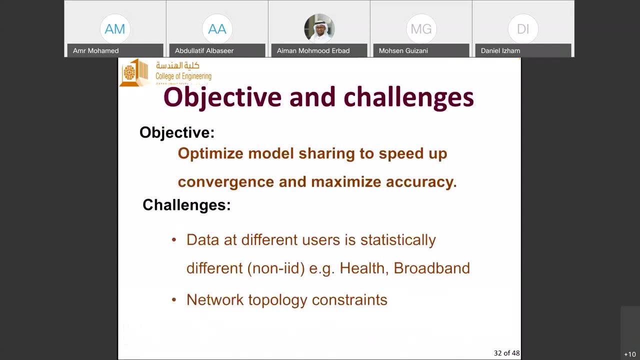 federated average. okay, so in that case we perform hierarchical federated average steps. okay, so this will see the benefit of this hierarchical federated learning architecture in a minute. so the objective in that case is to try to optimize the, the model sharing of uh, of weights, okay, between the uh, the iot devices and the edge. okay, to try to, on one hand. 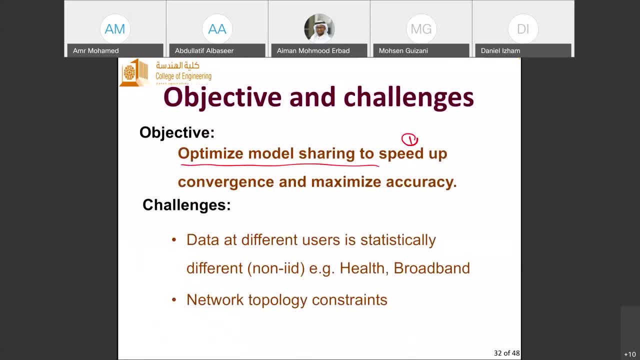 speed up the conversions and, on another hand, maximize the accuracy. okay, so we try to speed up the conversions and maximize the accuracy at the same time. okay, through the concept of, as i said, collective wisdom. and the challenge here is that that that data at the different user level is statistically different. so, for example, for example, if i want to, 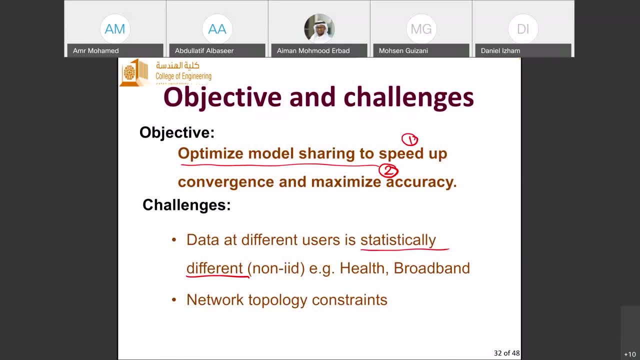 detect a certain health health related disorder. okay, i'm trying to deploy a machine learning model that remotely detects a certain health disorder like, for example, heart attack or a seizure, a patient who is having seizure, or something like this. okay, so in that case, i would not expect a single user to have data enough to detect all the 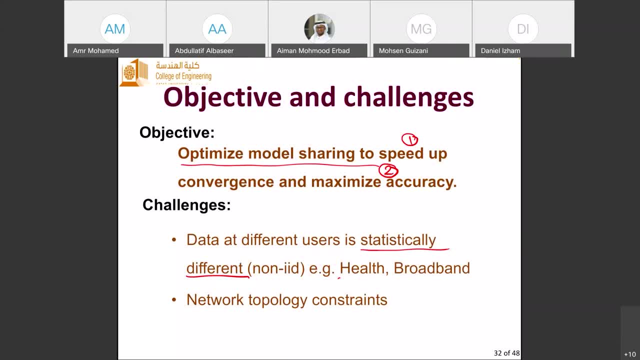 different classes. okay, the classes here being, for example, the severity of the heart attack, or the severity of the seizure, or the location of the seizure, and so on. so in general, you have multiple classes, like, let's say, like 10 different classes, and i'm not expecting each individual user to have 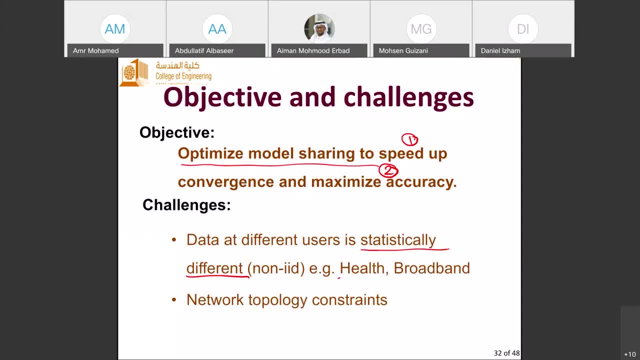 all the 10 classes, of course. naturally we have a certain type of disorder. each user will have one or two maximum types of this order. another application where, again, like for example orido, they are trying to detect the type of traffic okay from different users in order to enhance their broadband service. so again, i'm not. 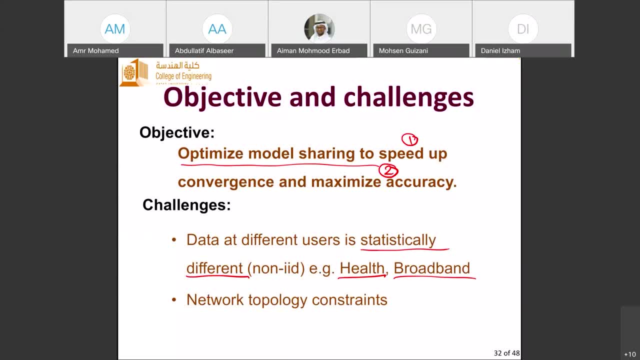 expecting a single user to to, to, to do all the different services at all times. so i'm expecting, for example, certain types of users: they do gaming more than watching tv. other users: they do- they do watch tv more than browsing the internet, or something like this. okay, 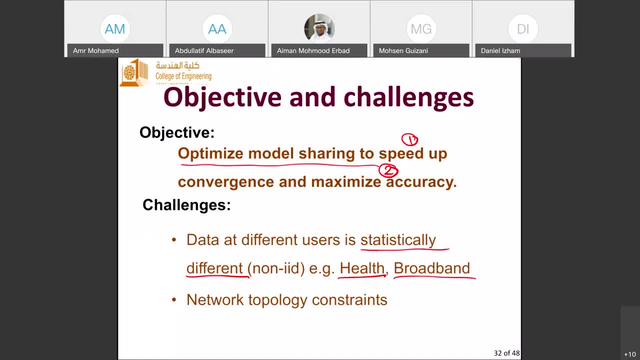 so in that case, uh, the, the, the, the different data that exists at different users is statistically different, so we call it non-iid, we call this type of data set non-iid, which stands for non-identical, and uh, uh, uh, statistic is statistically different data, okay. 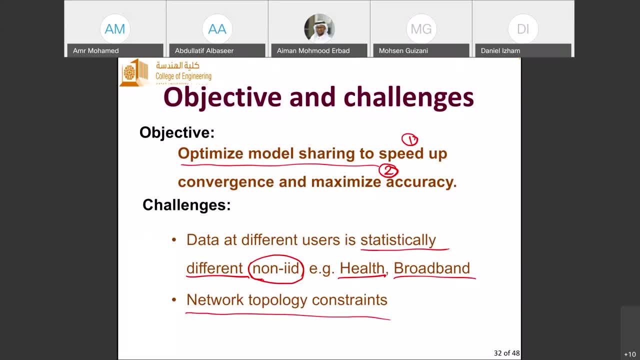 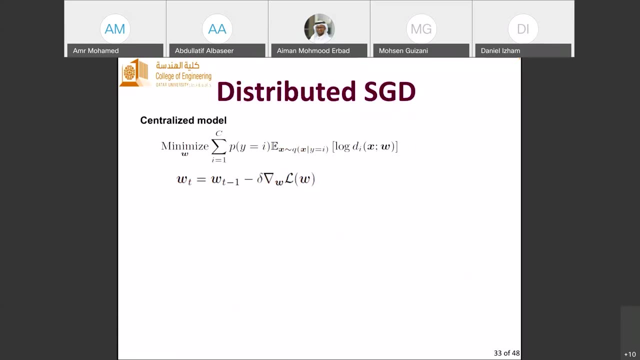 and again, we have to take into consideration the topology constraints of the network. so, for example, not every node would have access to all the edges, so i need to take into consideration some network topology constraints. all right, so in order to perform this federated learning in a distributed manner, we know that the centralized model simply tries to minimize 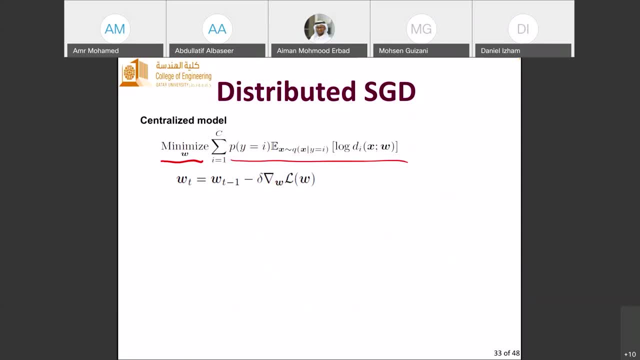 a loss function and this loss function is based on the cross entropy. so the, the people from machine learning, they would know this loss function, the, the cross entropy, and we are trying to estimate the weight, uh, the weights, based on negative, the, the gradient, okay, and of course they use the 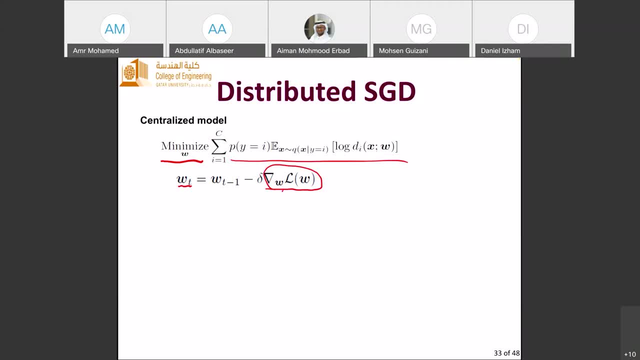 stochastic gradient descent, in that case to avoid, you know, having to estimate the gradient based on the whole data set. uh, so these weights are estimated iteratively, but this model assumes that all the data set exists in the cloud, which is not possible in our case because the data is 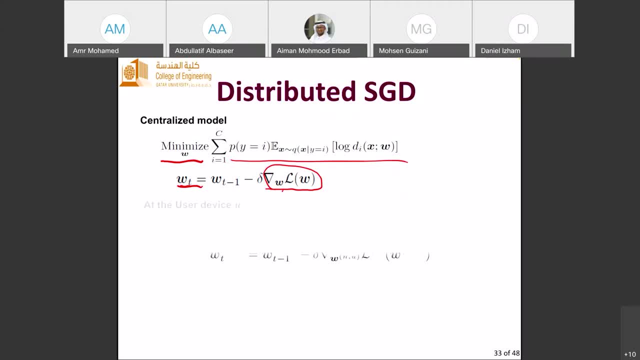 at the different users, right. so instead, what we what we need to do is that, at the user device level, we need to estimate, okay, the local weights. the local weights which is based on a specific edge and a specific user. okay, based on the local gradient descent, based on part of the data set. 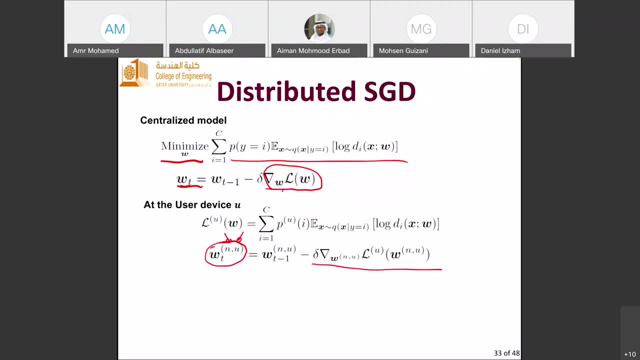 that exists at at this user, okay. and then this: these weights can be averaged using the, again the federated average, at two steps. the first step: after t dash iterations, we perform the federated average at the edge level, at each edge- okay. and then from the m edges: okay, we perform another federated average stage. 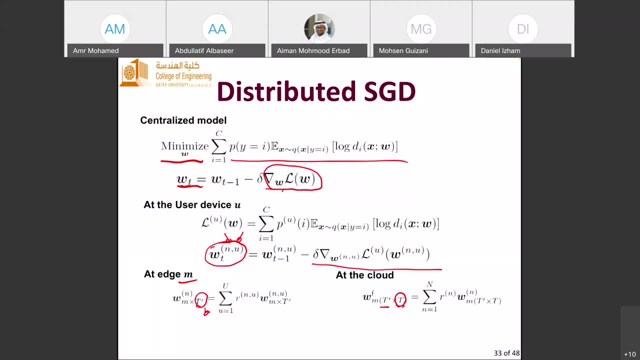 at the cloud level. so after t dash steps, we do at the edge, and after t dash, after t other steps, we do the federated average at the cloud. okay, so that's so. the idea here is that this is the distributed weights. okay, so these are the distributed weights of the model. 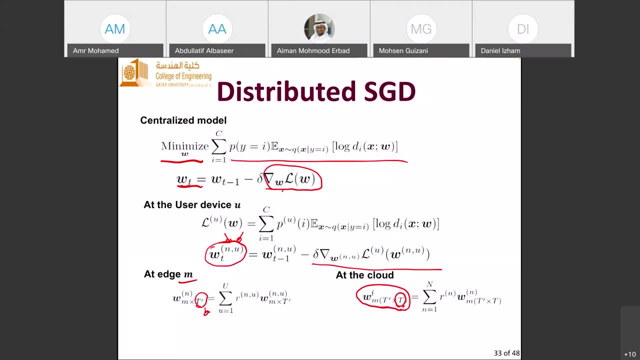 given the federated learning paradigm that we just explained, this is the centralized weights. okay, so the idea now is to minimize, is to try to minimize the magn, the magnitude of the difference between the federated weights and the uh and the centralized weights, and this is what we call the uh, the divergence factor. okay, so the divergence factor. 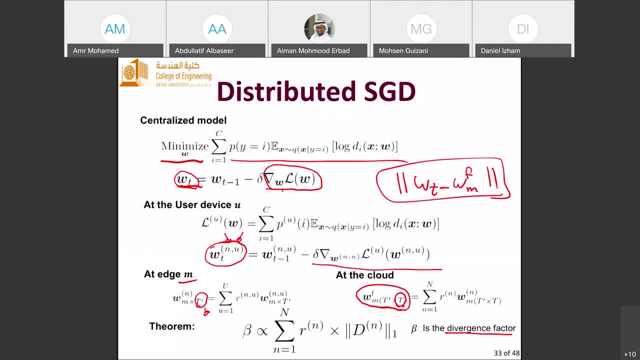 is in fact the difference, or the magnitude difference, between the centralized weights and the federated weights. all right, so in the paper we we actually go- i mean, uh, the researcher- intensively in the calculation to try to prove that this divergence factor is indeed proportional to the, uh, the proportion of the data at each. 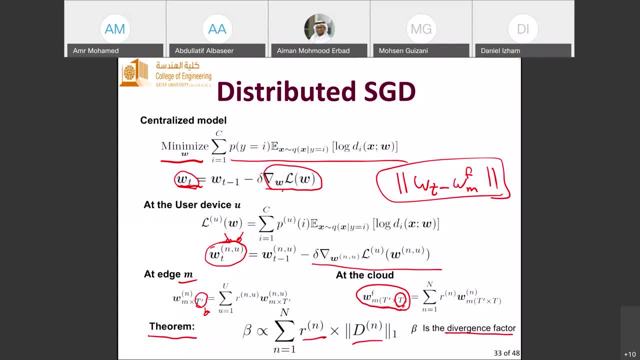 edge node and the distribution of the data at each node. okay, which is a multiplication of those two components, the proportion of the data. so how much of the data set exists at each edge node and what is the distribution of this data? and again, someone might ask if you know the distribution. 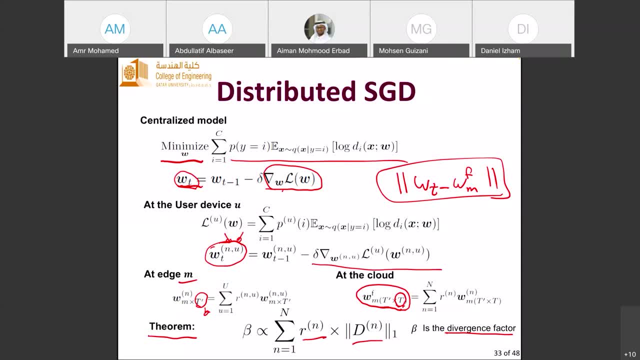 you know the data and the answer is no. that just the fact that you know the distribution of the data. it doesn't mean that you know the actual data itself. okay, so uh, by distribution here i mean how much time this edge sees that the person is having seizure, for example, or having a heart attack. 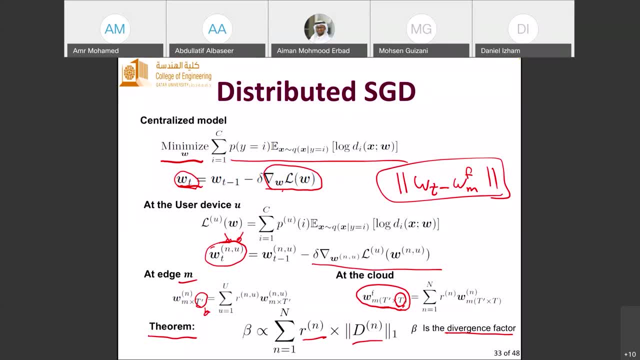 but i didn't know exactly who, who is the person who is having seizure and at what time, and so on and so forth. so knowing the distribution is actually a prerequisite to perform this minimization for the diversion, the divergence factor. so in this work, the, the parameter that we have taken in order to minimize this divergence factor was how to assign. 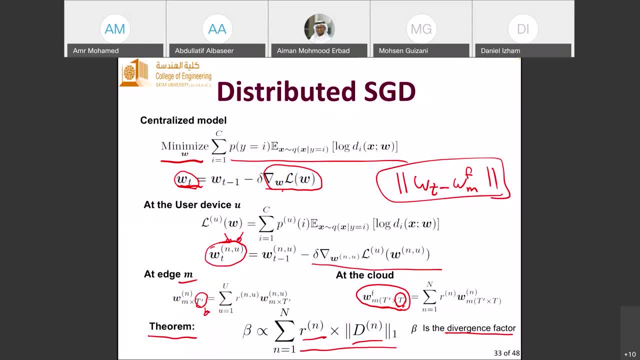 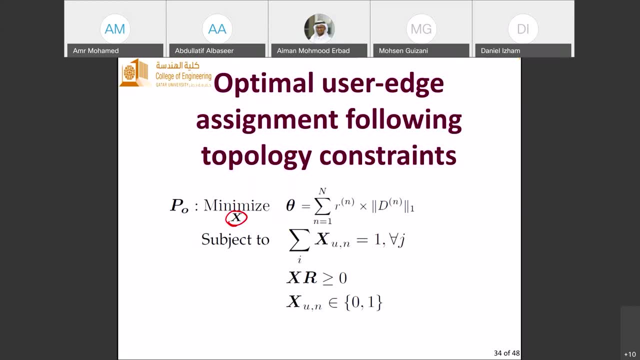 the individual devices to particular edges. okay, so this x, uh, here is the decision variable which, which really represents which device should be attached to which edge node in such a way that minimizes this a, this divergence factor. okay, so this optimization problem is a non-linear integer program in nature because, uh, both the, both the r. 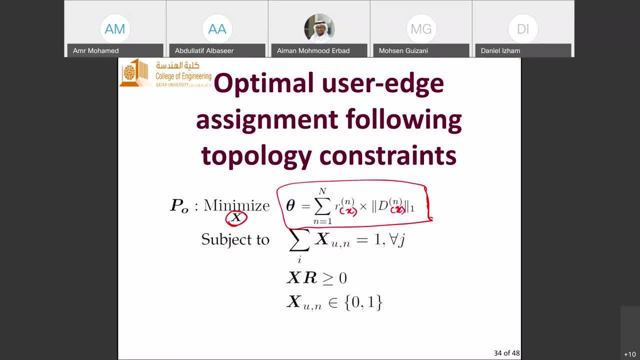 and the d are actually function of x. okay, which makes this problem non-linear: integer, uh, program in nature and uh, of course, we have another constraint here, which is the uh, the topology constraint. so which node can reach, so how how many? so, for example, one node has access to how many edges? so if, if, if, all nodes. 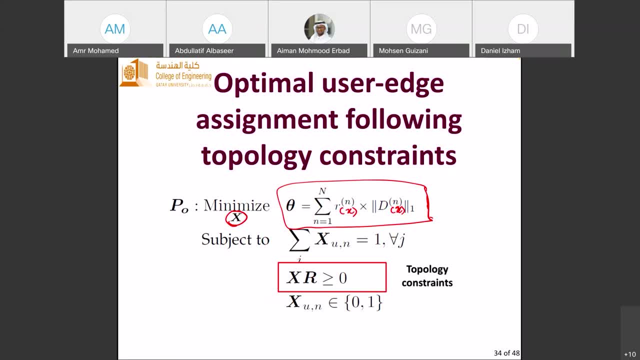 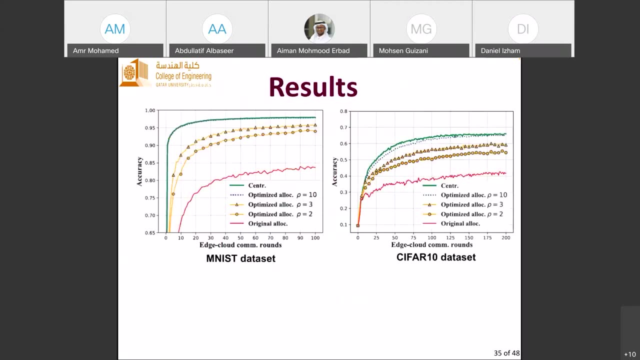 have access to all edges, then you have very high degree of freedom and you can assign the node to the edge that gives you the minimum divergence factor. in that case, okay, uh, so that's the, that's the problem and the uh. the results here show that, uh, uh indeed. 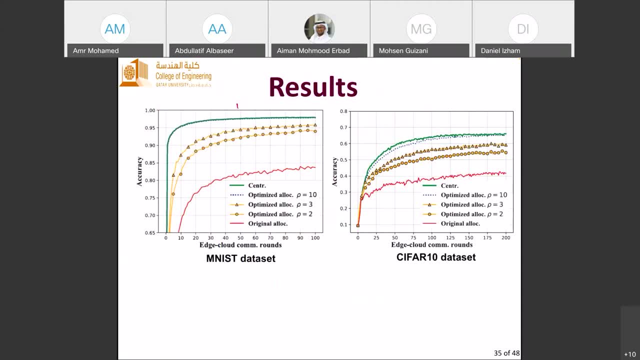 the uh, the optimization. so so the green, the green curve here is for the centralized weights, where the data set exists, uh, totally in the cloud and we perform the uh, the, the weight estimation on the cloud only, okay, whereas the uh, the yellow curves here they uh, uh, represent the estimated 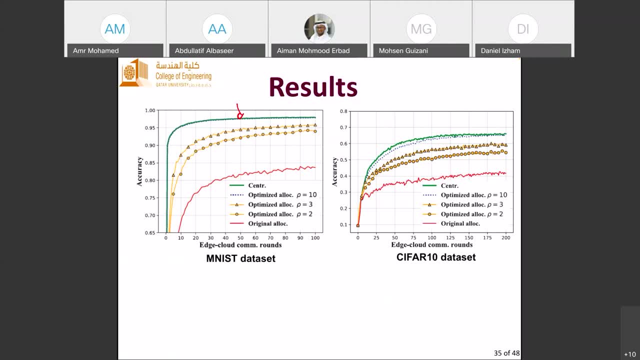 uh accuracy and the conversions of the loss function okay, by assigning the, the devices to the edges in a strategic way, in such a way that tries to again minimize this divergence factor and, as course, on different data sets- the MNEST and the CIFAR data sets- and we can see significant 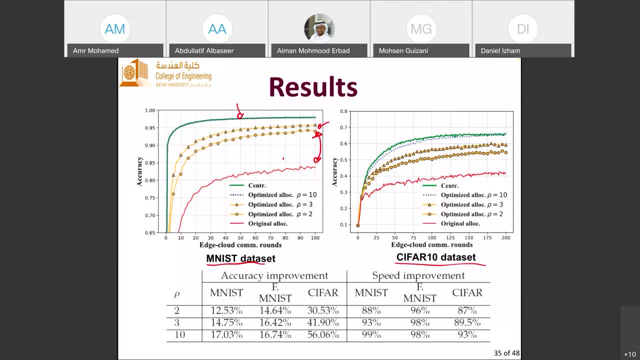 performance enhancement- okay, based on formal federated learning. So this red, this curve here is the non-hierarchical case where the weights are learned based on the current distribution of data at the device, without having to have edges that participate in the hierarchical. 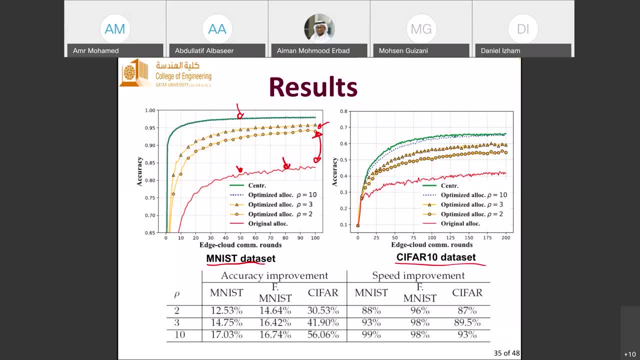 federated learning. So in that case, the performance enhancement using the hierarchical federated learning is not only significant in terms of enhancing the security- sorry, enhancing the accuracy- but also significant in terms of speed, So we can reach to the same. 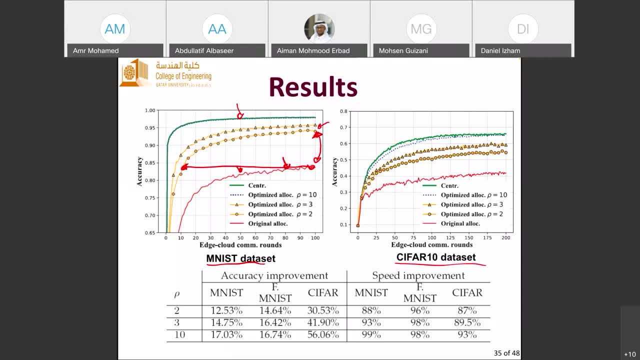 accuracy, We can reach to the same level much, much, much faster, okay, So here we have to have like almost 100 rounds of exchange of weights between the edge and the clouds, okay, in order to reach to an accuracy level of close to 84%, okay, which, in that case, is reached using the optimal. 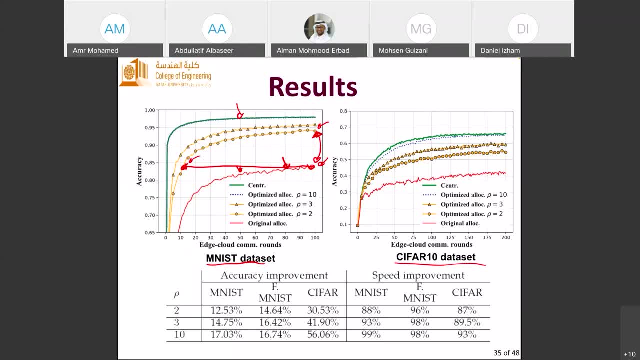 allocation at only like 10 different or 12 different communities. So in that case, this table here shows the performance enhancement in terms of accuracy and speed. okay, As we increase rho and rho- here it means the number of edges that each 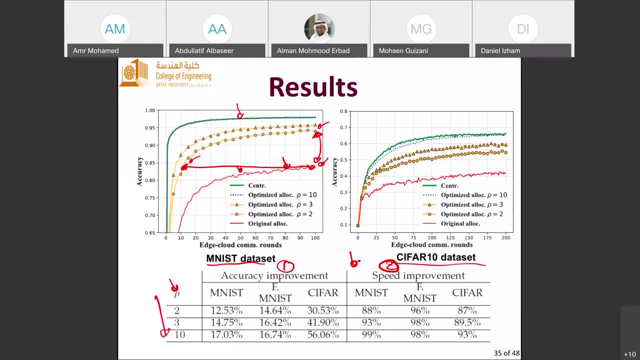 node has access to. So as we increase rho, this means that we don't have any topology constraints, which means that the each node has access to as many edges as it wants. So in that case, we assign the node to the edges strategically in order to improve or to optimize. 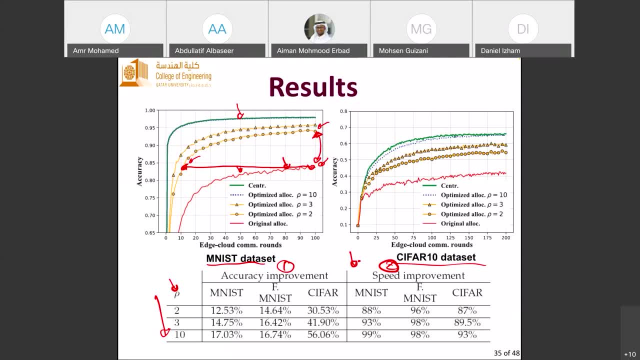 the speed and the accuracy levels. okay, So this is the federated learning part, and here we have tried to conduct hierarchical federated learning. okay, by understanding the statistical differences between various types of edges that the local data sets that exist at different user, and then by assigning these users to 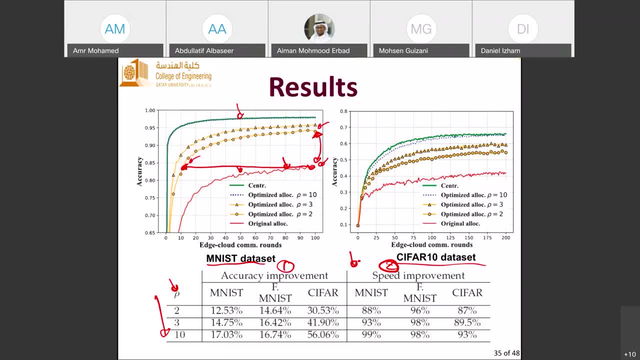 strategic edges. we were able to enhance the conversions performance significantly using the hierarchical federated learning. so before we move to the next part, let's just take some questions. uh, for this part. okay, my stuff, what, okay? thank you, professor uh, for this valuable explanation. i have just a question for uh. please can you go for uh or two uh problem. 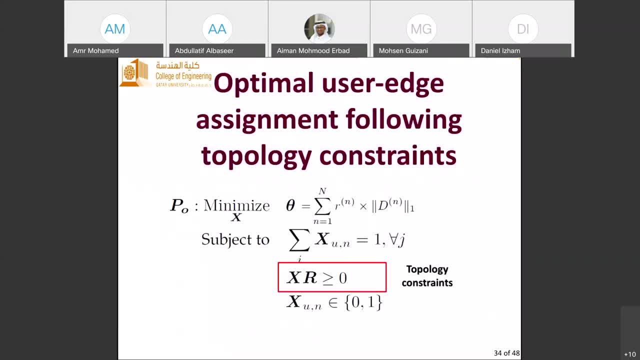 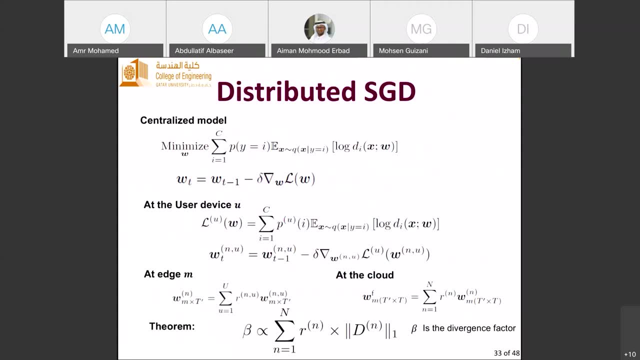 formulation: uh, the optimization problem. this one, no, no, the previous slide is this one. yes, for the cross entropy. i think the formula has a negative sign at the beginning. the one which one? uh, for the formula of cross entropy: yes, this is the loss function. yes, okay, there's a moment. so if there is a minus here before this, yes, yes, could be. 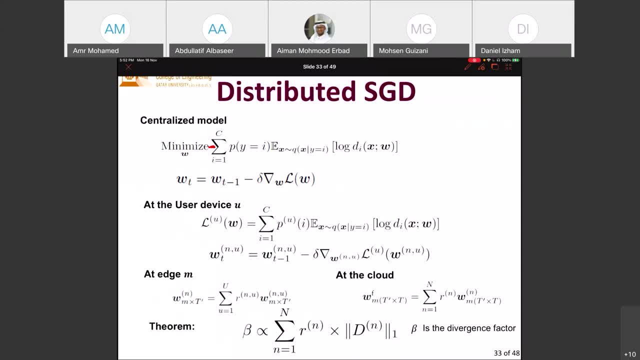 could be. i have to double check, but uh, i think the cross entropy it could be, i don't know. okay, so we can, we can double check that, okay, uh. the second question: how to group the users or how to assign the users to the edge. uh, should the users uh exibilist or uh this? 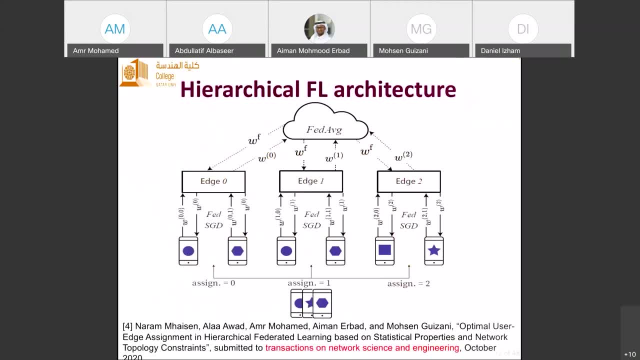 their classes. oh yes, uh, that's a that's a good question, uh, so, um, so here this is. this is the actual system model, right? so the idea here is that each, each device has part of the data set. okay, okay, so this data set okay at device i. 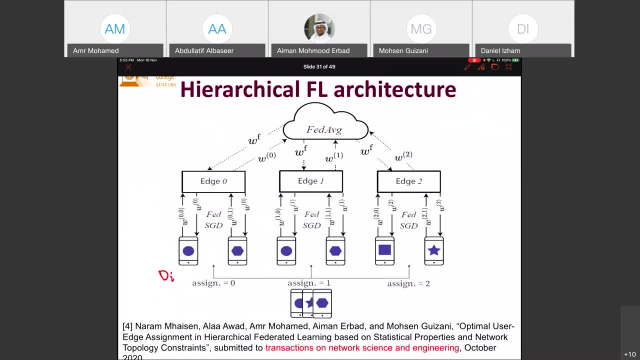 we need to know the distribution of this data set. we need to know the distribution, not the actual data set. remember, we need to know the distribution, which means that how much time this user, for example, sees a seizure or sees a heart attack or something like this, or how much, what is the percentage of? 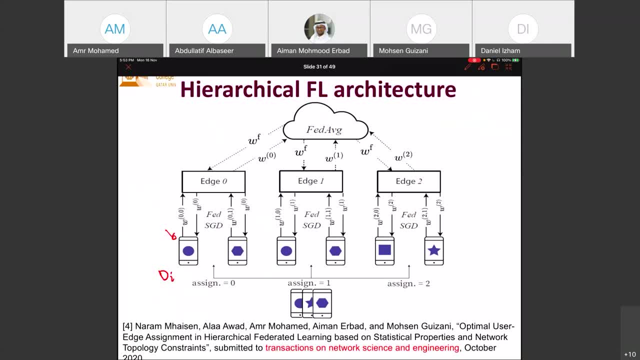 time that this camera sees a cat, something like that. okay, so, based on the distribution of the local data set, what? what this uh, uh optimal algorithm tries to do is to say: okay so, distribution, i need to assign this device, this stitch. okay, for example, what i need, okay, yeah. so this means that. 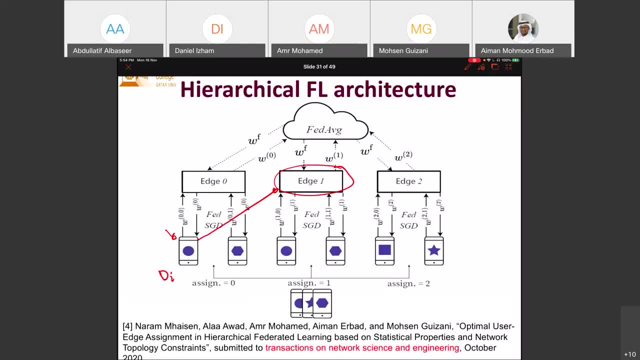 this level, this edge would have a data set that statistically closer to each other. okay, and by doing this at this level as well, i try to make the data statistically closer to each other, which which will affect the number of communication rounds. okay, that you have to go through in order. 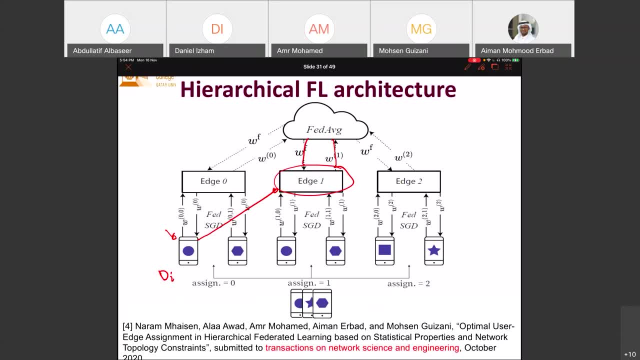 to have conversions. so by assigning the node, based on the statistical properties of the local data set to a specific edge, you try to minimize the communication round, communication rounds that you have to go through to achieve conversions. okay, okay, that's, that's what this work tries to do. okay, but, uh, okay, here, uh, do you think the privacy will be violated? 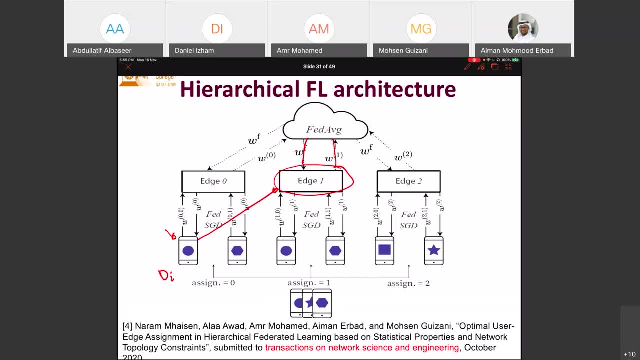 the privacy would be violated. if you need to know at the edge, if you need to know the data set at the device, no, but here on the data set of the device, then there is a privacy issue. but if you need to know the distribution of that data, then someone might argue that even this would be. 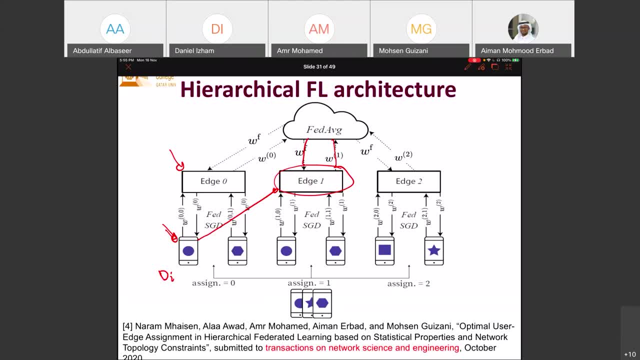 a privacy issue. but in that work to facilitate the distributed optimization, we need to have this assumption that the distribution of the, the local data set, is known a priori and i- and, by the way, this assumption is the basic assumption of maybe 50 of the work in this area, so not just this. 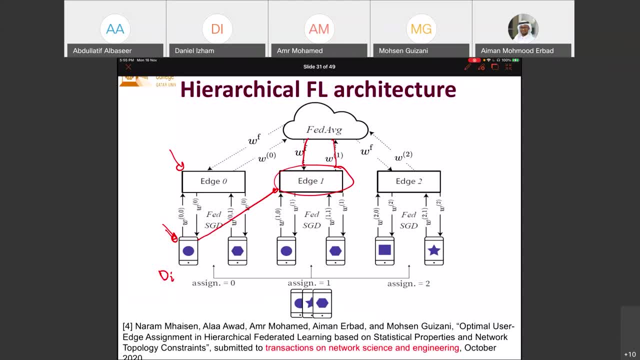 work in because we, so we, we have to have this assumption in order to facilitate the, uh, the, the mathematical analysis, because this, uh, this paper, by the way, goes through very, very rigorous mathematical analysis to derive the, the boundaries of, uh, uh, of the of this divergence factor. okay, so this divergence factor which i have mentioned here, 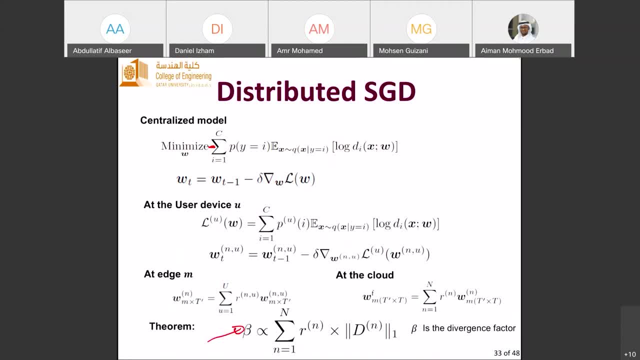 okay. so in order to reach to that particular state, you have to to do some rigorous mathematical analysis, to uh to, to know that the divergence factor is indeed proportional to the distribution of the data at the edge. and how to do this uh distribution and how to control it. to control it. 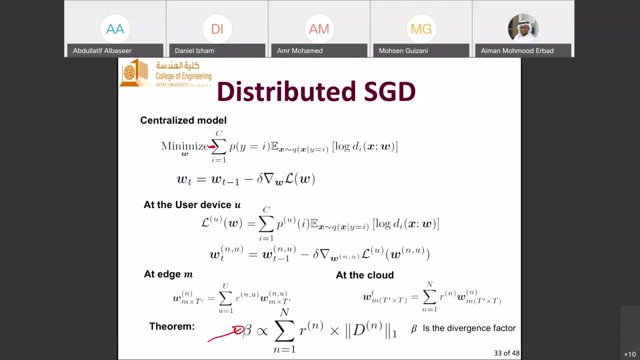 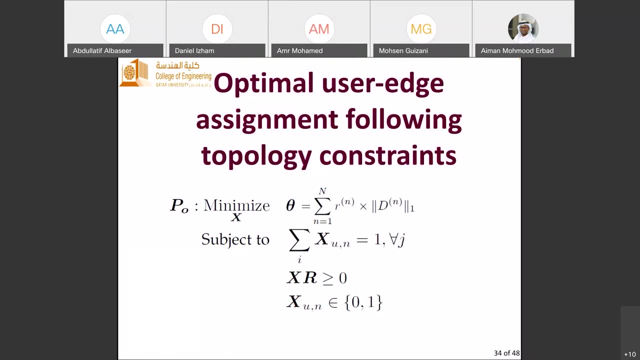 of course, is to position or to attach a specific node to a specific edge. okay, in order to minimize that divergence factor. not only that, really the this work also goes through some rigorous, systematic analysis to try to simplify this optimization problem. because what? yeah, this problem, although it looks simpler compared to the optimization problems we talked, 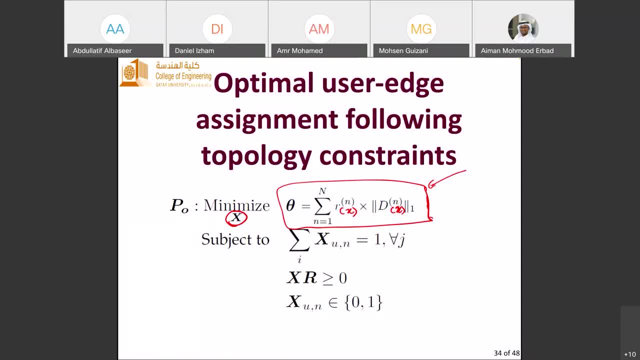 about before. however, uh, this problem is highly complex because it's non-linear integer uh program and uh in the paper we. we actually try to simplify this through multiple steps uh to to try to use some of the common techniques, like branch and bound techniques to uh to make the solution of this problem more efficient. 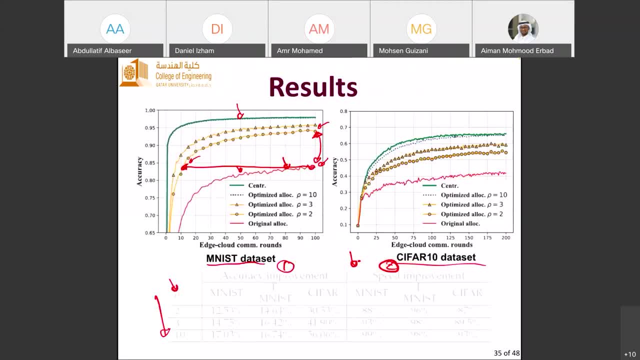 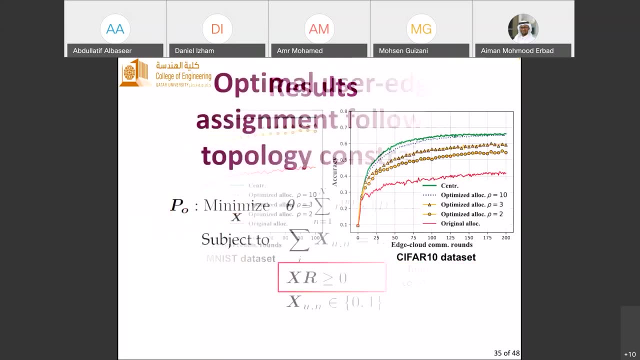 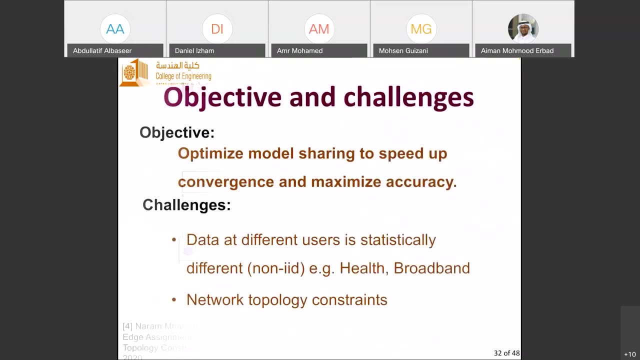 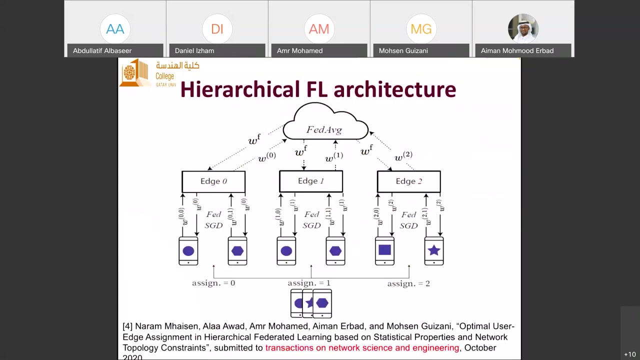 okay, okay, i have one last question, please, regarding the system mode, the system. please can you go to the system now for federated specific gradient descent? uh, the edge user should repeat, or uh, should send the update every single local step. right, it's clear that you are deeply into that area. yes, you're right. 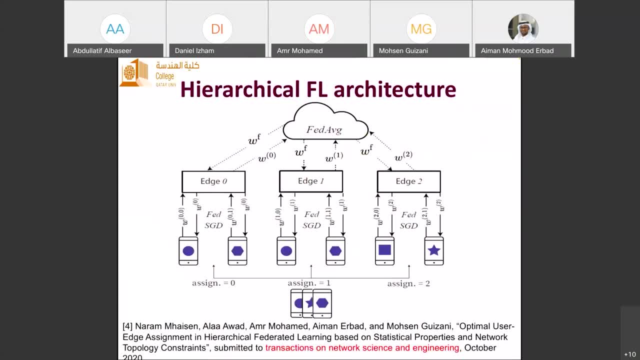 this is this color area. okay, go ahead, go ahead. okay. uh, do you think this is will be uh extensive? uh, regarding the communication, uh resources? uh, of course not, but the assumption here, the assumption here, is that the communication between the edge and the device is, is, is very low cost. 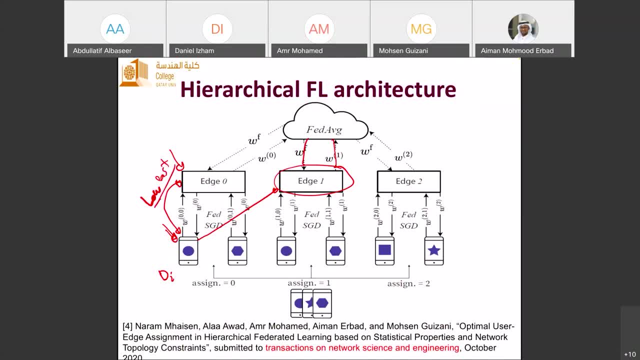 that's why really, we have this edge, because the edges are supposed to be close to the, the devices, in such a way that allows you to use very low power communication like, for example, bluetooth or lora or something like this. okay, but will minimize. okay, but we, we have a model size. 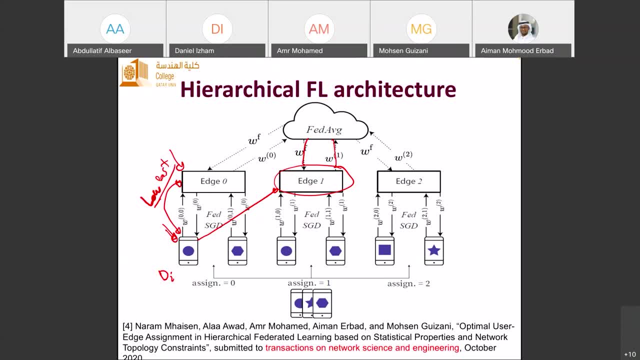 sometimes the model size constitutes million to billions of parameters like cnn or dense notes. this will, yes, this will make the communication here uh, uh quite expensive. and you are perfectly right, the? uh remember here: the assumption of the fact that the weights are exchanged per iteration is to facilitate the statistical analysis. 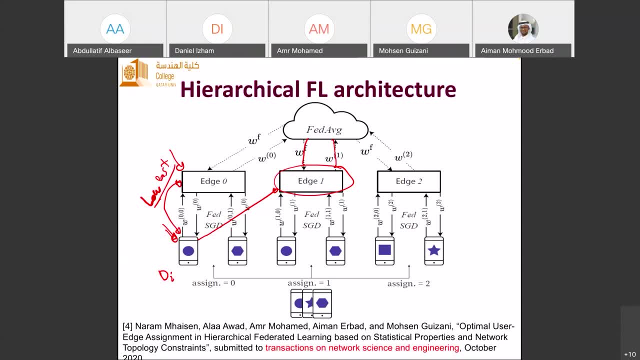 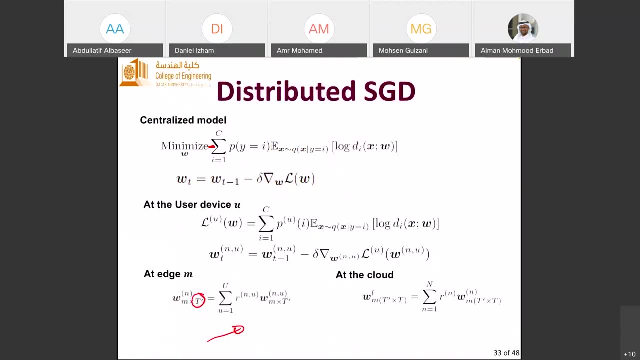 but empirically you can use uh, you can exchange the, uh, the weights, every specific number of iterations, and this is what i have actually explained in this modeling right. so when i said that every t dash, okay, every t dash, you need to exchange the weights, right, so you can really exchange the weights every like, for example, 100 iterations, which 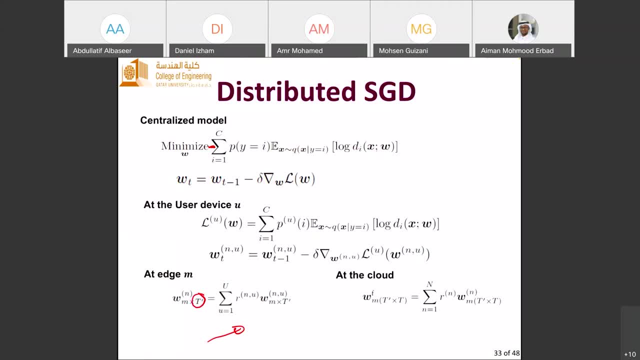 which will make the communication cost even less. however, the, the, we, we had to make the assumption that this t dash equal to one, only to facilitate the statistical, uh or the mathematical derivations. okay, so to facilitate the mathematical derivation and reach to that theorem, for example, we had to make the assumption that t dash is one. okay, this is in. 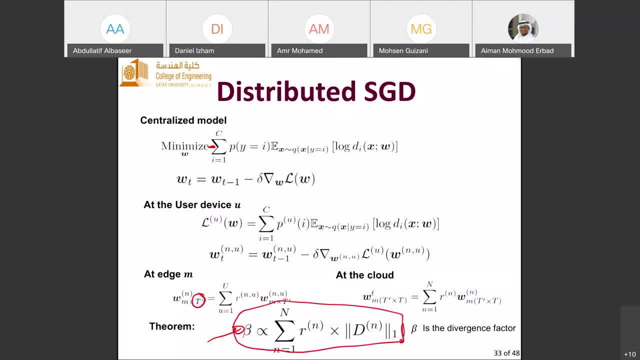 case of using stochastic gradient descent. right, if we have many batches, that's a gradient descent. the imbalance data set will affect strongly the number of local objects. yes, you're right. yes, yes, i can. i can really estimate the optimal t dash. that, again, that minimizes the divergence factor. you are perfectly right, and this is actually the extension that we. 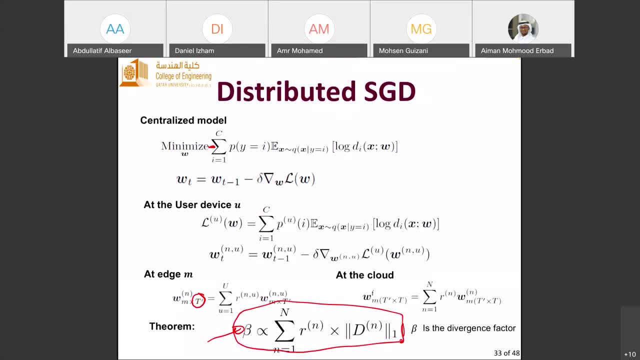 are trying to do now. however, for that particular work, we did not address this and, in order to minimize the divergence factor, we have simply assumed that t dash is one to facilitate the mathematical analysis. just to to, to make it simpler, okay. but again, analytically you can use: 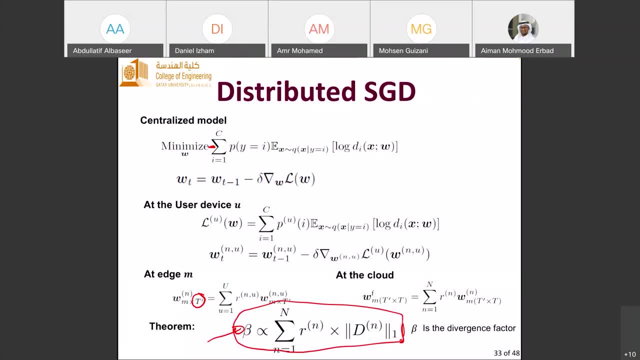 any arbitrary t dash. you are allowed to use any arbitrary t dash, there is no problem. okay, but we will have a problem with the synchronization. yes, actually, yeah, you are bringing. a very interesting point here is that here i did not even say that t dash is different from one device to 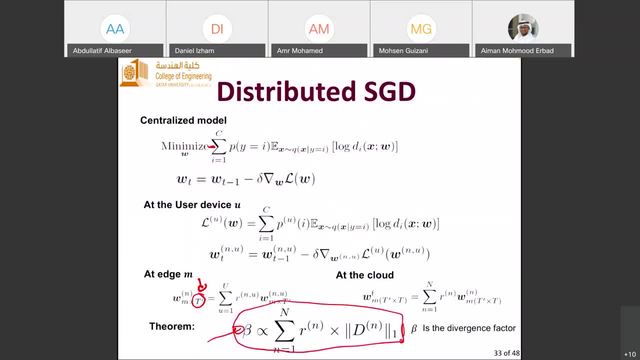 another. in fact, you could have a different t dash from one device to another, in which case you have asynchronous communication. similar is so. this is what you are referring to. so, for example, if i have, if i have a device here and i have multiple edges or multiple devices, okay, and i'm trying to. 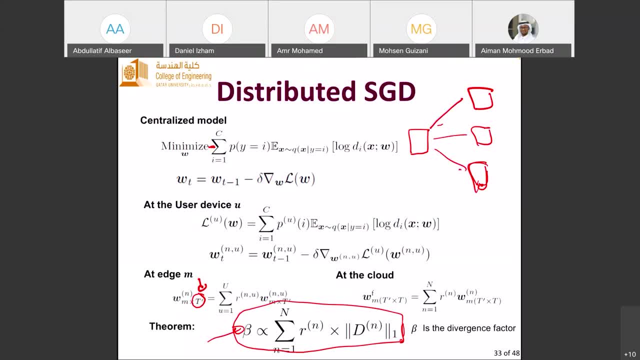 change the weights, okay, with uh, with the, with the, with these devices, so, so, if, if, if t dash here is is different from here, okay, then we end up with asynchronous communication. so what is the effect of this on the conversions? what is the effect of this on the accuracy? 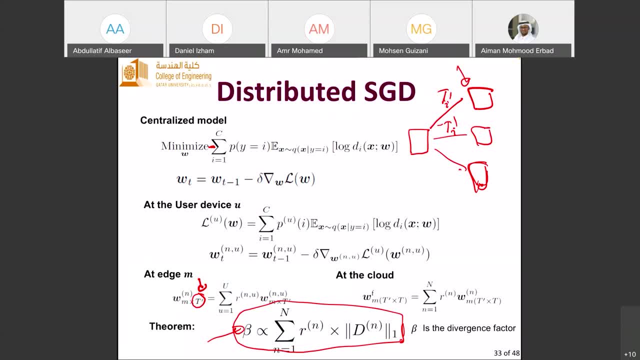 that requires, that requires some analysis. yeah, it depends on the distribution of the data itself. sahih, it depends on the statistical distribution of the data and also it. it depends on the communication cost between the, the the devices. so some devices they would. they would have, for example, better wireless channel gain, in which case 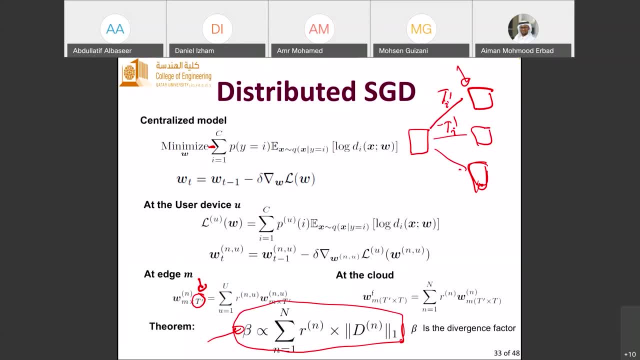 exchanging the- uh, the weights more often would not be that expensive other devices they will have a low channel gain, in which case the communication would be very, very expensive. so you would want to exchange the weights less often. okay, but i have, we have thought about all these issues, but, but in 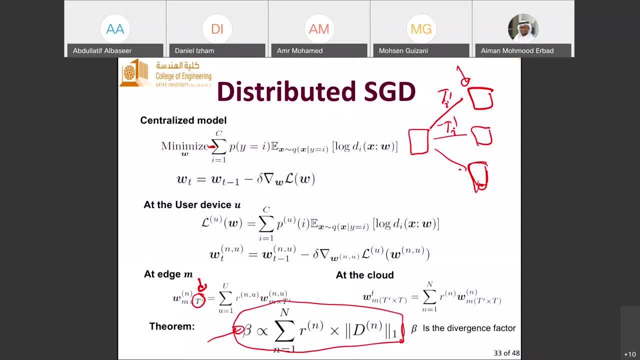 terms of mathematical analysis. we had to make certain assumptions to rule out some of these aspects and focus on particular aspects that are addressed in this particular work. Fadlal uh. okay for the uh channel game between the edge server and the end users. i think it is a selection phase in this uh integrated learning. 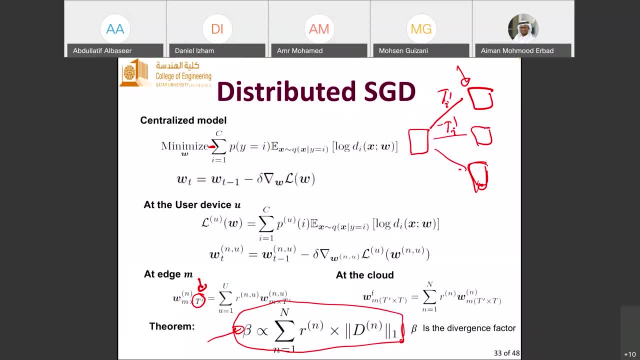 yes to the learning, so this problem can be considered at the edge level. yeah, we do it at the edge level. yes, here now we do it at the edge level. but what i'm trying to say is that if you have a problem on a certain level, maybe it's a problem that is very high or high, or 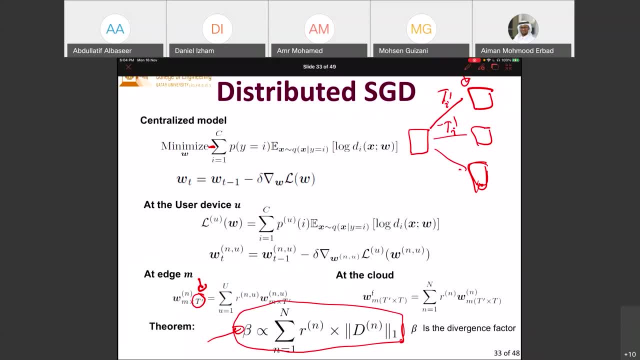 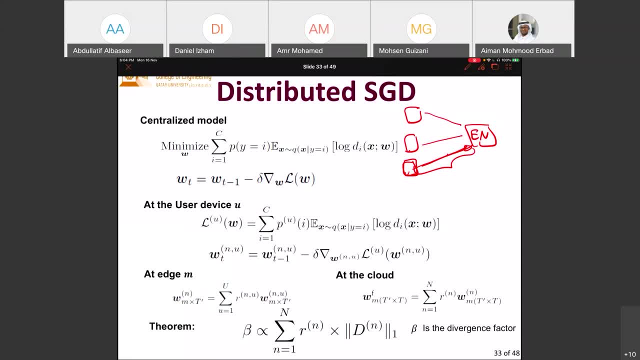 It's because of the fact that this link is is really good. This device is a poor device and the link between it and the edge is not as good as other devices, So in that case you need to exchange the weights less often. 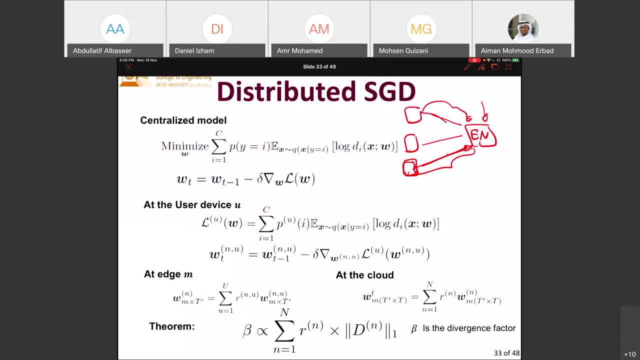 Yeah, In all cases, they all exchange the weights with the edge. But if they change, if they, if they exchange these weights using different frequencies or, in other words, different T-dash, what is the effect of this on the accuracy, on the speed of conversions, on this kind of things? 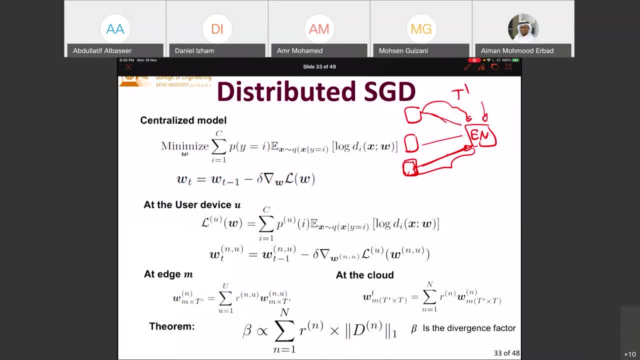 That's what needs more analysis, And we did not address that as part of this work. Also, I think that the edge server can allocate more bandwidth to the user, Because I think that's exactly that's exactly what we're doing now. 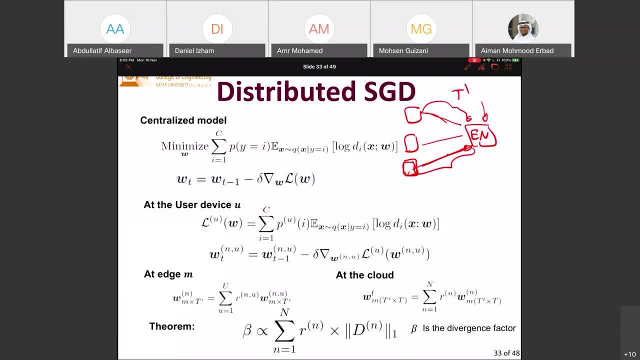 That's exactly what we're trying to do now. But again, I mean, in order to try to optimize this, you have to have, you have to formulate an objective for the, the minimization function, And in that case, uh, 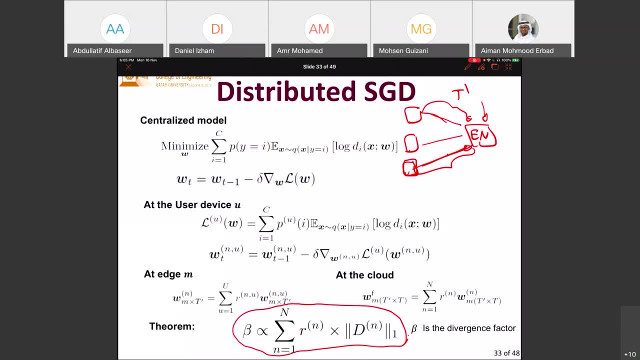 different because of the difference in the system model that you are proposing now. Uh, in this particular work, because of the the assumptions we made, we were able to formulate the optimization problem using these particular components, which can be minimized in real time. 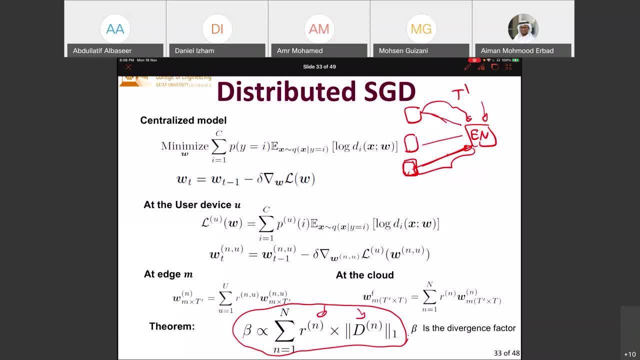 Okay, If you, if you assume, for example, asynchronous communication, if you assume different channel gain, if you assume bandwidth provisioning, this will make the objective totally different, totally different, And the optimization problem will change drastically And, in fact, 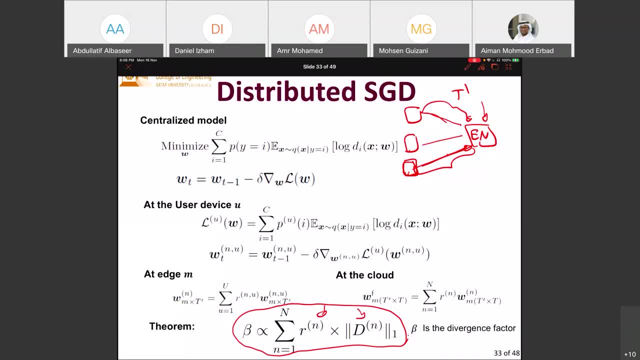 we are trying to to do that now as part of the extension of this work. I think someone else is raising his hand. Uh, hello professor. No, no, it was just a mistake. Sorry, I'm sorry, Okay. 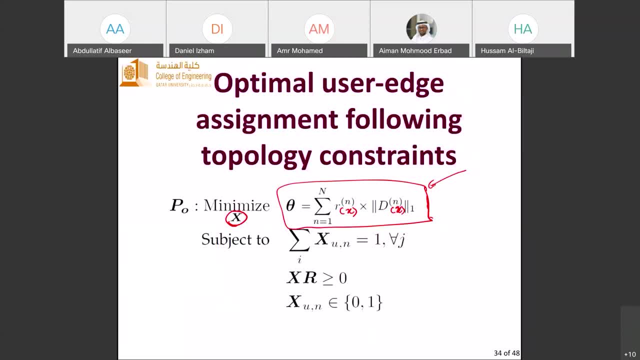 Okay, Dr, I have a question. There is a question also. go ahead, Yes, Yes, sir. Uh, actually, regarding the scalability of the solution here, the hierarchical one, we have scalability in the number of edges and the number of nodes. 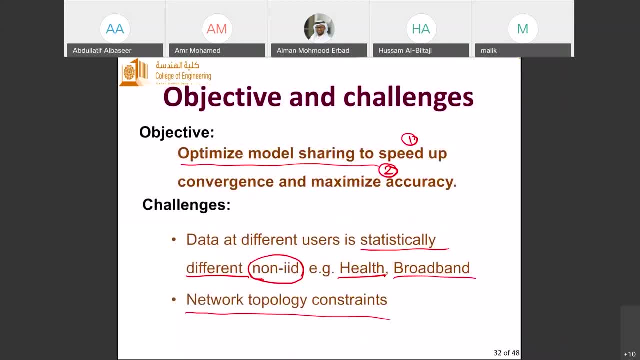 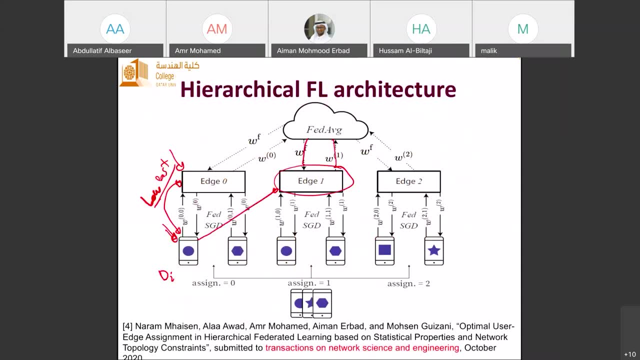 How to consider this one in your model. Yeah, The scalability is addressed in this model in multiple stages. Uh, first, really, the hierarchical nature of this model. Okay, Addresses the scalability, as we have of course talked in the very uh. 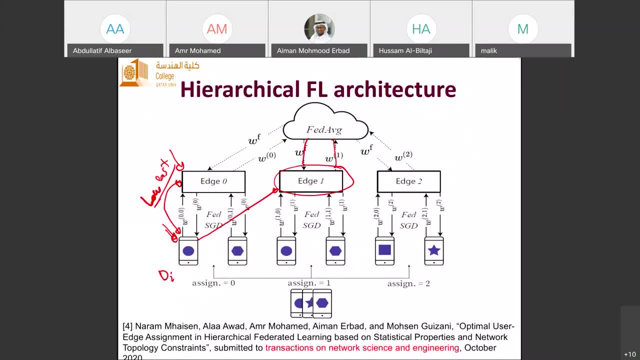 beginning of this presentation, when we talked about the edge computing as a way to address scalability. So so, by by exchanging the weights with the edges, that really should enhance the scalability issues And and this is what we have indeed seen from the results. 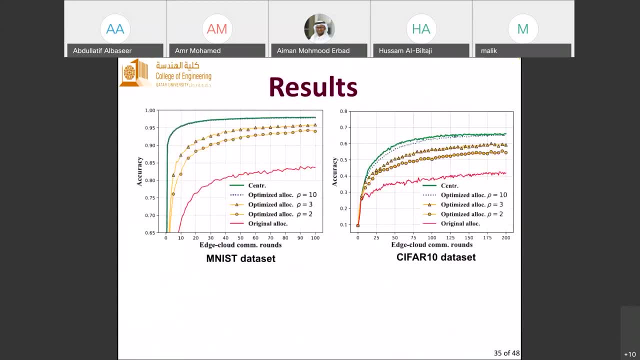 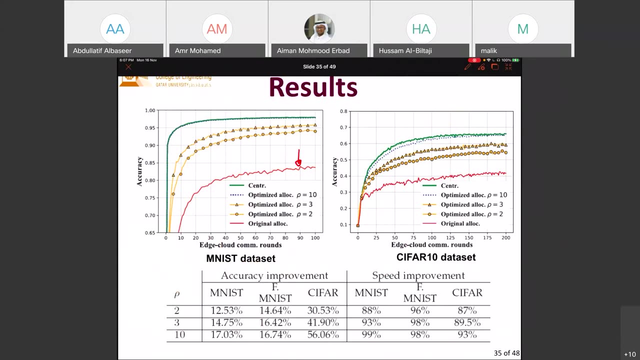 If you, uh, if you take a look at the results here. so we have seen here from the results that, uh, this is the the federated learning, the clear, sorry, the the red. So this red curve is the federated learning without the edges. 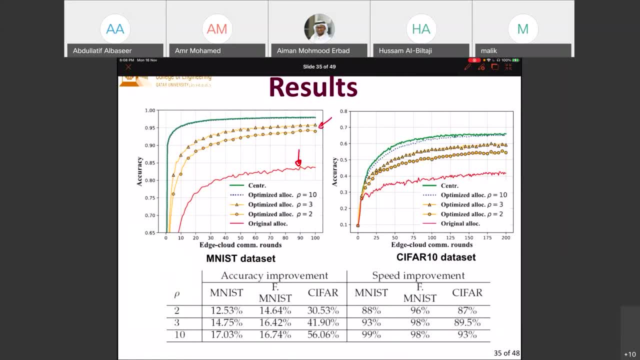 Okay, This is the hierarchical federated learning part. So the performance has been enhanced a lot with the, with the concept of hierarchical federated learning. but that's not the only stage where we add the scalability, Also the another aspect of the solution. 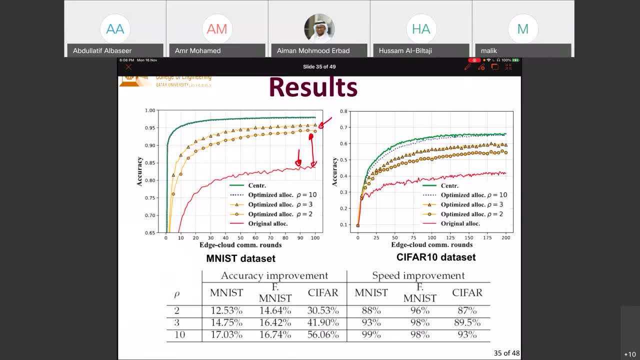 which I did not cover here- where to divide The users into groups. So, for example, if you have hundreds of thousands of users in the country and you're trying to perform federated learning, of course, even with the edge computing. 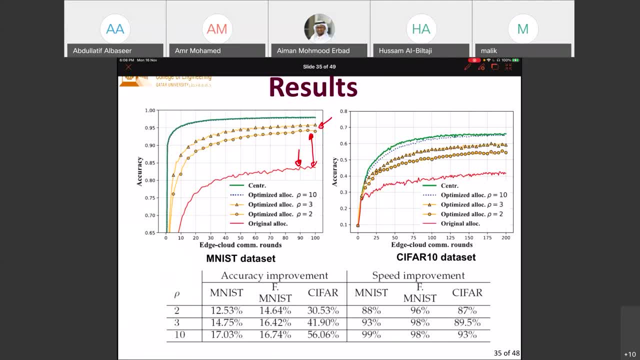 you're going to have to have a scalability issue, or you may have a scalability issue, In which case the first thing we do here is to try to logically, logically uh- group the users or cluster the users into groups, Uh. 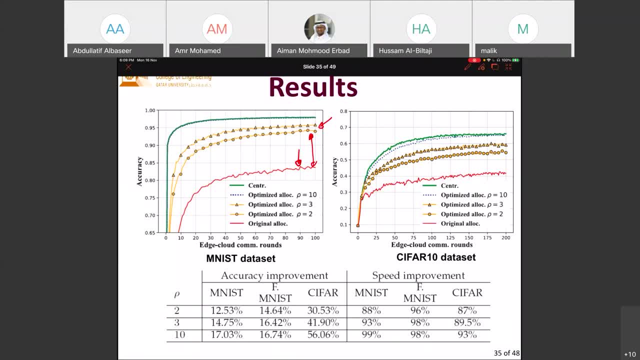 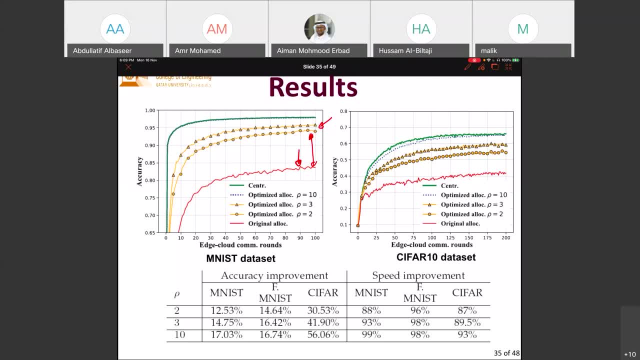 Uh, so these group of users? they see a cat- uh uh uh- 50% of the time and they see a dog 50% of the time, something like that. Okay, So by grouping, by this logical grouping of the users, 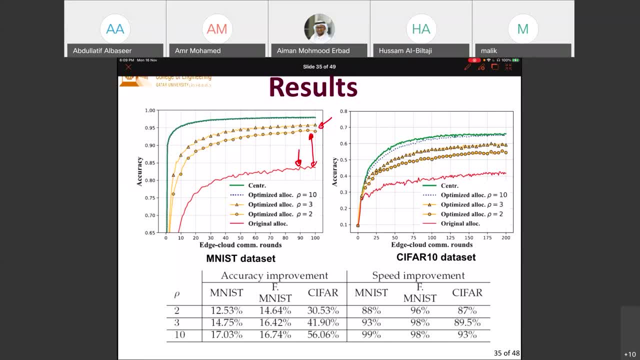 Okay. So we try to allocate group of users in one shot to the edge, Okay, As opposed to single user. So this also addresses the skill ability issue by allocating group of users to an edge, not a single user to an edge. 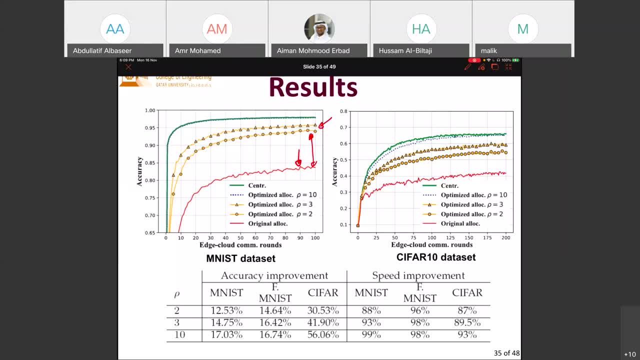 So this makes actually the solution much faster and more scalable for large number of users. Okay, So these are different levels where we address the scalability. I'm very glad, by the way, with this. yeah, any any questions, because it's really enriches the discussion and hopefully it's for the benefit of everyone. 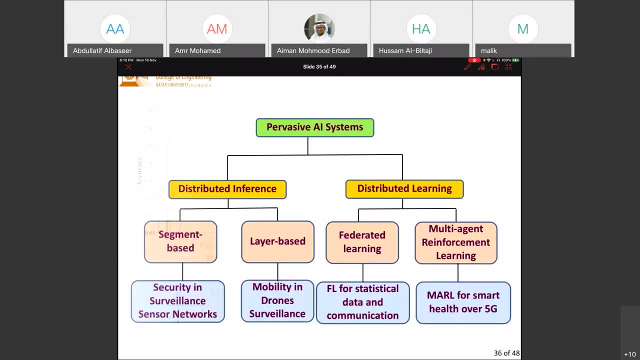 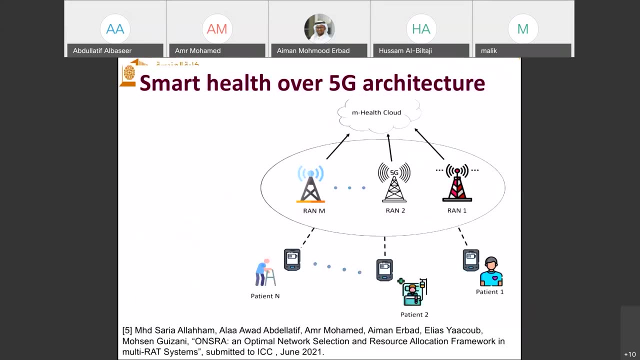 And, uh, I don't know. now we can move to the, the last part of the uh multi agent reinforcement learning, and I don't see any objection to move on. So I'll move on. Go ahead, All right. 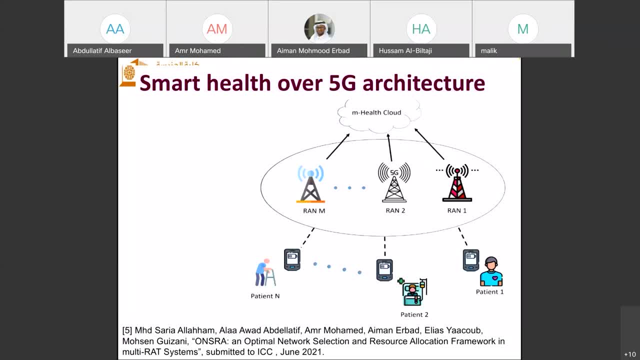 So okay, So for this particular use case, what we have is, in fact, a smart health application over five G networks. So this use case is particularly interesting because it addresses some of the issues that we have nowadays, like, for example, 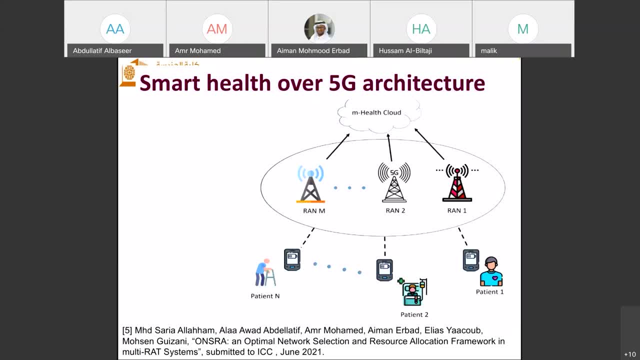 the covered 19.. And so the idea here is that, for, for each individual user, we perform remote monitoring. Okay, And here what we're trying to do is that, through the uh, the vital signs- each user will try to uh. 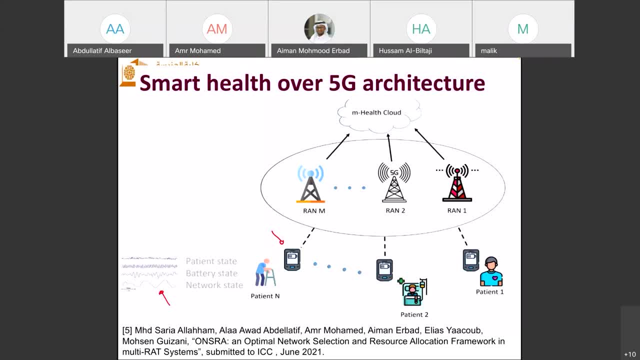 we'll try to perform some processing using a I okay, based on patient state, battery state, network state. So, for example, think about uh application, for example. so imagine hundreds of of patients or hundreds of users across the country. they have a close application. 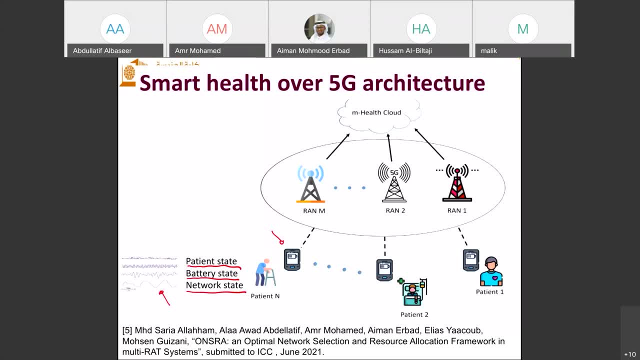 right, And we need to make a cross application more intelligent and smarter than what it really is now. Okay, So first we need to perform some uh customization of vital signs at each user level, based on the patient state, For example. 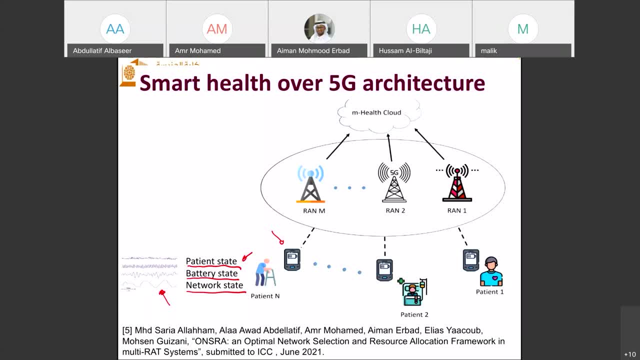 if the patient has seizure or the patient has heart attack, this vital sign becomes really really important and critical and it needs to be delivered to the cloud right away because there is some emergency case. and not only that. this signal, this uh. 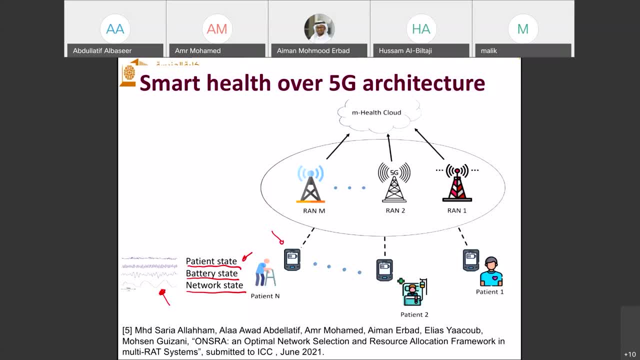 these vital sign needs to be very, very accurate, and there is no compromise to the accuracy of this vital sign because of the fact that patient is currently having a certain disorder. Okay, So, based on that, the, the, the, uh, the smart application at the patient level will perform. 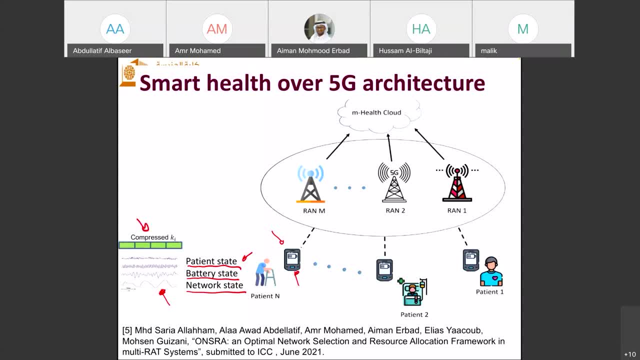 what we call adaptive compression. So adaptive compression here is basically to try to compress these vital signs before delivery. Okay, And then we tried to split the compressed data across the different radio access networks. So 5G proposes heterogeneous architecture where you have heterogeneous types of networks. 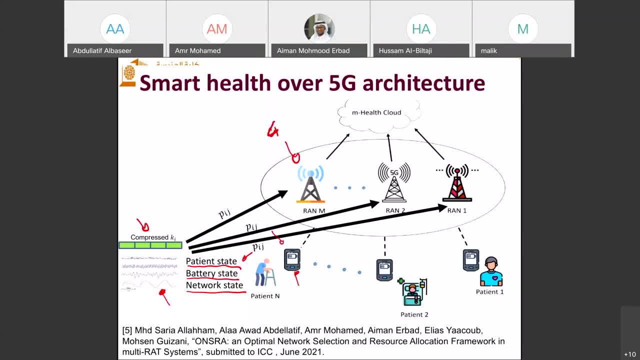 So, for example, this one is is 4G, This one, for example, is uh uh uh. this one is a uh uh uh, this one is a muscle on wifi. Okay, So each radio access network has certain resources that it can assign to the different. 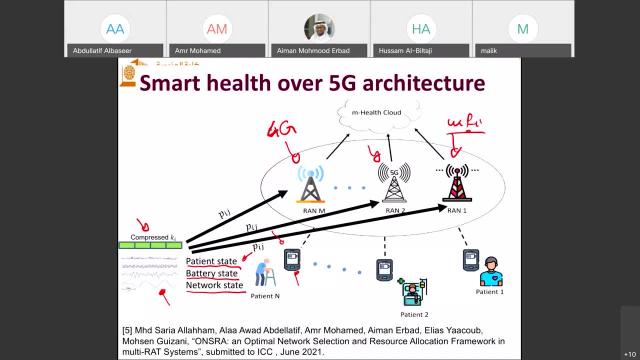 uh user. based on allocating the resources from the radio access technology to the individual users, users will can deliver their vital signs with a specific performance. Okay So, uh, uh, uh, uh uh performance. okay so again, the idea here is that based on the patient state, based 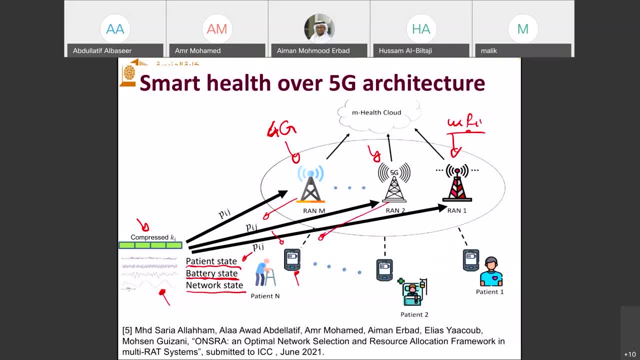 on the battery level of the of the cell phone or the edge node and, based on the network state, how many rands or how many radio access networks the user has access to. okay, in which case the user can split the traffic across the different trends in order to get certain performance end-to-end. so the objective 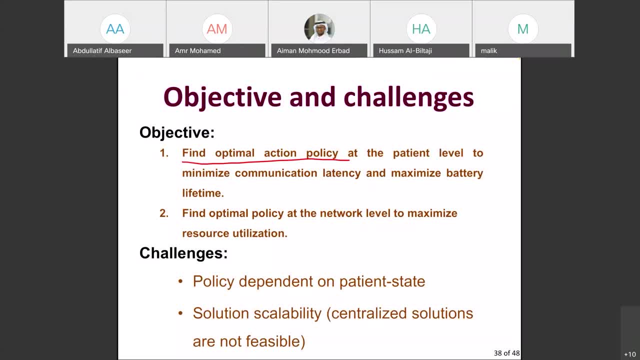 of this work is to try to find the optimal action policy at the patient level, which means: what is the, what is the appropriate compression ratio level that we can use at the patient level? what is the split of the traffic across the different rands in order to minimize the latency and maximize the battery? 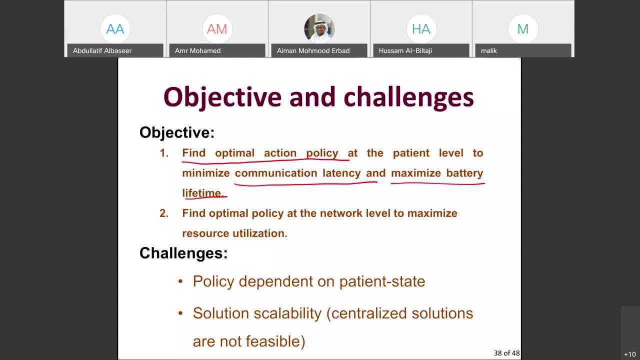 lifetime over time, maximize the the device lifetime in terms of battery. okay, but this is not the only objective. the other combined objective that goes with it is that, at the network level, we need to also devise an optimal policy to allocate the resources in order to maximize the resources of the network. right, so it's, it's, you can think of it. 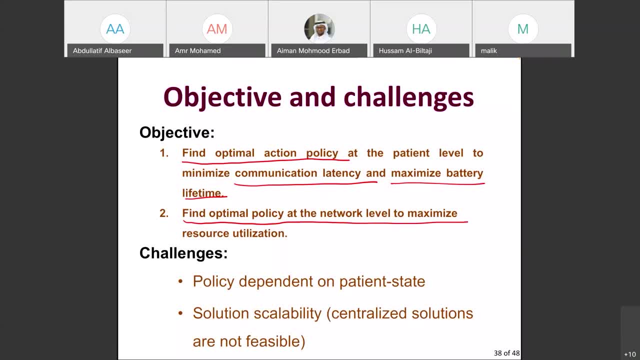 as a game where the users are trying to gain and as much resources as possible from the different radio access networks and, at the same time, the radio access networks are trying to allocate the resources smartly to the different users in order to optimize their user experience. okay, 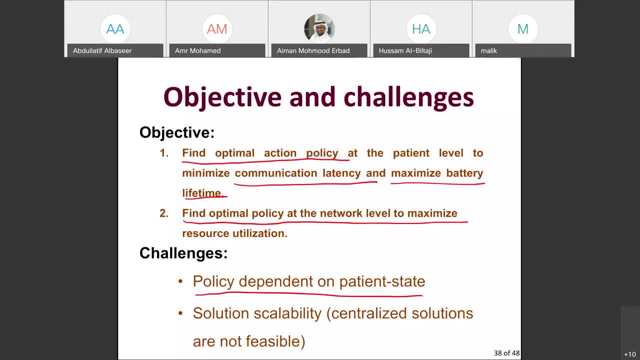 and the challenge here is that the policy that you need to devise is, in fact, based on the patient state, and that's what's different about this work- is that we have to take the patient state into consideration, and we have to take into consideration if the patient is having seizure, or the patient is having a heart attack or any kind of disorder. i cannot assume that the data has to be transferred with the same level of urgency and with the same performance, like the person who is norman. okay, so i have to watch for the patient state. not only that, i have to watch also for the battery level of the cell phone and so on, and also the solution scalability. so any centralized solution in that case would not be feasible, because 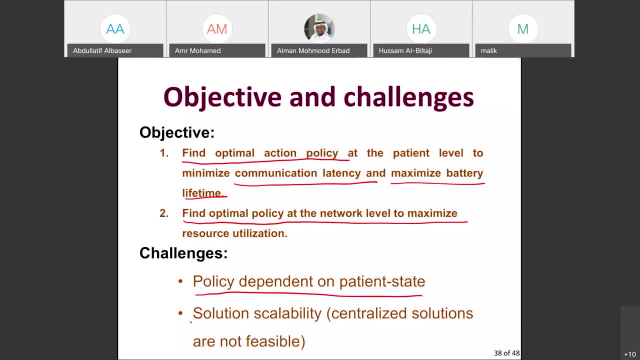 and also the solution scalability. so any centralized solution in that case would not be feasible because, Because of the fact that, uh, I cannot uh assume that the network would tell the user compress the data in this way. No, this decision has to be taken by the individual user. 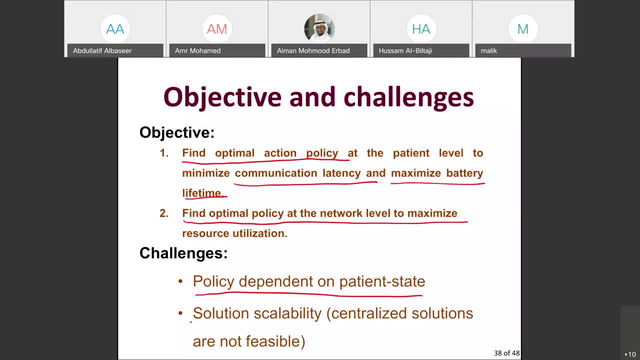 Okay, the network can allocate resources, but cannot allocate how the user is really, uh, customizing the data that it's being transferred. All right, so the objective, this is. this- is the- I mean a very, very complex problem in that case. 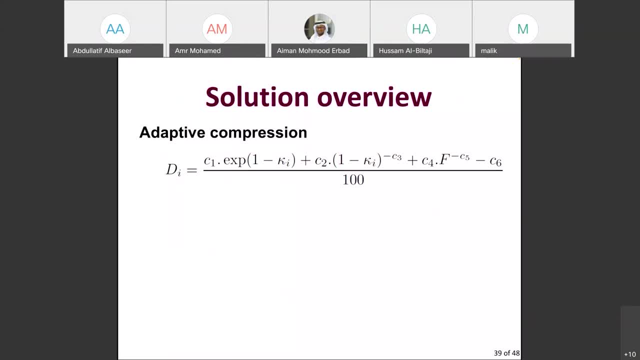 So, in order to facilitate the uh um the optimization, in this case we device different models. The 1st model is the adaptive compression model, And here the adaptive compression model tries to estimate the portion of the data based on performing. 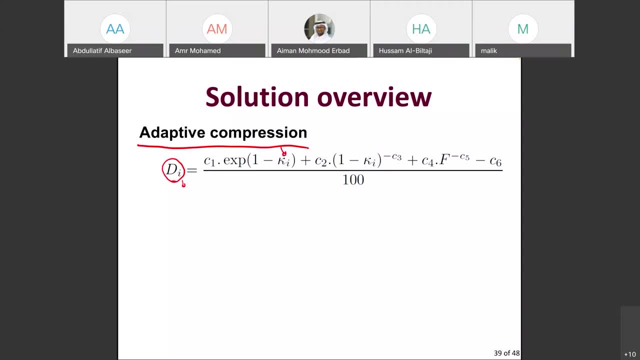 A certain compression to be listed, And the distortion is the amount of information loss In this particular Vital sign, based on the fact that we compress the data up to that compression level. Okay, and here we have. we have in fact done this adaptive compression using multiple techniques, using machine learning, using uh uh, um, digital Wavelet transform, using different uh, uh uh techniques and uh. we can map these techniques to that mathematical model which later on facilitates the uh, the optimization framework. 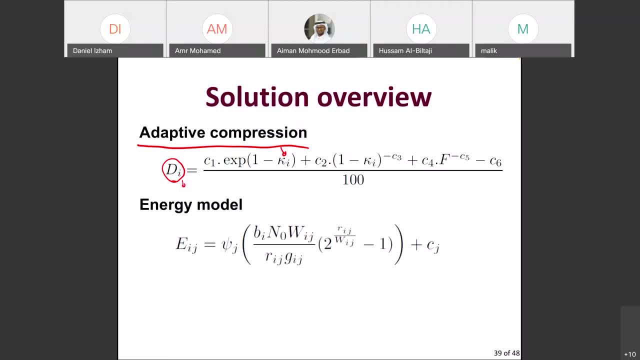 The 2nd model here is the energy model. The energy model is the amount of energy that I need to spend in order to send A unit of data to a particular redegie access network. Okay, so this is based on the famous uh relay, uh channel model. 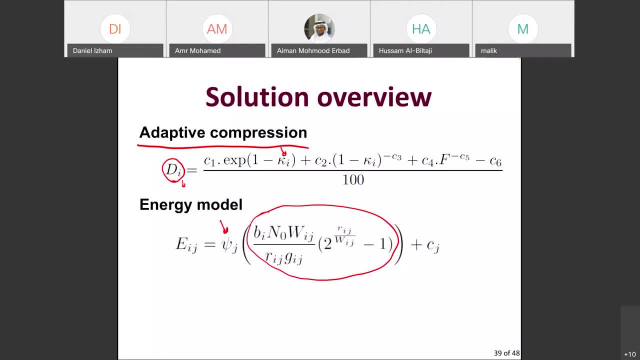 Okay, except that this model is, in fact, uh uh, uh, uh, uh uh, proportional 2, a specific parameter, parameter parameters which is upside J and CJ, which are distinct for each radio access network. So each network would have different constants for upside J and CJ. 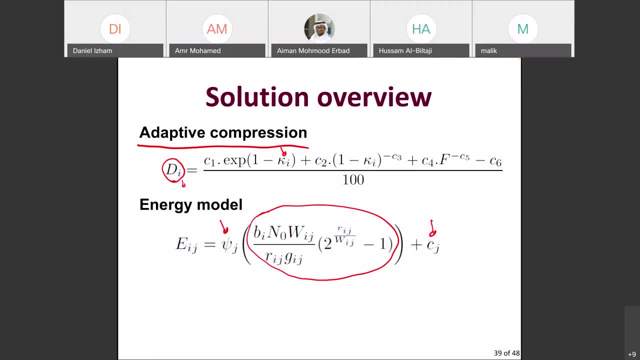 So by changing these constants, I make the uh uh, uh uh each ran more energy hungry or less energy hungry. Okay, So there are some uh energy requirements different for each rank. The third model is the latency model, which is the most. it's the simplest model, which. 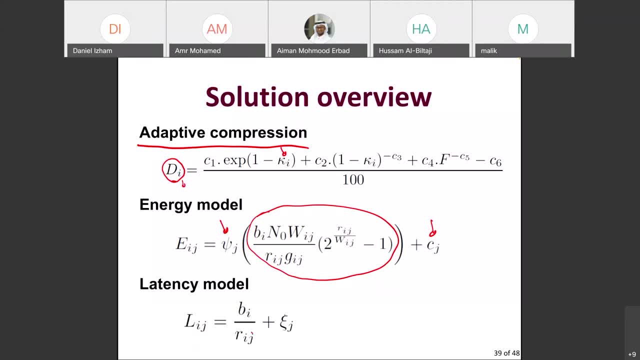 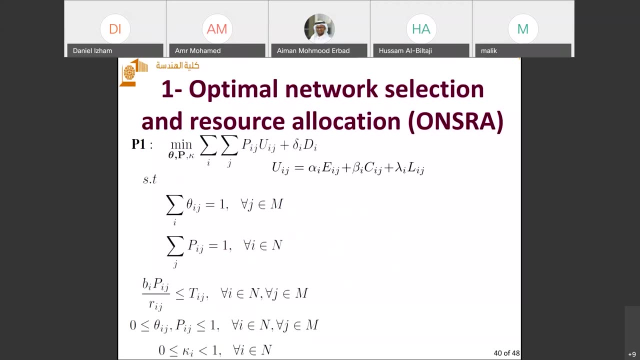 is based on the estimated rate, okay, Which is based on, again, the Rayleigh channel model, uh, and based on that we can estimate the latency model. So, based on this, we have a game. uh uh uh, solve this problem in two different ways. 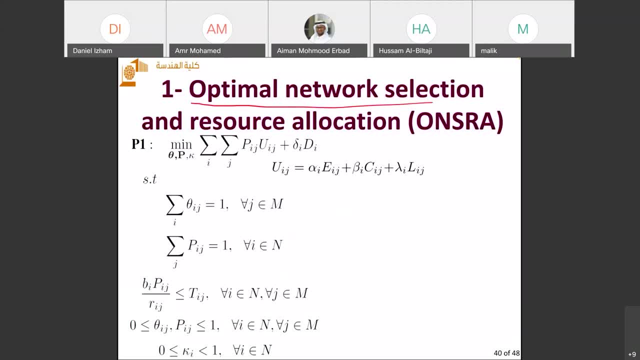 The first Is using distributed optimization framework where we have modeled the uh. so we need to. we need to minimize a multi objective problem in that case. So the we have to minimize utility at the user level by addressing the uh. the compromise: 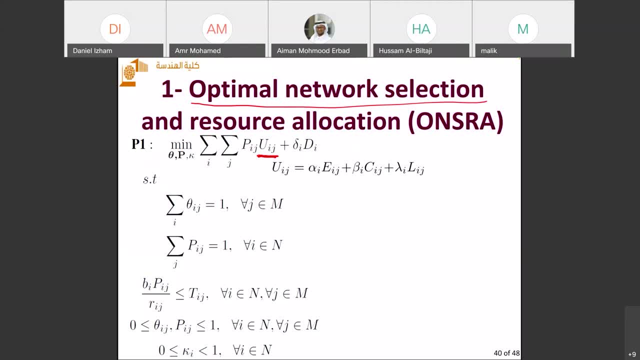 or addressing the trade off between three different components: the consumption at the device level. The monetary fund- Okay, The amount of Uh money that you have to pay in order to send that data. and the latency, or the amount of time that you have to spend to send unit of data to this particular radio access network. 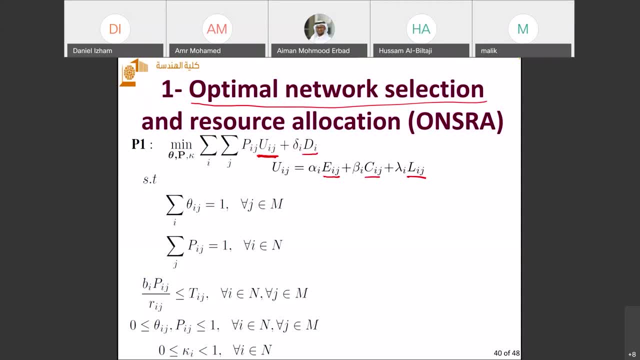 And also we need to minimize the distortion, in which case we need to preserve the quality of the vital signs And we need to address the trade off between all these four components. So we have four components in total. Okay, So the energy, The course. 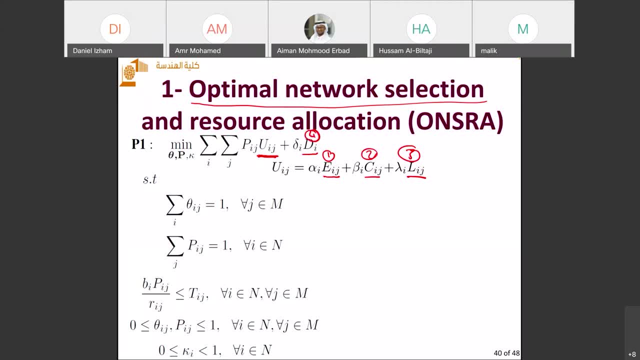 The latency, The distortion. Okay, So we need to find the optimal trade off between all these four components, And this is, of course, subject to some. this is the bandwidth allocation from the network, And P here is the split factor where, uh, we need to split the traffic from each user. 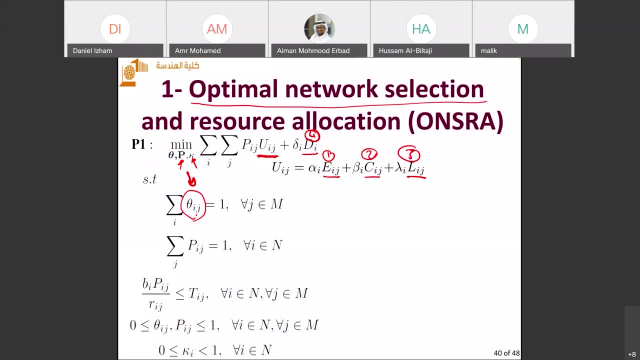 to different radio access network at each user will also need to do a certain level of compression to the data. Okay, Okay, So this uh, this uh uh optimization problem, as you can imagine is is really really. 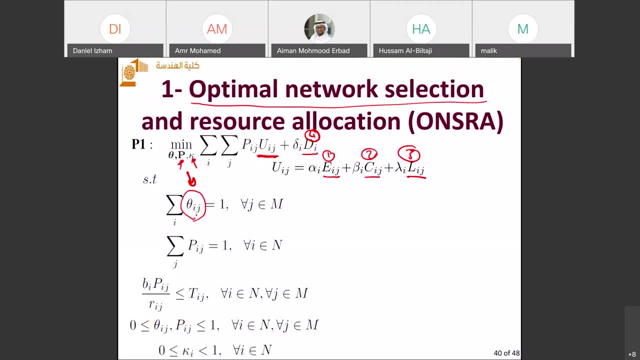 complex. Uh, not only it's uh, uh, it's nonlinear, it's actually nonlinear in all these parameters, Okay, And uh, in that case, uh, it's really highly complex. And also, if we solve this problem in that way, the solution would be centralized, which? 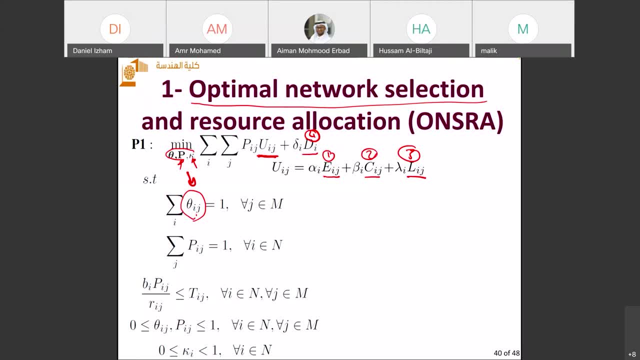 as I said before, it's not feasible for uh the, uh the network that we are talking about. So instead, what we did is that we have, in fact, uh uh divided this P1 problem into two sub-problems. 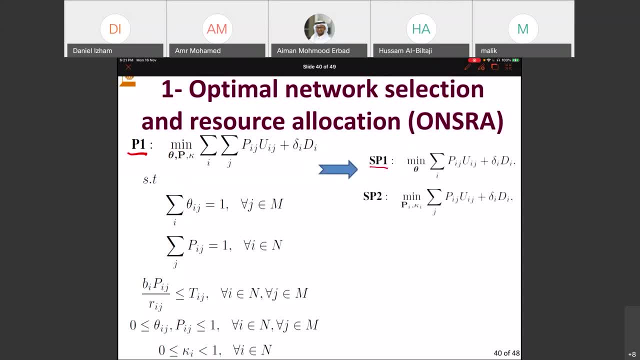 Okay. So sub-problem one would be: would, would run at the network and would try to do the bandwidth allocation at the network first. Okay, Okay, Okay, Okay, Okay. So, uh, in that case, uh, we would get the unaligned bandwidth, so we would get the. 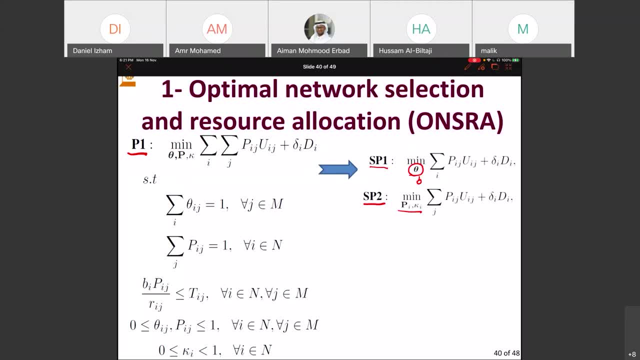 allocated bandwidth to the individual users and the users would then try to run the uh. the second sub-problem where they need to split the, the, the vital signs, across the different radio access network and they would need to estimate the, the uh, the compression. 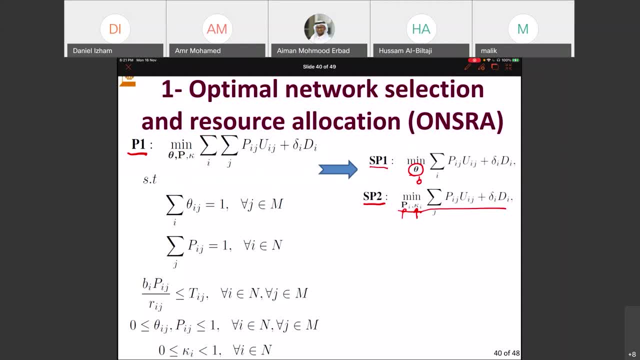 level at each user And they need to do that iteratively, as we will see in a minute. So we have went further and we tried to subdivide sub problem 2 into 2 sub sub problems to try to simplify the the solution even more. 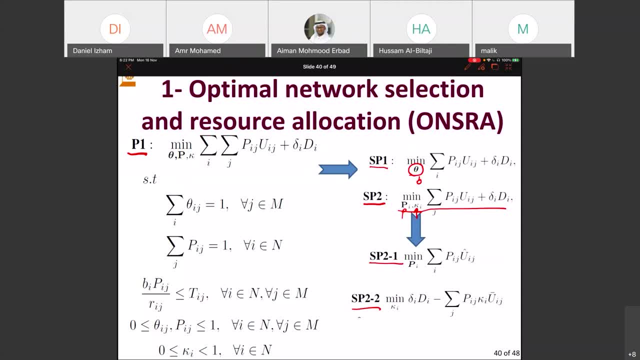 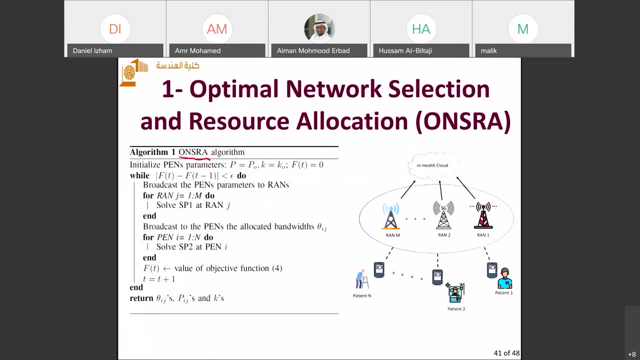 And we perform these 2 sub problems, uh, in some cases using some closed form solution which speeds up The uh, the overall solution, significantly. So this is the uh, the, the overall algorithm Which we call it on, or uh, optimal network selection and radio resource allocation. Okay, Okay, So the, the idea of this algorithm, 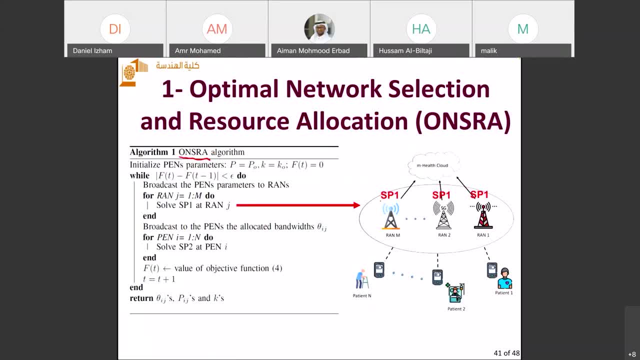 Is that, 1st, we try to uh solve the, uh the sub problem 1 at each individual radio access network To try to allocate the bandwidth Okay by solving a small optimization problem at each Okay localized. and then, after we do this, 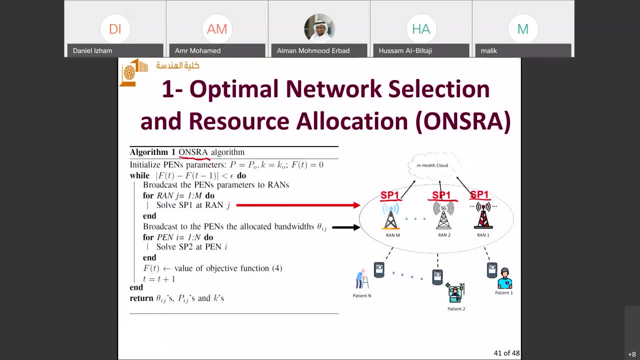 We send. we send the allocated bandwidth To the individual users, and individual users can then, uh uh uh, run the sub problem too by trying to estimate the optimal network indicators, how they will split Their traffic across the different trends and what is the compression level that they need to have locally at each year. 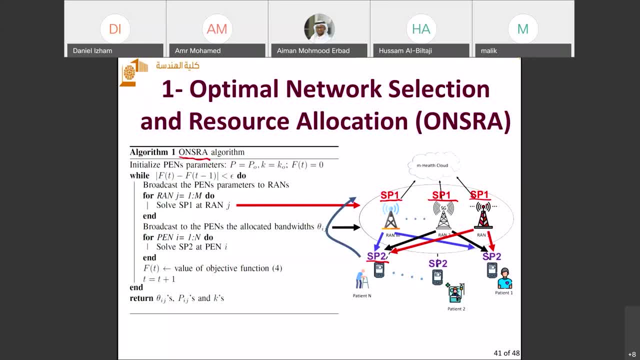 Okay, and we do that iteratively Until we achieve certain conversions. so basically, by doing this, Sub problems- we have divided the big problem into smaller sub problems that can be solved in a distributed manner. And, by the way, this is not using. until now we are not using the. I will come next. 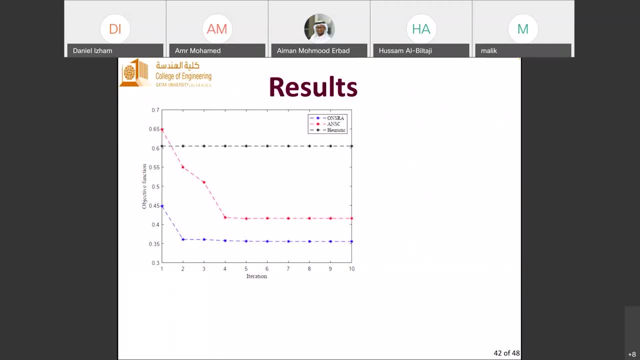 Okay. so the results here show that This particular distributed optimization is indeed, uh uh, uh uh, relatively efficient. And here the we compared this optimization solution with 2 state of the art solutions. 1 is by assuming a simple model at the network, that the network allocates resources equally between users. 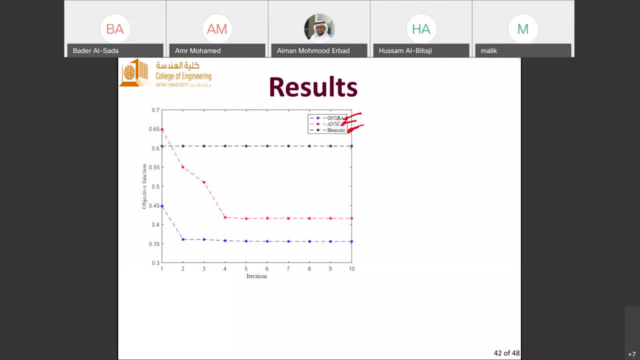 And this heuristic assumes that that the traffic is split equally, uh, on all lands. okay, so uh. by making the this comparison, we can see that blue curve here represents the uh, the answer, or the proposed optimization algorithm, which outperforms significantly the other heuristics or the other state-of-the-art techniques by significant amounts. 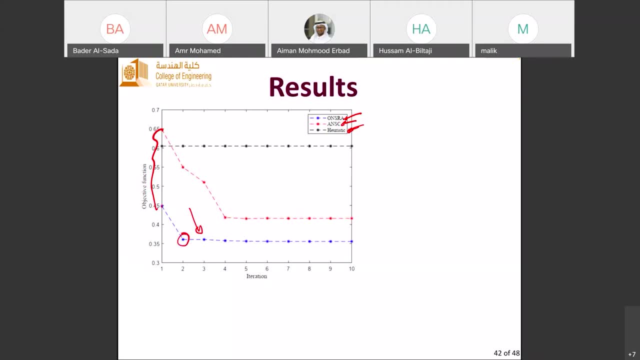 and also we notice here is that the iterations that are required to reach to the optimal solution are really quite low, so in some cases we need to go between the rands and- uh the users- maybe two times only to reach to the final solution, which is, which is relatively good news, that this can. 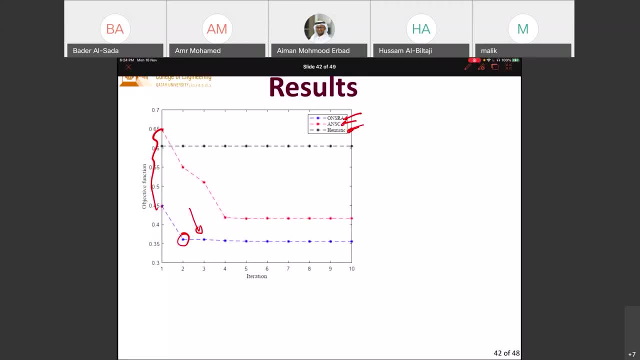 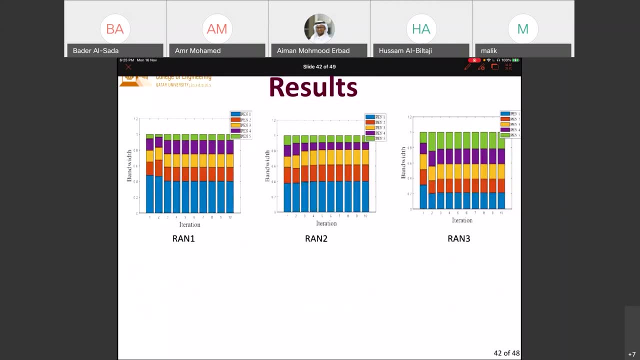 really perform a good performance overall, okay type. so you, we, we, we were able to uh, see how the different brands- now we have three rands, one of them is 4g, 5g and wi-fi, and of course, each one of them would have different communication requirements. 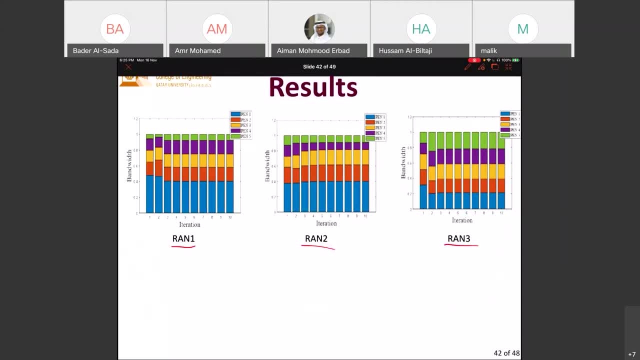 and uh different resources and, of course, different rates, allocation and so on, and we were able to see that uh, the user one which is the uh pervasive edge node one, the user edge one, has a different solution, because we are actually watching in randy model charges Santo on uh system tasks. 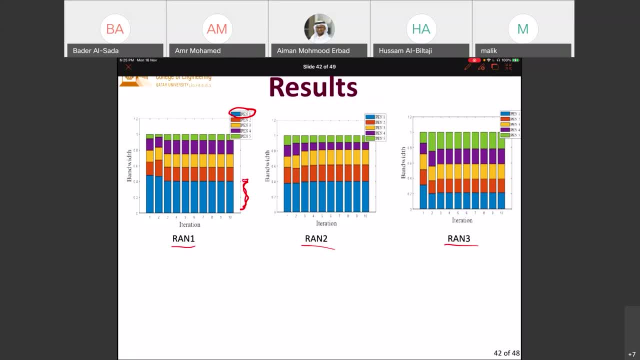 and then we can see the levels of the rammd code are depending on the possibilities, forroughness, um, and even if the g-resistance is uh depends on the band library universo, uh exchange rate by the farther layer to already solve thened. so with that, 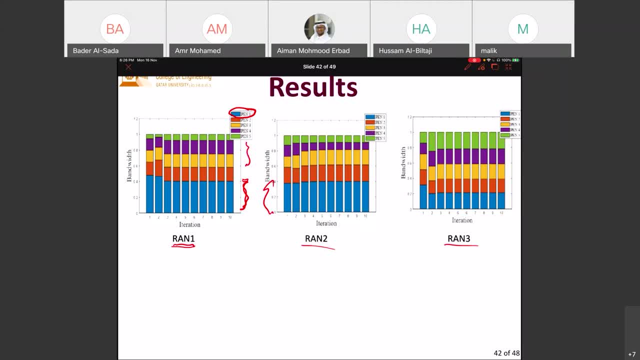 strategy. if you project on the other side with this kind of component that is based on the other side of the data system, then it will arrive at a bed and treatments traffic with it. everything is quite stable again, the data is integrated and solved, uh has the, uh the biggest uh or the largest size of data and in that case it allocates. it allocates big part of this traffic to random. 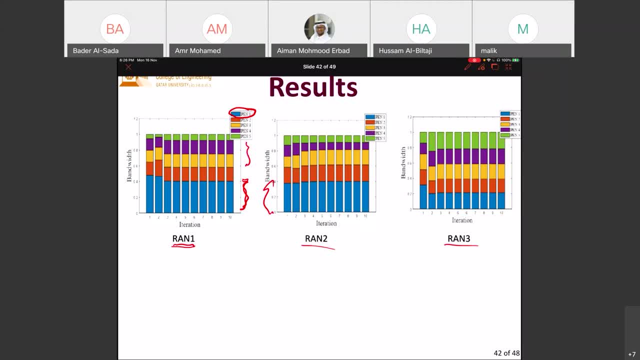 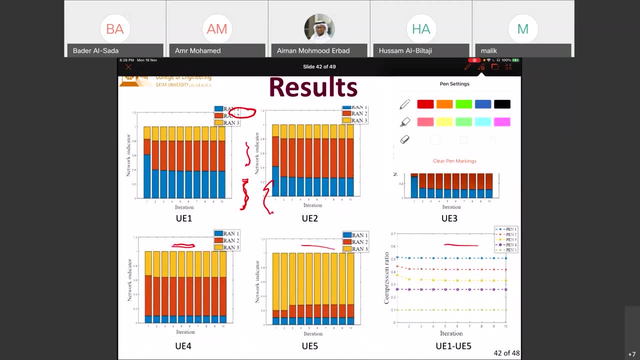 other shares or the other resources from these RANs. Okay, so we also can see the performance in terms of how each user- so we have here in total about five UEs, five user equipments- how the individual users can split their traffic. 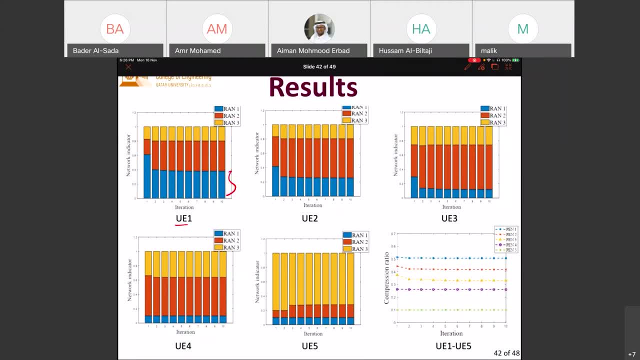 across the different RANs. And again user one with the highest or the largest amount of data, how it splits that across the different RANs. And here we see that for the last curve, here we see that the compression ratio is the highest. 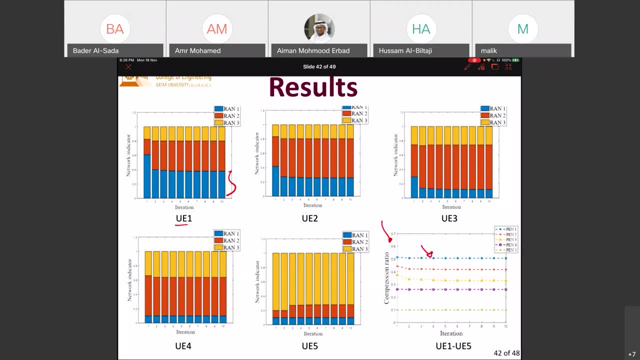 for user one, because user one has the highest or the largest amount of data, So we try to compress the data before delivery in a much higher way compared to the other users. okay, So this work, by the way, did not take into consideration the patient state. 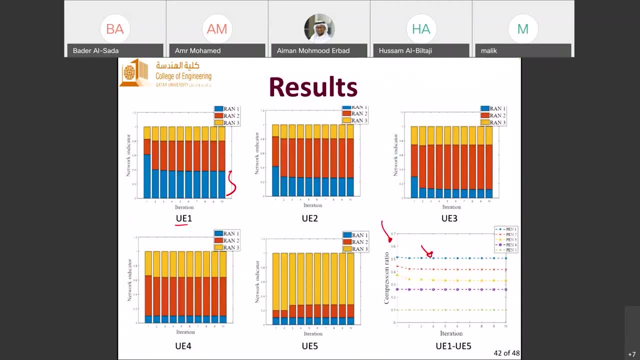 and did not take into consideration the evolution of the bandwidth allocation across a long period of time. In other words, this optimization problem or this solution is greedy in time, is greedy with respect to time. okay, So the other approach here is to try to use 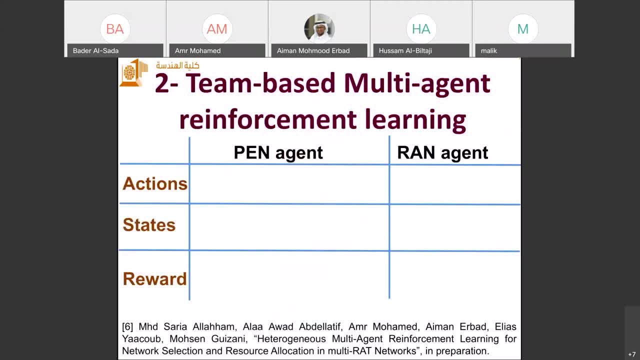 a multi-agent reinforcement learning. So, for multi-agent reinforcement learning, we have two tiers or two types of agents. in that case, We have agents that are running at the user level and we have agents that are running at the network level. Okay, so, which means that this is not only. 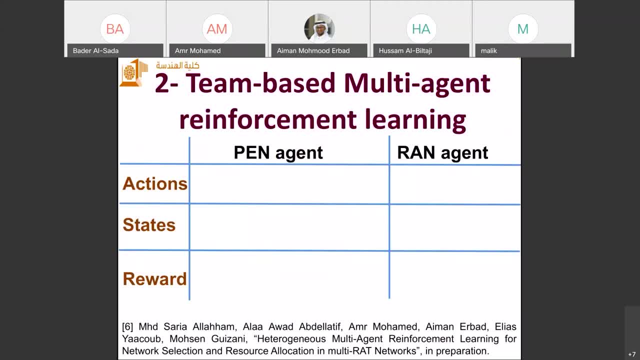 multi-agent reinforcement learning. it's multi-heterogeneous reinforcement learning agents. okay, so each type of agent, we we call it. it's a team based, which means that each type of agent is actually grouped in a team, that they need to cooperate together at a certain level in order to perform the 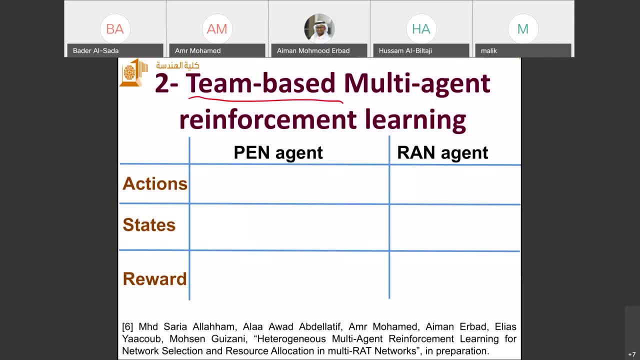 optimization problem. so, for example, at the user level, the action would be: I need to split the traffic using this PIJ and I need to perform certain compression level. at the RAN level, the action would be: what is the share of bandwidth for each user? okay, that is taken from this RAN in terms of states, the states for. 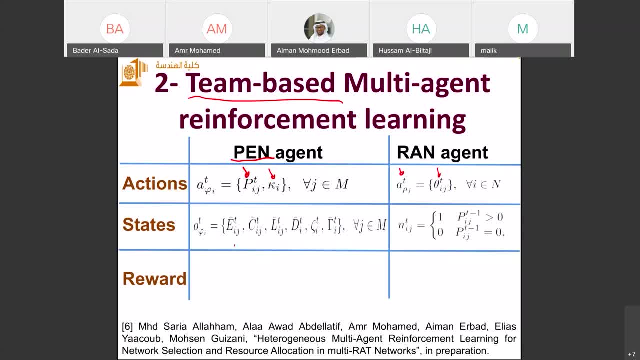 the user agent would take into consideration the energy, that the cost, the monetary cost, the latest latency, the distortion, and the patient state and the residual battery level. so this: these parameters constitute the states at the patient level. at the network level, the state is simply how many of these users are allocated to. 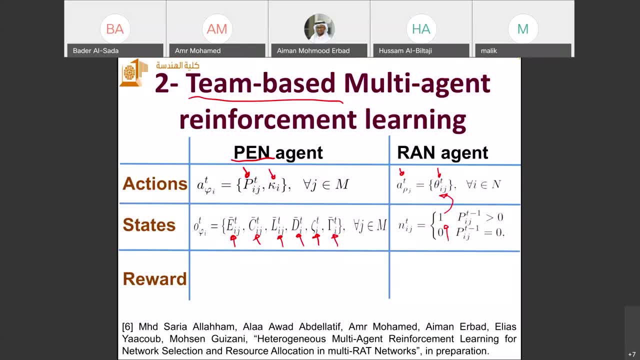 this RAN so that we can perform the bandwidth allocation to this number of users. so based on that, we estimate, or we we try to calculate, these balances based on the patient. so if the patient state is one, this means that the patient, for example, has seizure. if the patient state is one, here we see that we don't actually. 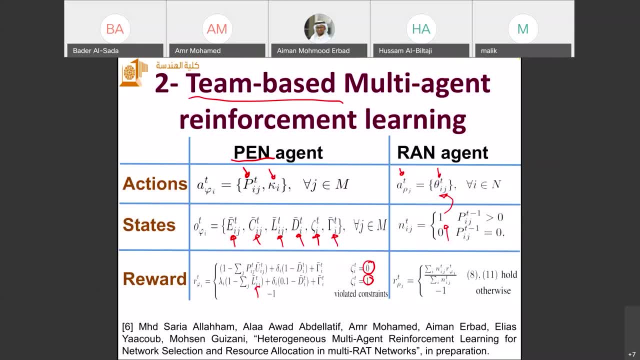 care about energy. we don't care about, uh, anything other than latency. so even if we, if we have to spend more energy, we need to send this data very, very urgently to the cloud: lowest latency possible, even if we have to spend very high amount of energy. okay, 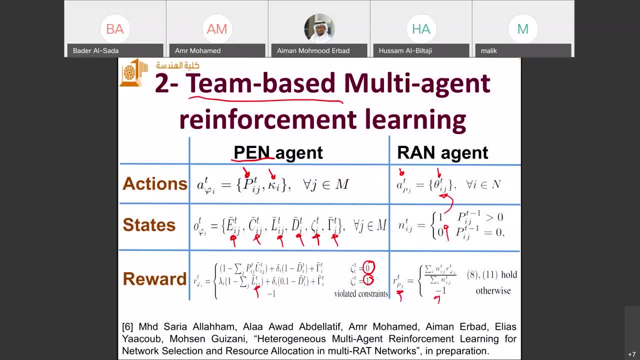 And here the reward is simply based on the allocated rates for each user, based on the bandwidth allocation. what is the average rates from each user, which is proportional to the reward that this RAN would get? So this is the distributed architecture for the multi-agent. 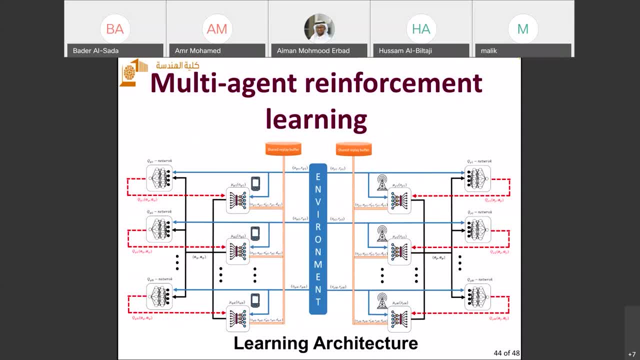 So here we are using a specific class of reinforcement learning called the deterministic DDPG- okay, Distributed deterministic policy gradient. I cannot emphasize enough that this type of problems is really, really complicated because all the problems are related to the DDPG. 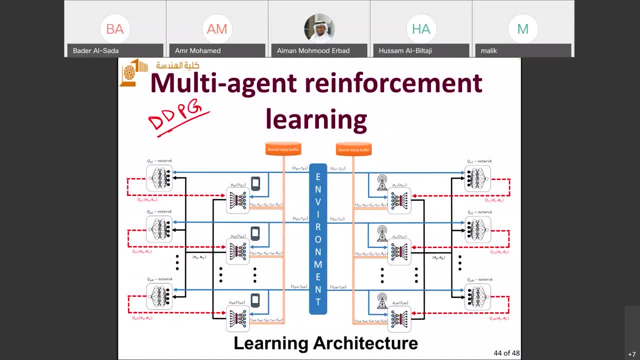 So the four parameters that we are trying to allocate here are continuous in nature, Specifically the bandwidth, the compression level and so on. these are all continuous in nature, So we cannot use the DQN directly. the deep Q network. 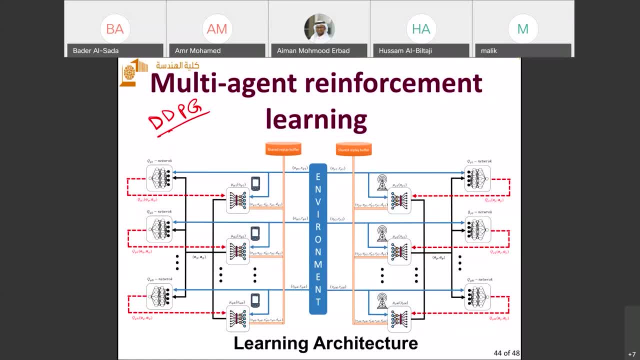 We have to use DDPG or the policy gradient in order to find the best set of actions that we can take at any point of time. Okay, And these are. So the architecture is quite complex, to be honest, So it assumes that you have, for each user, you have to run two machine learning models. 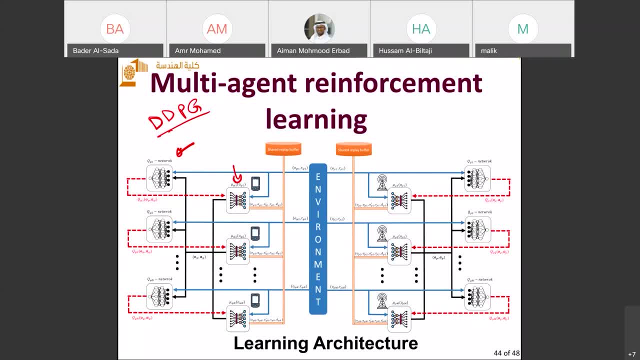 One is called the actor and one is called the critique, If any of you is familiar with the DRL architectures. so we are using an actor- critique model which assumes two machine learning models running at each entity. So we have two machine learning models running at each entity. 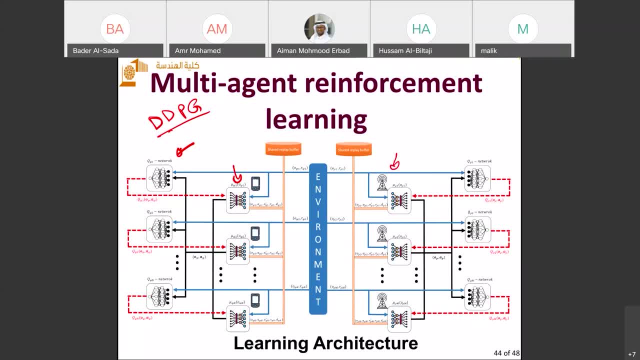 So we have two machine learning models running at each entity. So we have two machine learning models running at the user level and two machine learning models running at the access point or at the RAND level. These networks or these machine learning models, they are interacting with each other using 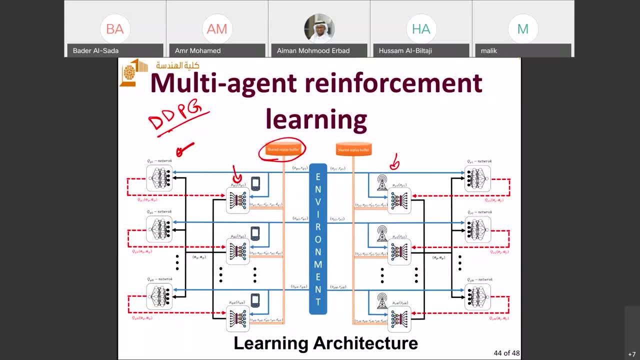 some replay buffers, which represent the amount of cooperation that has to happen between these different agents. Okay, So, by doing this, this is in fact the learning architecture, Okay, Okay, So the bad news is that this learning architecture is very, very complex, and someone might argue: 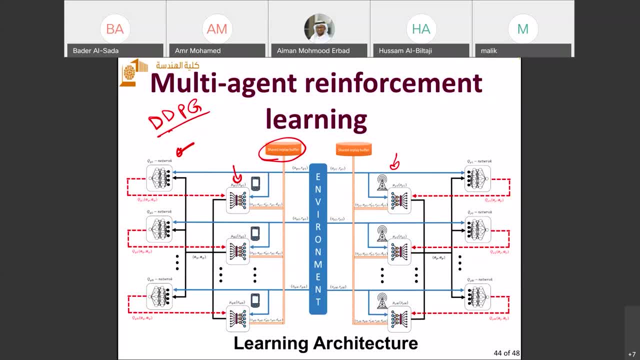 that the amount of complexity here overweighs the value of the multi-agent reinforcement learning solution, because you have to deploy all these machine learning models at the user level and at the network level. The slight good news here is that the execution of the machine learning models is very, very. 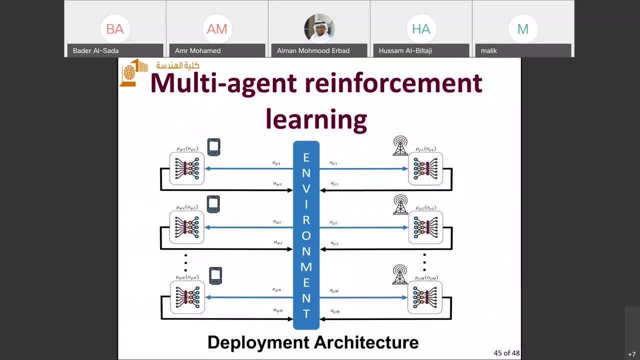 simple. The exploitation or the actual deployed architecture is quite simple. So you have only one machine learning model at each user, Okay, And this is after the learning phase. So after the learning phase, the exploitation phase can be conducted using only one machine. 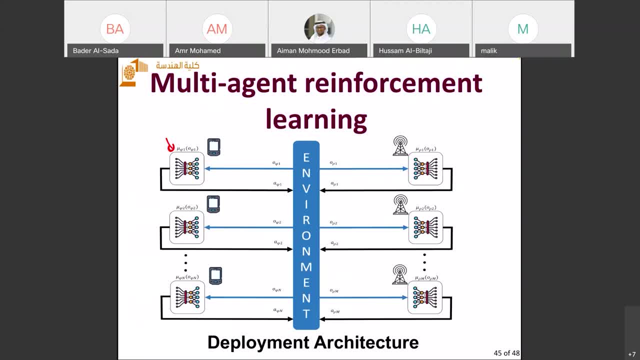 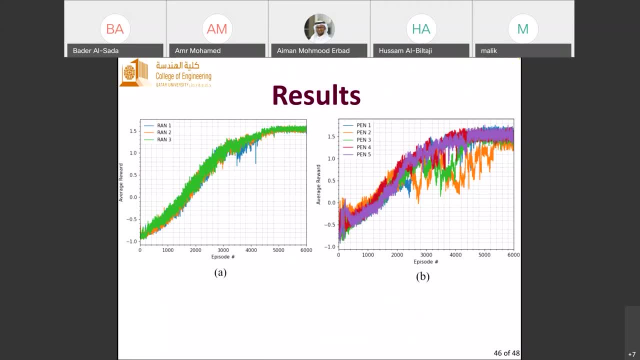 learning model at each entity. Okay, So very quickly again. the first step for each machine learning model is end of the reinforcement. learning is again to analyze the conversions and here, luckily, we were able to achieve conversions at all the entities, so all the different trends. 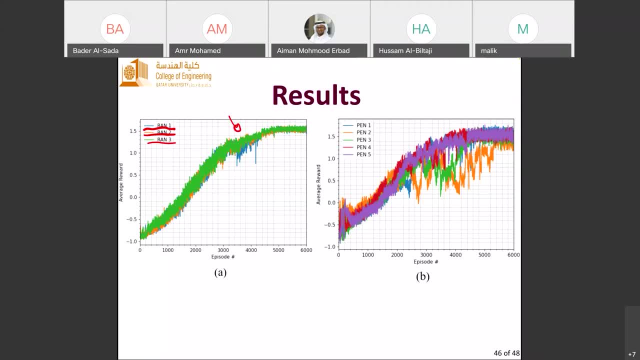 they converge in a distributed manner. so even the learning of the actions and the observations can happen in real time and we can achieve the distributed conversions. and also we can achieve conversions at the user level, at the user agent level. so these are very good news, that conversions 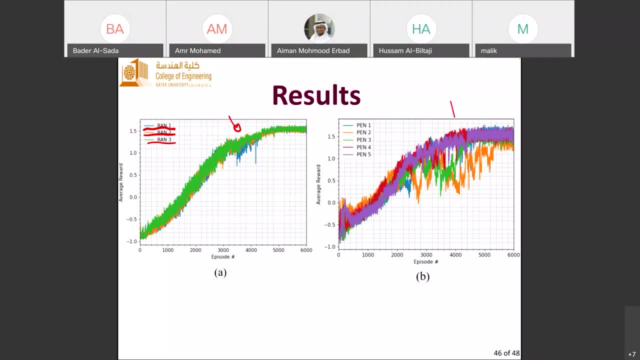 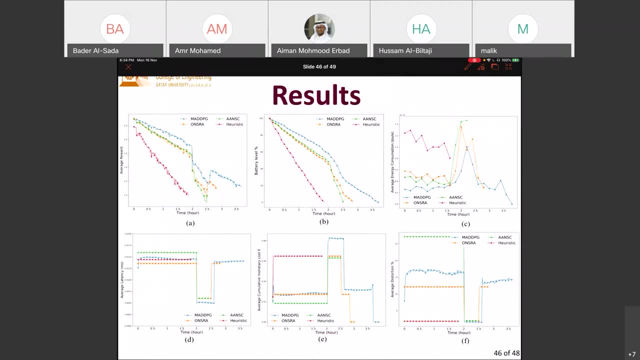 are attained or it's achievable in multi-agent distributed way. and, the last but not least, we can see the results in terms of the overall average reward. here, interestingly speaking, we see a drop in the reward, and the reason here is that here we have an event. 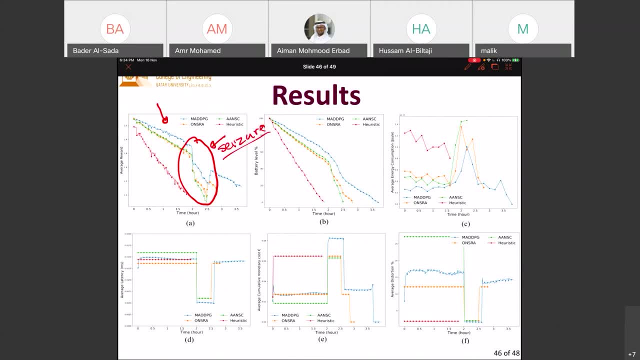 we have a seizure event here for the patient, so a patient at this point of time, probabilistically that happened- that this seizure is. this patient is having a disorder or is having a seizure, in which case we need to deliver the vital signs to the cloud in a very urgent manner. 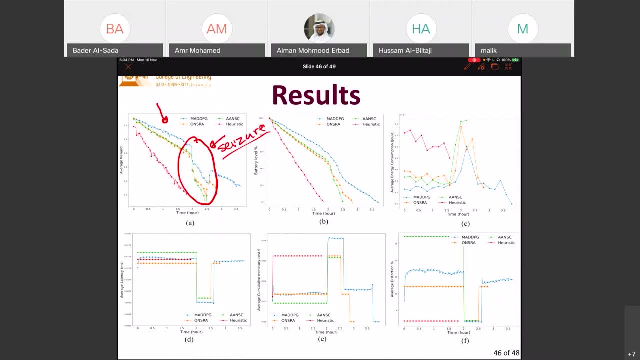 and in that case, we need to sacrifice the energy and we need to sacrifice everything for the, for the sake of latency, okay, and the good news here is that we can see that using the multi-agent ddpg- okay, it outperforms the, the, the optimization solution that we. 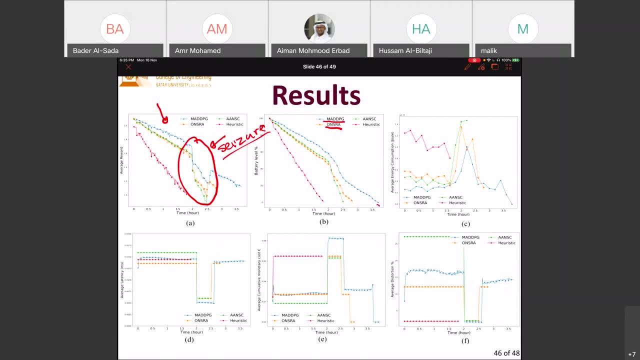 have covered before a significant amount so that the the battery level, this battery level can last at least 50 percent longer compared to the optimization solution, just by using the multi-agent reinforcement learning. okay, even you see the pump. here again, this is based on the the seizure event that happened. 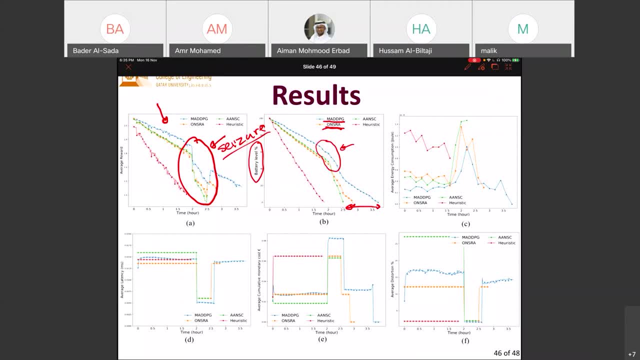 to the to the patient and in that case the energy level or the battery level drops a little bit drastically because of the event, the disorder that happened to the patient. we see, of course, the peak of the, the energy consumption that happened here, again due to the patient state. so the patient state. 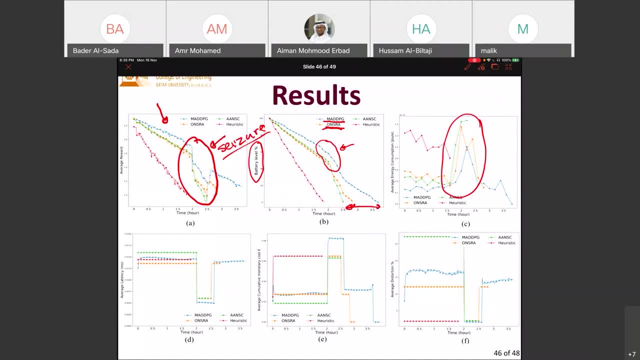 here is taken into consideration while you are doing the uh, the, the action at the user level and at the network level and, of course, the. the event affected all the components of the optimization problem in terms of the, the energy, the average latency, the average uh uh, the, the. 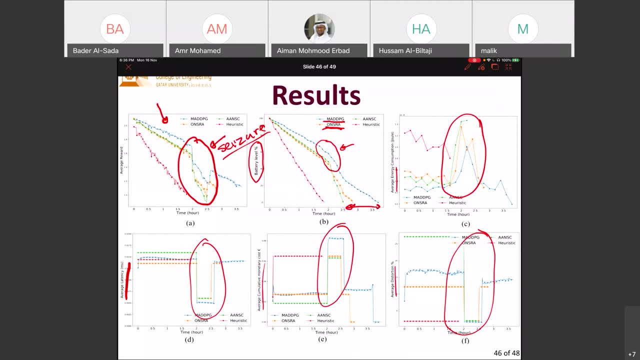 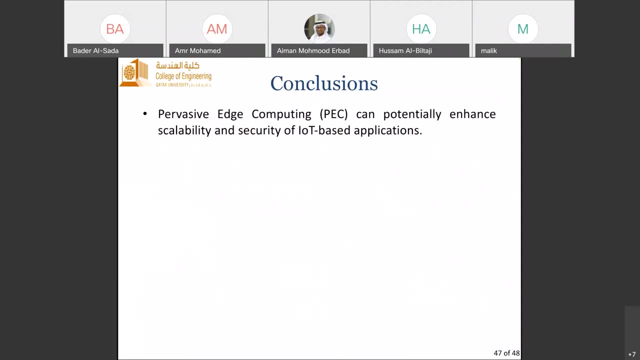 cumulative memory and the distortion level. uh, i'm surprised that you have survived the presentation until now. so so yes, we did. i'm really surprised and i'm glad that you survived the presentation until now. so at the conclusion, pervasive edge computing can potentially enhance the scalability and the security of iot. 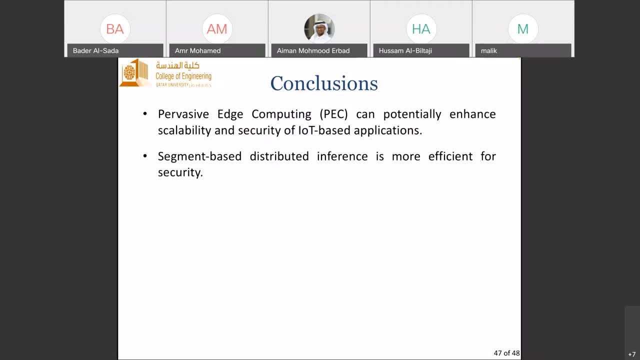 based applications. as we have seen, segment-based distributed inference is more efficient for security and we have seen the black box attack analysis, the, the mobility prediction is essential for distributed inference, particularly for non-homogeneous drone swarm formation, and also the hierarchical federated learning can in fact have a key performance enhancement to address the statistical 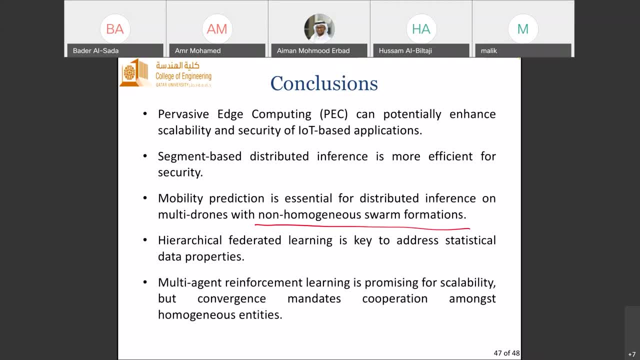 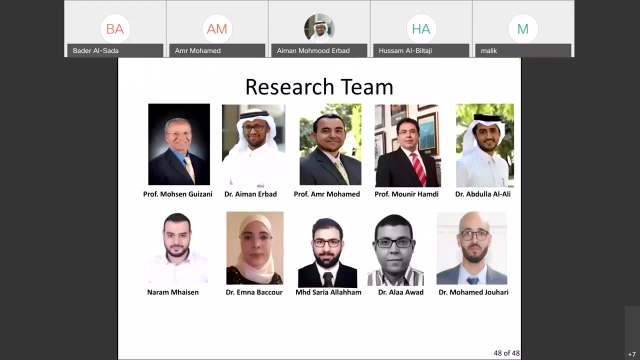 of the data properties and, finally, the multi-agent reinforcement. learning is promising for scalability and for solving very, very complex optimization, a problem in a distributed way, as we have seen. so, finally, i cannot really ignore the- uh, the- efforts of the group members. we have really a plethora of, you know, bright minds of researchers, particularly. 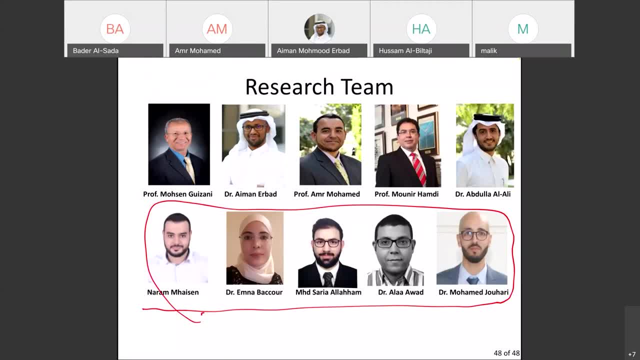 and i would like to commend them for their excellent work. of course, we have more members in our group, but these are the group members that i just summarized their work and, of course, the the supervisors from hbq and from qatar university. okay, thank you very much. 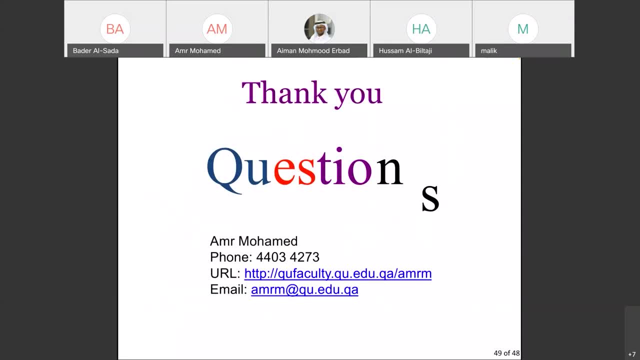 thank you. thank you so much, dr amr, for this very nice uh seminar slash tutorial in in a very complex area and very hot and uh recent area. so i don't know. if people have questions, maybe about the last part, the multi-run, they are still awake. 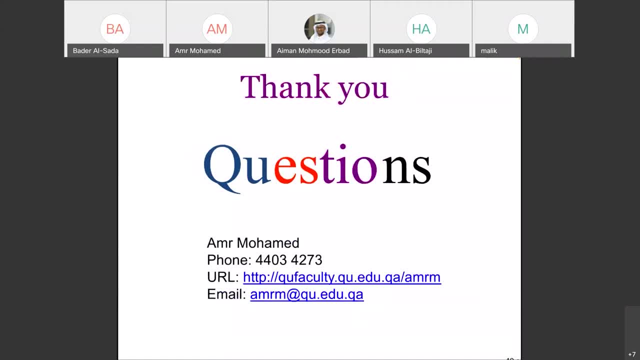 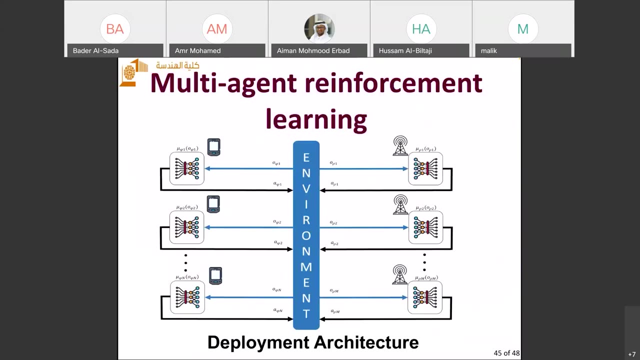 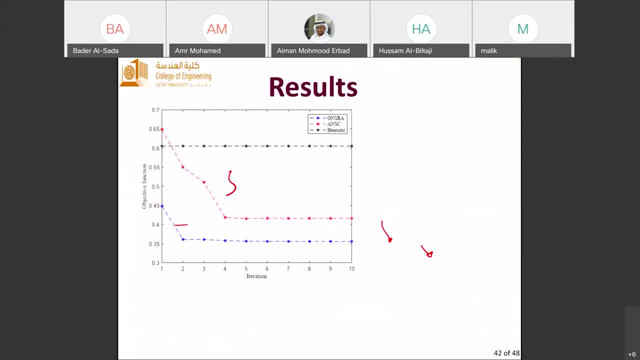 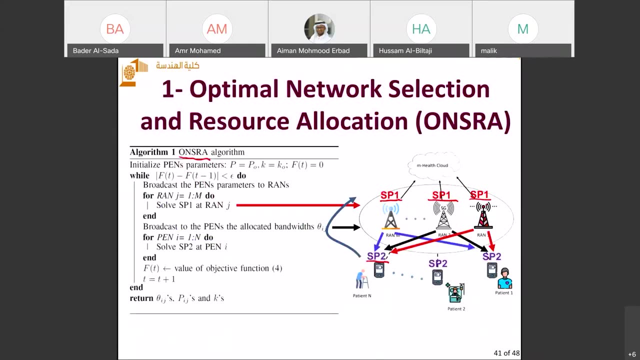 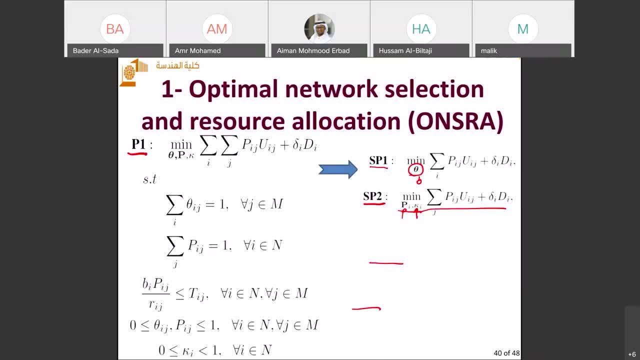 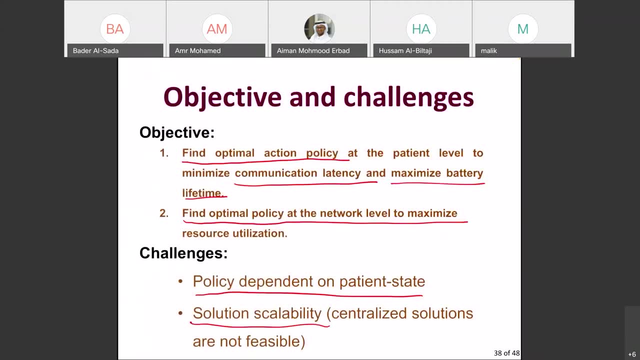 uh, the person currently is having seizure, okay, so for me, what i tried to solve now is that i tried to devise the optimal policy to deliver the piece of information that the person is having seizure in the very efficient way to the cloud, and then the cloud would say: okay, so i want. 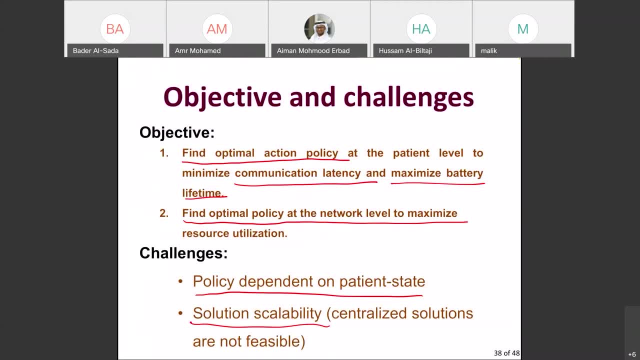 since the patient is having seizure, i want to analyze the vital signs even more, to know like, for example, what is the location of the seizure, what is the state of the of the patient while he's having seizure, and so on and so forth. but the cloud did not have a role in allocating the network resources. 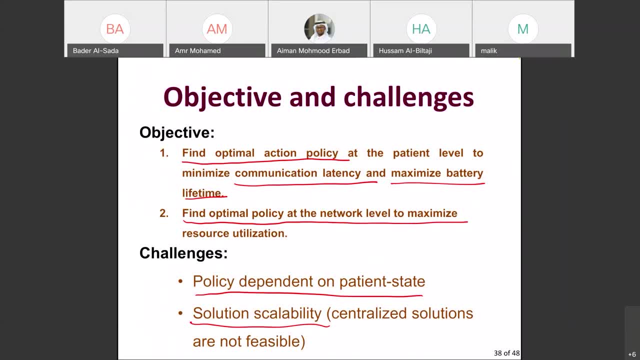 or allocating the different actions at different user levels. not sure if this is uh, yeah, so. so it is not an agent, right? how many agents we have in the mu m m? we have memory, but we also have contact data, so all we need is that we have a robot object to do that. it allows us to know where it is nood. 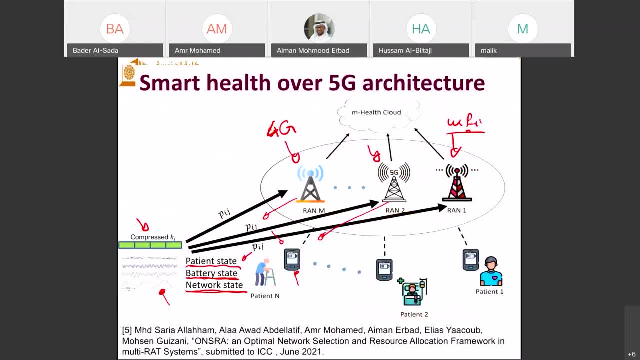 Yeah, I have multiple rats in general, For the sake of the results, we have only three rats and we had about five different patients. The only reason for that is that the actual simulation of the amount of multi-agent distributed reinforcement learning, the simulation itself, takes about three, four days because of the 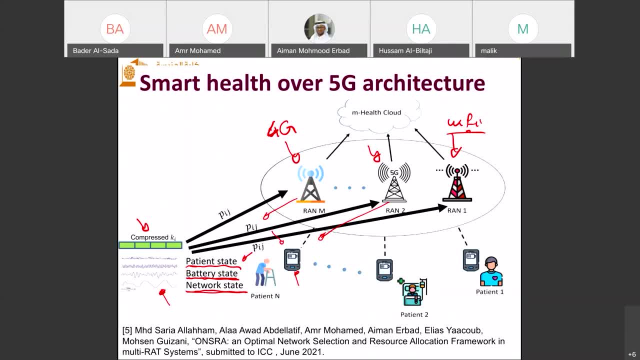 fact that all these agents are deployed in a virtualized environment, of course, So it's quite complex. If you distribute these agents across the different devices, of course, the scalability would be a lot better. So, again, the objective here is to try to. 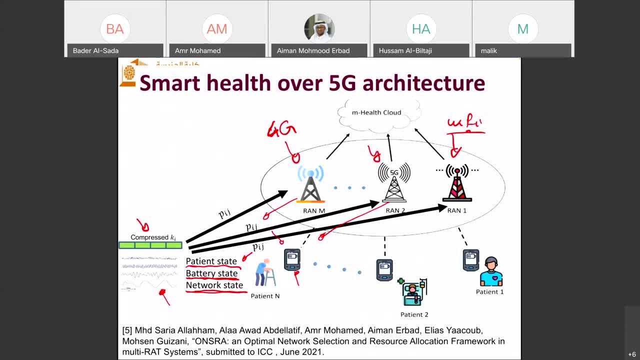 to to achieve the best policy in terms of taking actions at the user level and at the network level to try to optimize the delivery of the vital signs to the cloud. Okay, Okay, But then the assumption here is that the cloud has more analysis that it needs to do, which? 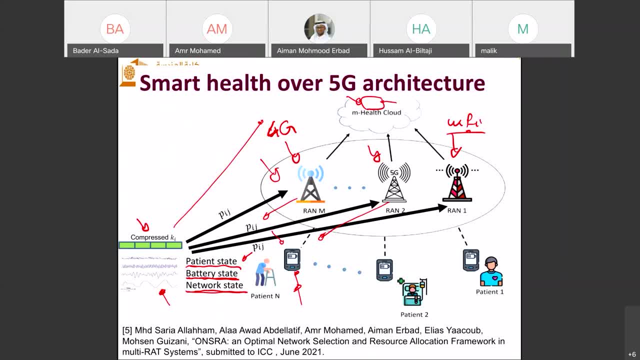 is outside of the scope of this. That's why there is no machine learning model in the cloud, in that case, Fadl. Yes, actually. One more comment please, if you go to the results part: the convergence of the models. 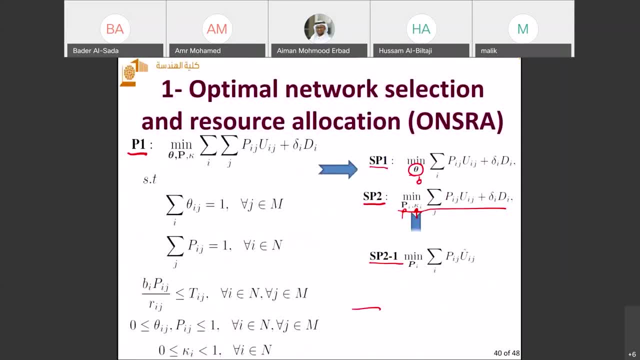 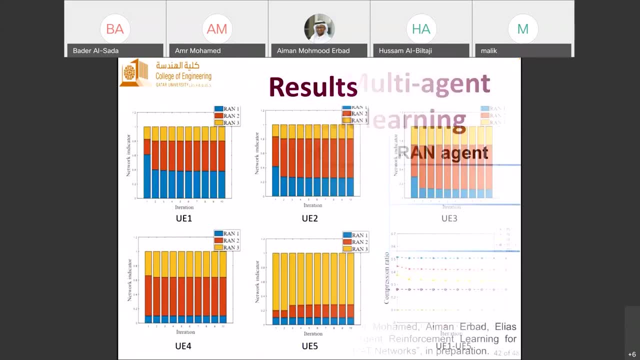 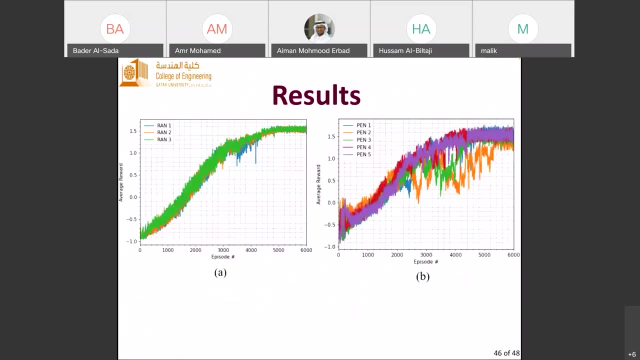 Yes, Sorry, The conversions of Yeah, Yes, Yes, actually, figure B: actually, If you see, I recommend that you extend this, You can extend the number of episodes here. Yes, yes, you're perfectly right. Yes, by the way, I had to say I had to say something. 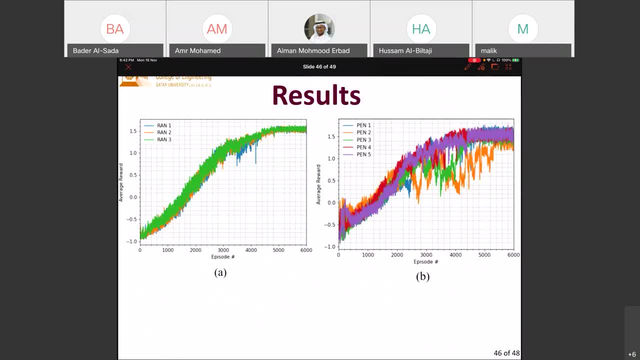 This is still a work in progress, by the way, this, particularly this multi-agent. That's why I left it at the very very last part of the presentation. This is still a work in progress and we're still trying to optimize, actually to try. 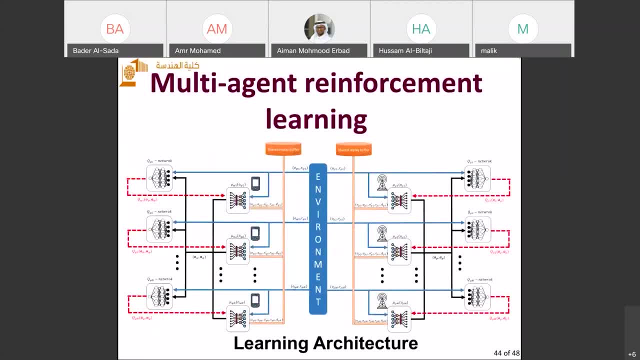 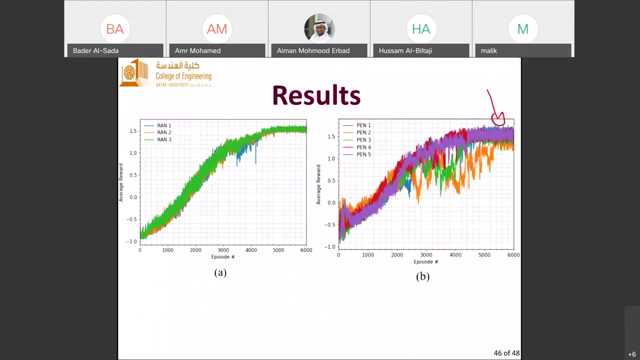 to redesign the learning architecture and the deployment architecture In a more efficient way. so still a work in progress, to be honest, but you are perfectly right. So we need to extend the learning part here in order to achieve more consistent conversions. 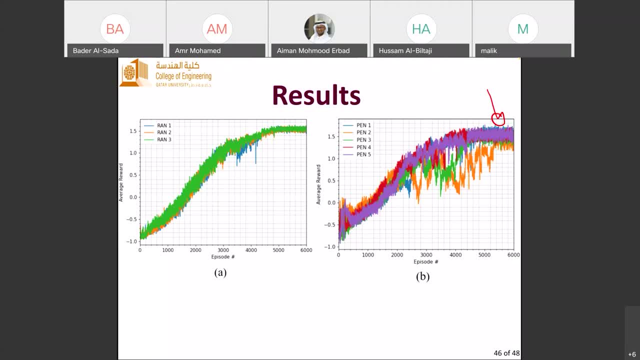 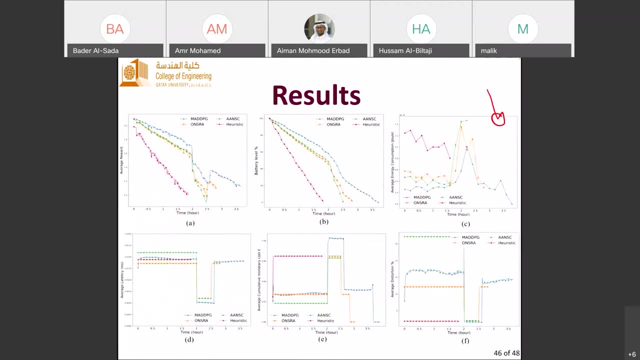 You're right, You're perfectly right. Yes, Actually, my final question here: go to the last results, please, the one just after this one. Okay, Here the ONSRA and the PG. The ONSRA, Right. 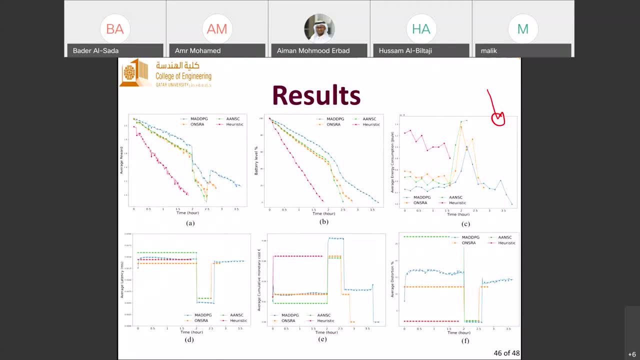 What do you mean? Yes, the theoretical optimization. yes, but yeah, I have to say something here. As we said before, this theoretical optimization is actually greedy with respect to time, which means that it actually finds the optimal solution at an instance of time. 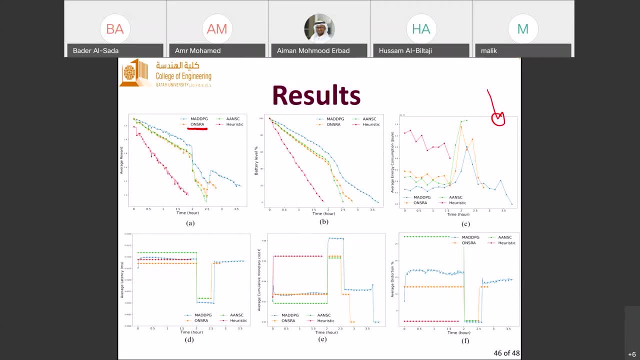 It does not try to find an optimal policy over a long period of time. You see the difference? Yes, So can we. It tries to find the optimal action at this point of time, without considering neither history nor future of how the parameters of the system would change. 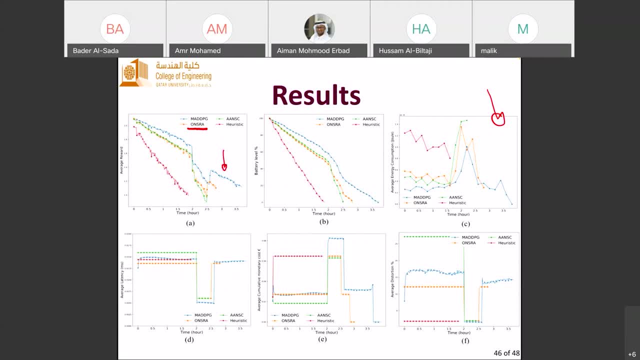 Like, for example, it doesn't take into consideration the battery level. So if the mobile device has a very low battery level, okay, The battery level, Okay, Okay, Okay. So the reinforcement learning can expect that, can predict that, because of the fact. 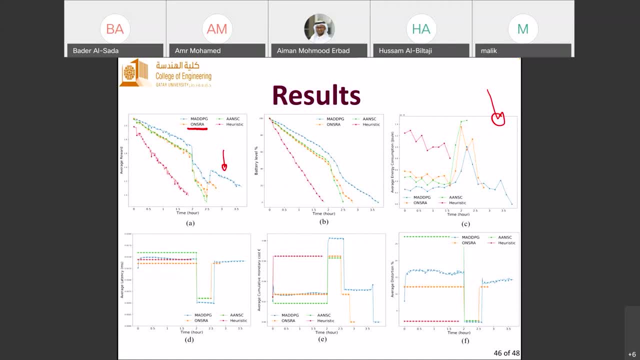 that if I take this action, the battery level would drop significantly. I have to spend more time on data compression in order to optimize the battery level at a long time horizon. The ONSRA, The ONSRA, The ONSRA. 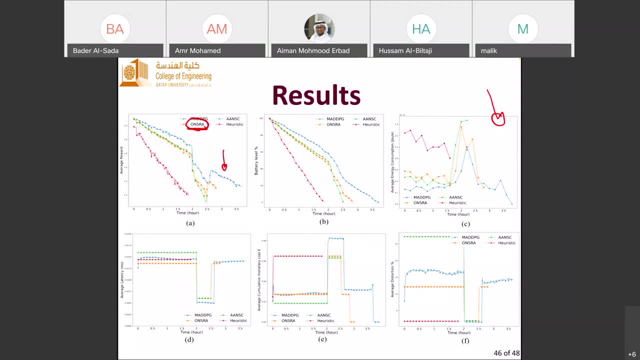 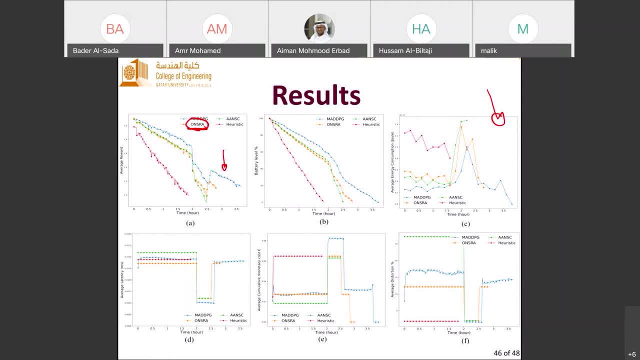 considering neither history nor future. That's the main difference And that's why here. you see that here, at this point, we can see a significant enhancement in terms of the lifetime: the lifetime almost by 30 percent or 40 percent and more like, if you. if we consider the performance. 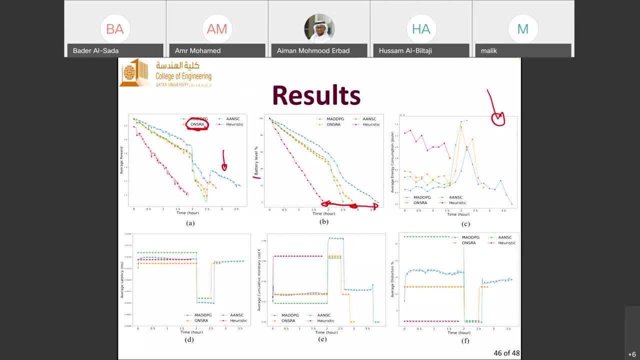 difference with respect to the heuristic: it's almost 100 percent, so i can make the battery life for at least double the amount of time. okay, using the multi-agent reinforcement learning compared to the simple solution, the simple heuristic solution. yeah, so one last technical question regarding you know. 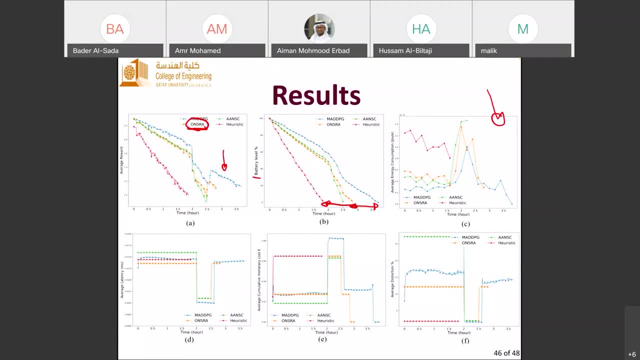 calculations. consider the interference, or i guess we don't have an interference in this case, since we have multiple rats, different rats, right? yes, you are perfectly right. we did not perform interference management in this particular problem. it's physical layer guys. so i'm glad he's not here, or he would not. he would be more. 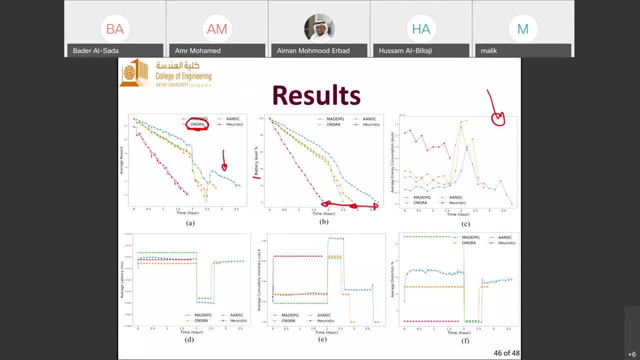 yeah, maybe more rigorous than his student in saying: okay, how can you not in this network? yeah, how come you and you go across the interference manager? i know, yeah, there is no mimo here and yeah, so, so, yeah, so. so we did not consider physical layer issues. uh, 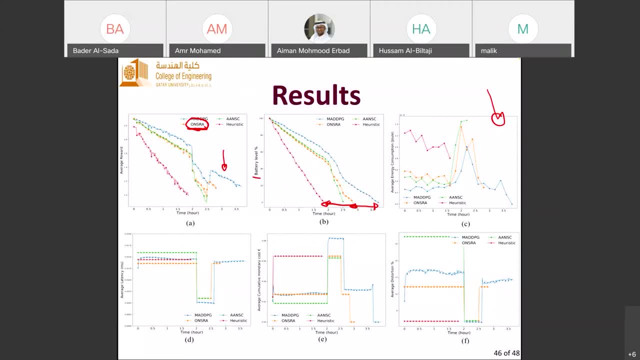 who is asking? i, i need to know your name, malik. malik, a lot of questions from malik and abdul latif, and these are actually their areas of work. so that's that's. that's very, very interesting, uh, questions. uh, yeah, mashallah you are. you are asking very good questions, malik. yes, really, uh. 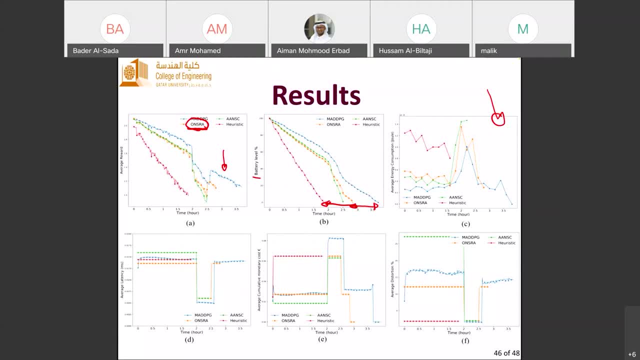 we did not address interference management in this part and we're considering that the communication that happens between the users and the rats has no effect on the interference to other users. okay, thank you so much. thank you, sorry for the question. thank you for no, actually excellent question really we enjoy.